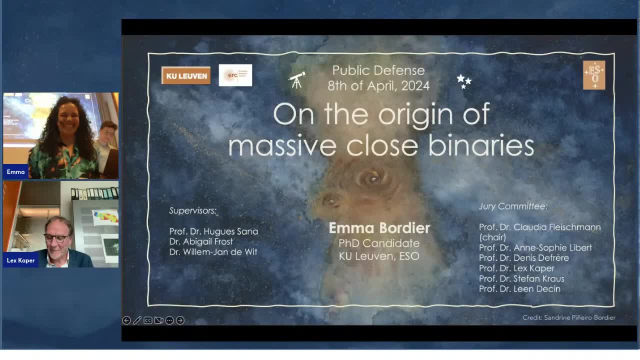 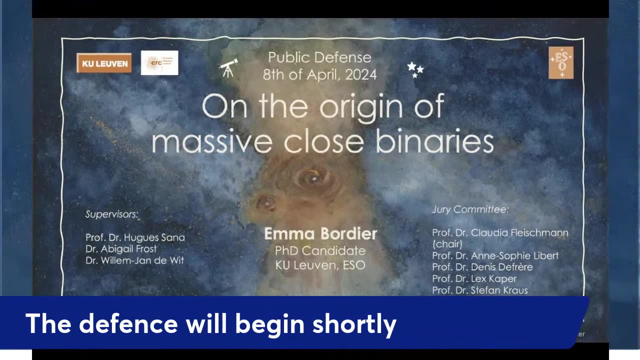 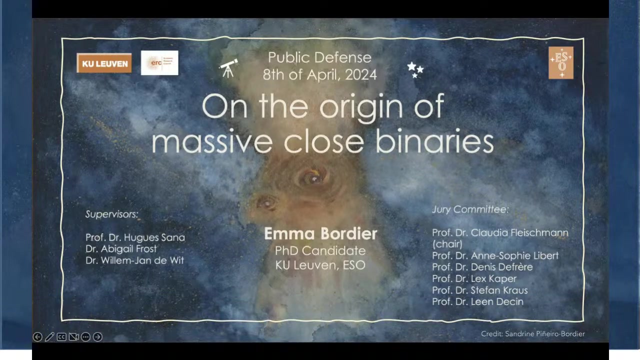 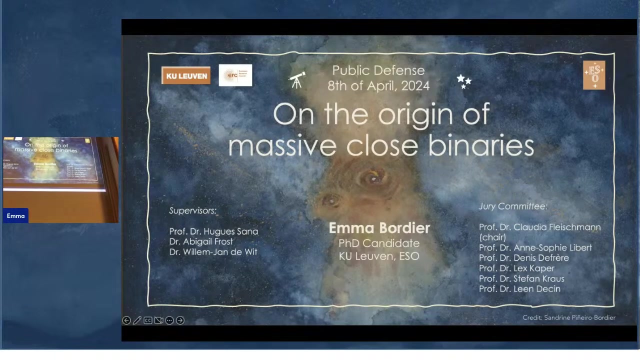 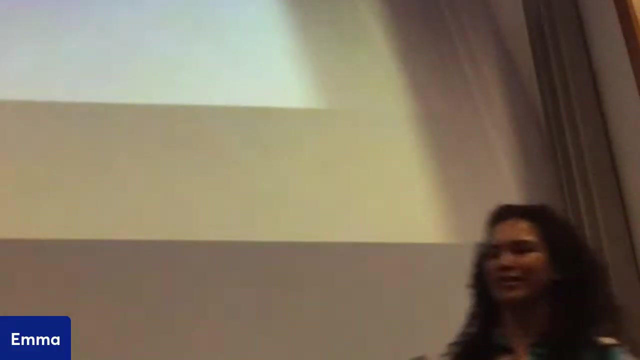 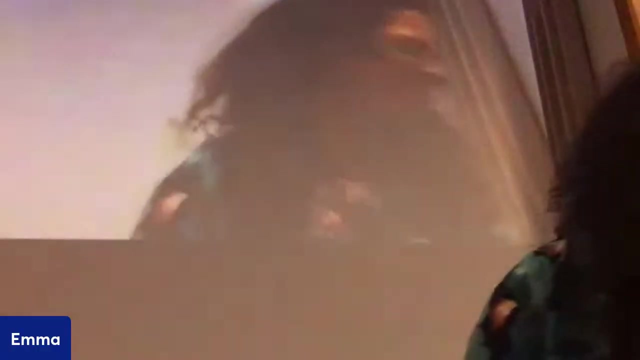 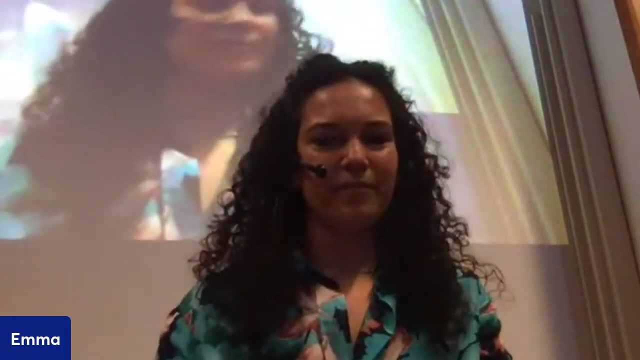 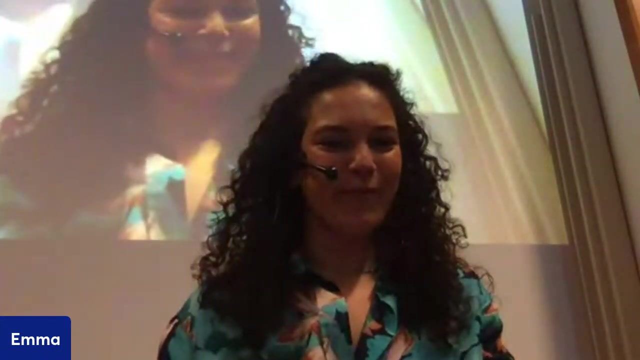 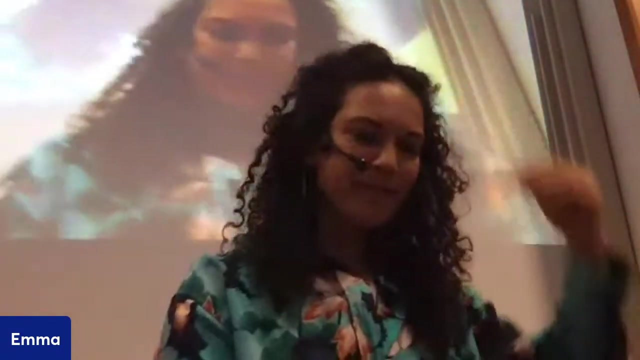 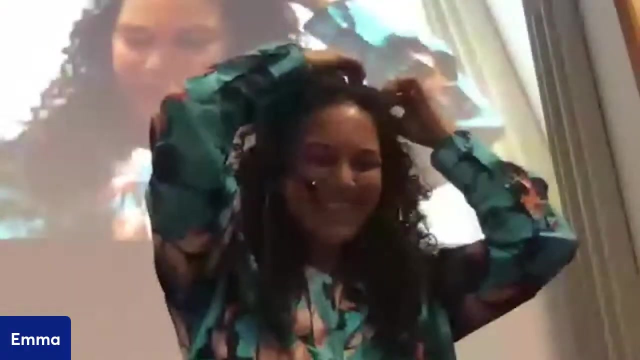 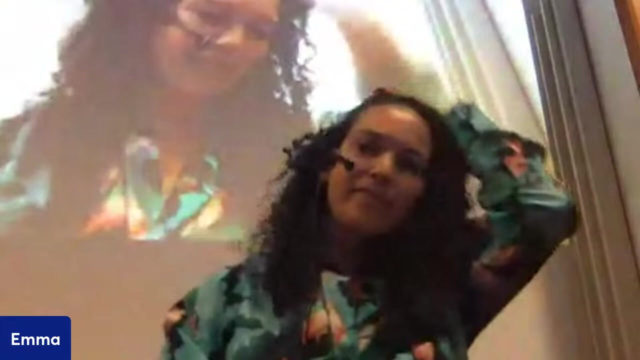 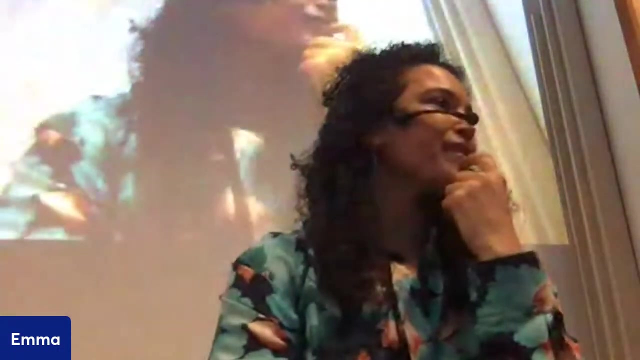 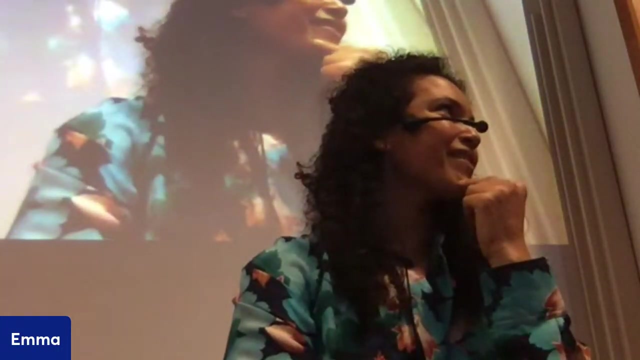 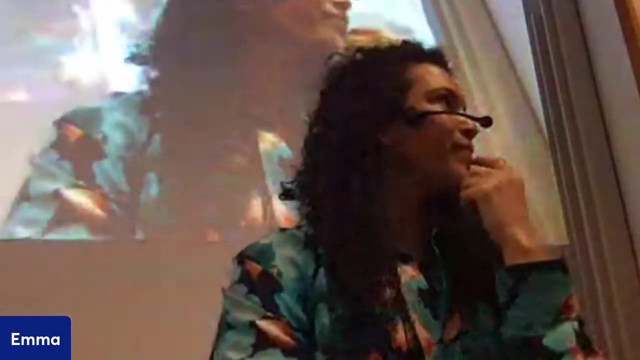 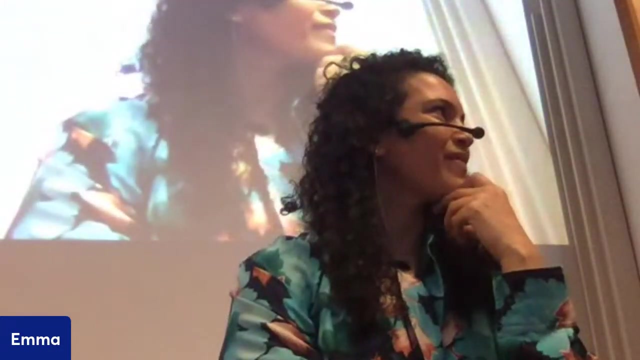 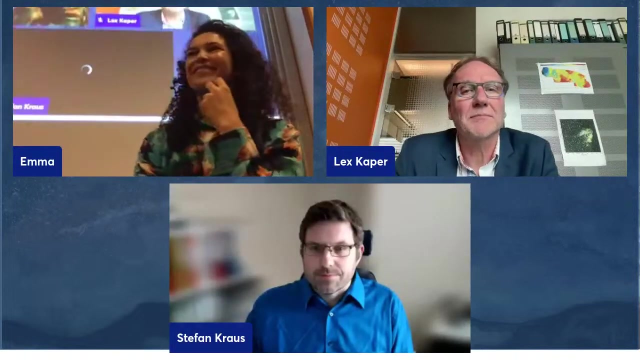 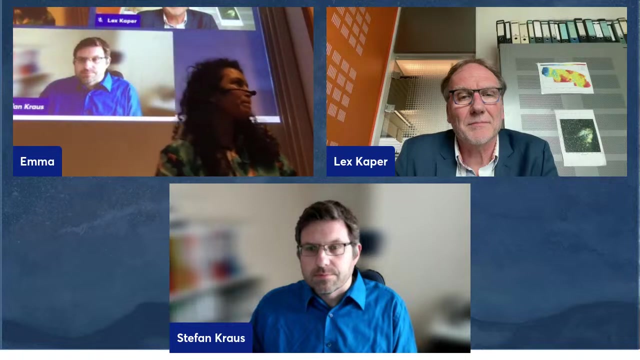 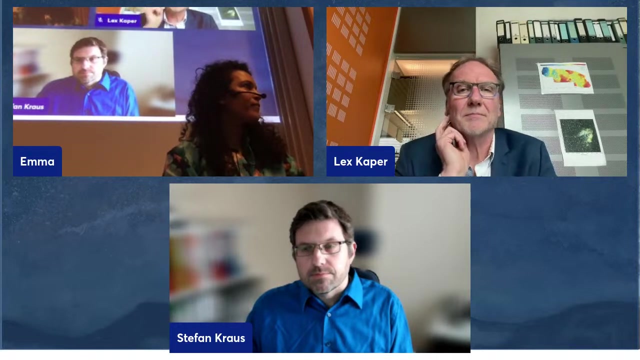 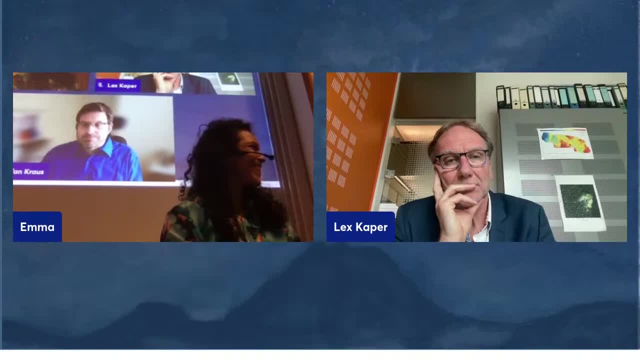 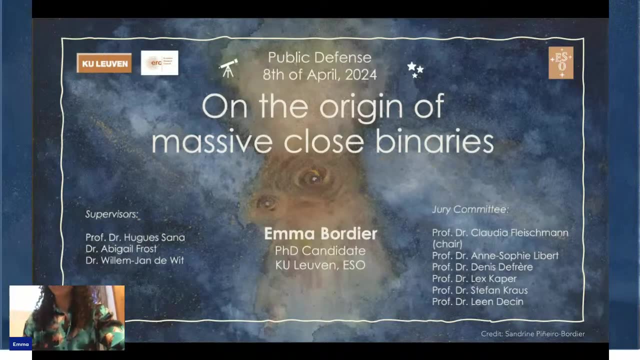 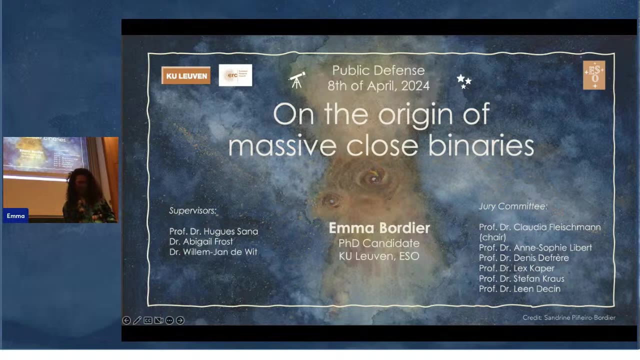 I'm chairing the session Now. the floor is yours. Good afternoon, everyone, and thanks for being here, either in this auditorium or online. Today I will be presenting a bit of the work that I've been doing the past four years that. 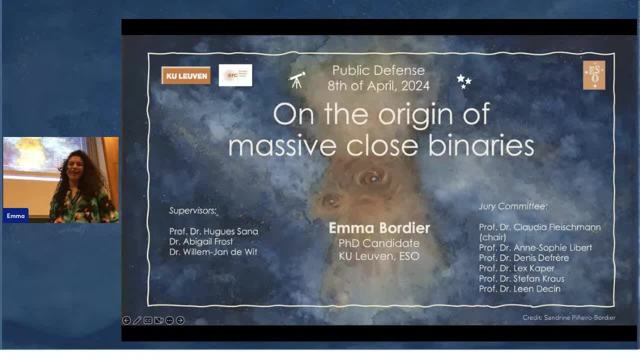 involved observations at higher para-resolution with the aim to provide my piece of the puzzle in the big unknown, that is, theory of massive close binaries. Thank you, Thank you, Thank you. Now, probably many of you don't understand completely that title, or maybe you understand. 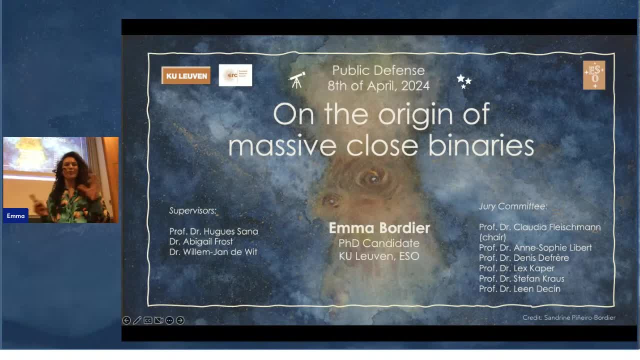 part of the words independently, but when they are put together then it becomes a mess. So I will start with explaining all the terms of the title and then I will follow by the main objectives of the thesis and present the main results of my work as well. 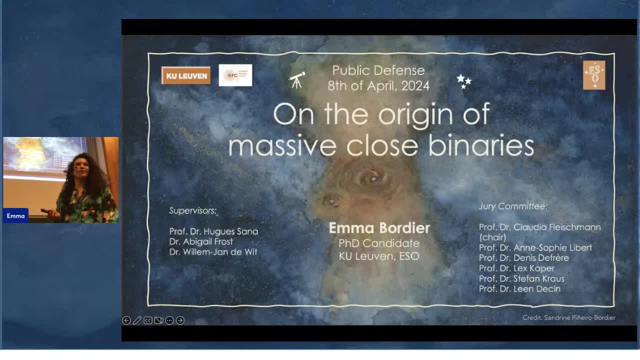 I really hope that at the end of this presentation you can leave either this auditorium or close it up on your laptop. They have to answer as many questions as possible. You will see that at the end of the conversation you can leave them to answer the question, if 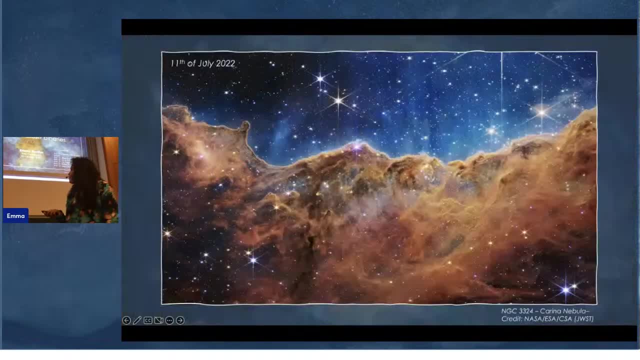 they manage to do so, And if you leave them to answer, you can leave them to ask the question, And if you leave them to answer, you can leave them to ask the question, And if you leave them to answer, you can leave them to ask the question. 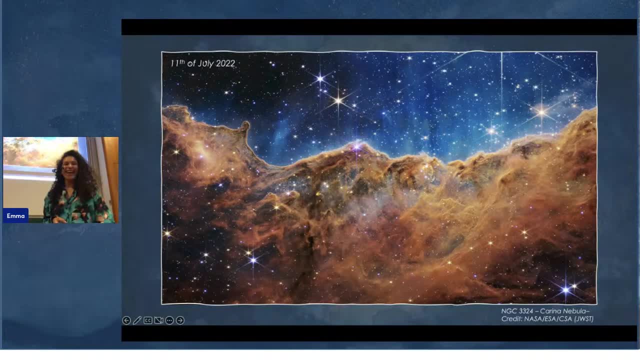 And if you do leave them to answer, You will have to leave them to answer again. I think the second topic is very important. You'll be able to bring back the previous topic. that is the talk of the day, So let's start with a fewlining. So first I'd like to bring you back to this related topic of July 2020.. I remember I was at ESO with other students and fellows in Chile And we had, for the very first time, the James Webb Space Telescope release. 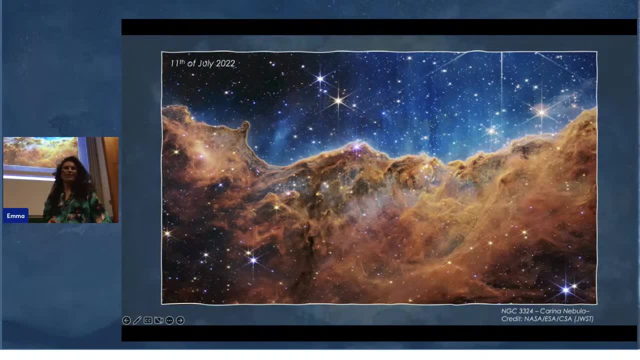 I remember I was at ESO with other students and fellows in Chile and we had, for the very first time, the GEMS Webb Space Telescope released. so NASA, ESA and also the CSA, which is the Canadian Space Agency. they made public five full-coloured scientific images and for the 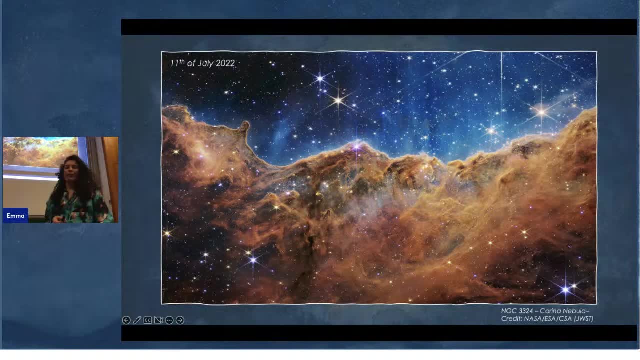 very first time by G1USD, and we were waiting for that time. I remember I had just started my academic journey, so these were the very first images we were already looking for. So this is a stellar nursery. this is the Carina Nebula and you can see it has a bit. 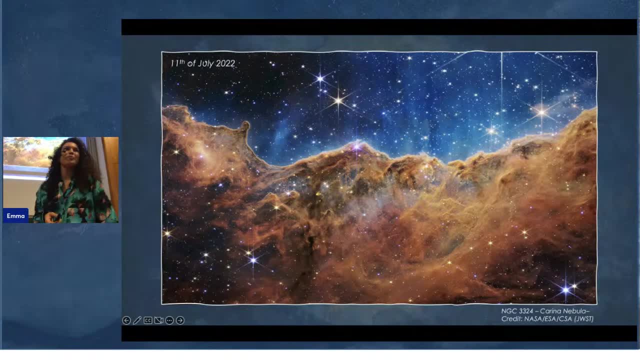 of a shape of a craggy mountain on a night evening- that's probably why I like it so much- And it represents the edge of a riverbank. So this is the Carina Nebula. This is the Carina Nebula. 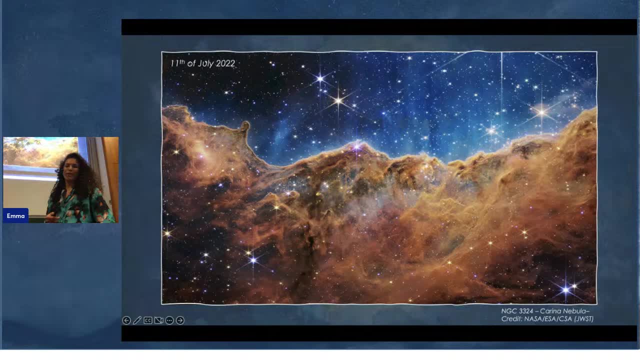 This is the Carina Nebula, And this is the Carina Nebula, And this is where everything begins. It is in stellar nurseries just like this one that our son was born 4.6 billion years ago and consequently, our home. 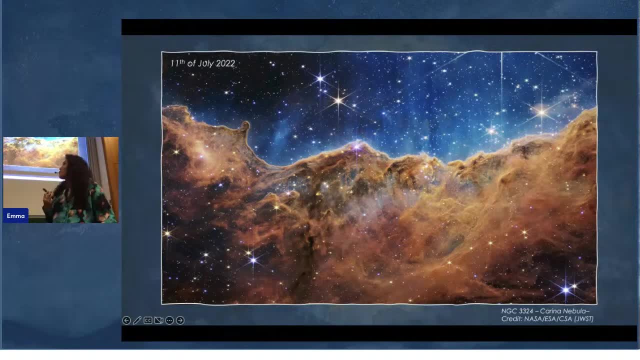 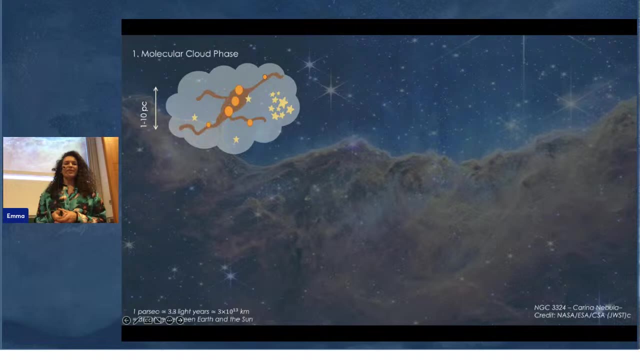 We were born out of dust and gas. yes, just that. But you will wonder, how do we turn these huge amounts of gas and dust into stars? So this reaches, uh, where the density is a bit higher than the internal world. um starts from. 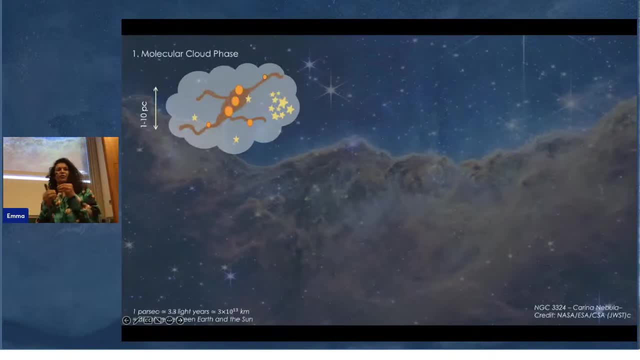 sorry- from an accumulation, small accumulations- of gas and dust which collapses due to gravity. so the dense and cold- is very cold in the cloud that are made of mix of atoms, molecules and dust under their own gravity, thanks truly to a personal source of energy such as a little. 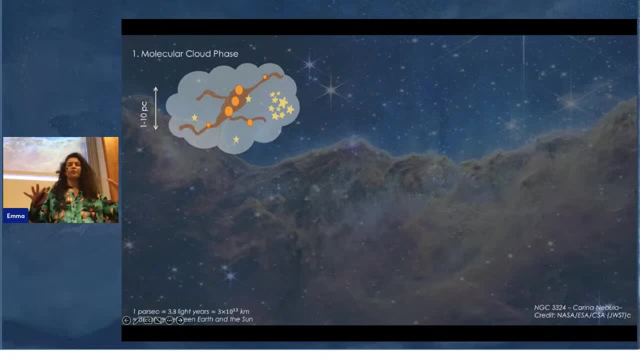 kick from the supernova or bucket, more clouds colliding also um with each other, and other cloud gets smaller, it breaks into massive filaments and spherical pockets that you can see here. so this is like a filament and some pockets um that we call clumps or hubs, and these hubs, uh, the host dense pores of different masses and these are the sites for. 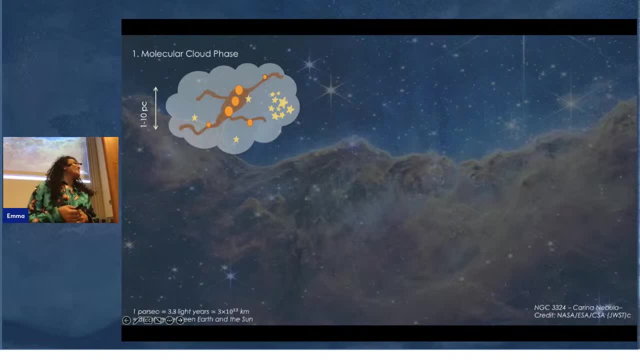 star formation. yeah, you can go good. so in the traditional theory of star formation, the mass that is present in this world, um defines the mass of the, the newly formed star, and in this dense pocket, and it created one or more stars. if you create more stars, then we can call it a cluster um the newly formed protostar. 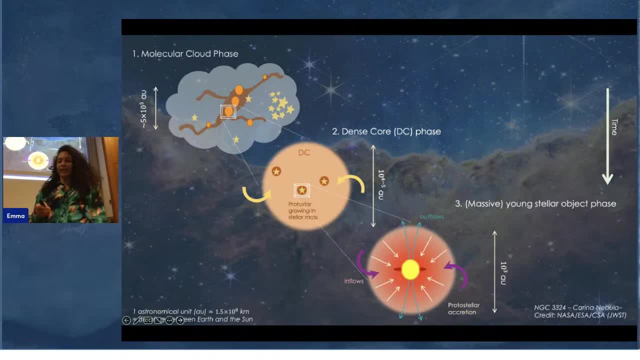 grows in mass through accretion at different scales. so it can grow from accretion, from the envelope by like gravitational driven um streams that people influence. but it can also grow from the accretion disk. so when you have, like all the material that is collapsing. 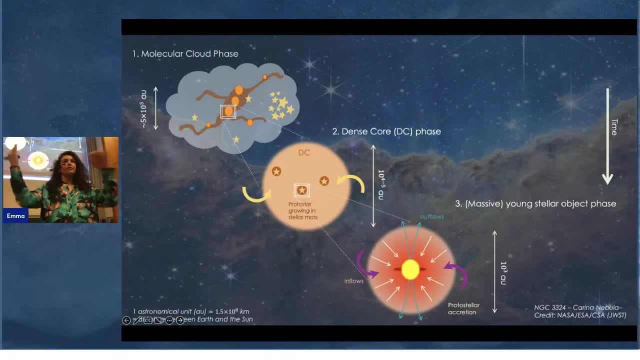 from the envelope. you have to imagine that this material, like, collapses but also retains very fast and to conserve the envelope. and then all of these patterns and you have a creation of an impression which is the around the forming star. and from this aggression disk there will be like 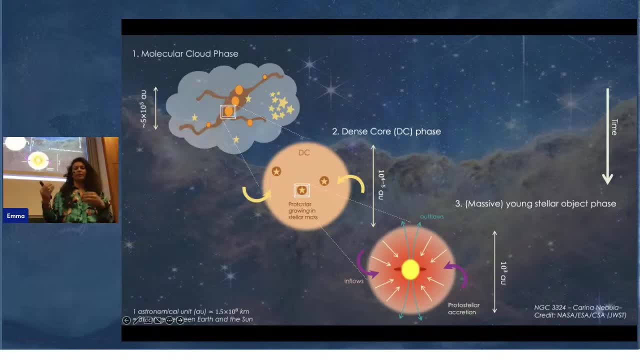 streams like spiral light chains that will um accrete all the matter, the material on the star, to, so that the star can build within us Over time. these nascent stars will use up much of the gas and dust from the original molecular cloud, though they may also blast some of it away in the form of jets or outflows during these very rare processes of accretion. 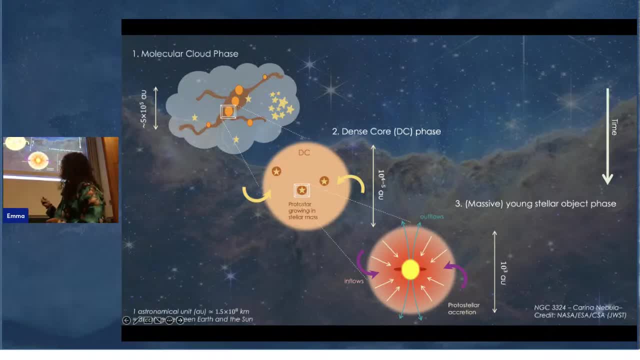 The disk around these stars is the place also where you can form planets that will become like the solar system in the case of glass stars, But in the case of massive stars it's the site where you can eventually form other stellar planets And then, when the star or central core here becomes hot enough, then nuclear reactions will be triggered at the center of the star and a new star is born. So the formation process is over And the star will start its very long journey until death. And at that time the radiation is so strong that the star will blow away all the remaining birth material. 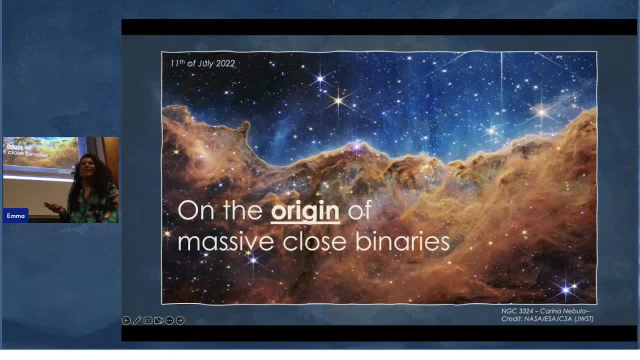 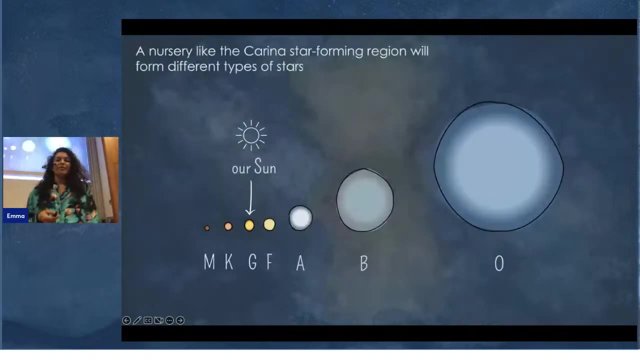 So now you already understand one of the terms, that is, the origin. So by origin I refer to the formation, actually, of stars. But what kind of stars do we actually form? OK, so depending on the size of the molecular cloud, we may form a few to a few thousand hundreds of thousands of stars. 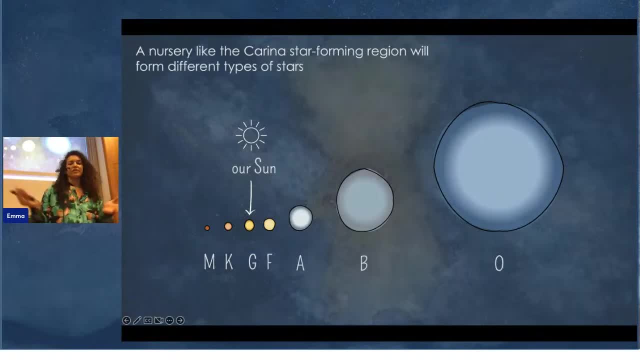 And there are like a plethora of different kind of stars that we identify with a spectral type, that are like the letters that you can see here at the bottom. It's just a bit like you. when you were born. You were assigned a name, a weight, height. 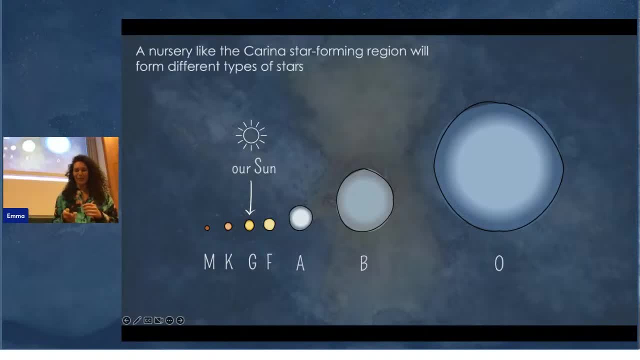 And this is how we know who you are And that you are unique. So it's a bit the same for the stars, And they differ by different things. First, there are several parameters, such as the mass, the temperature, the density. 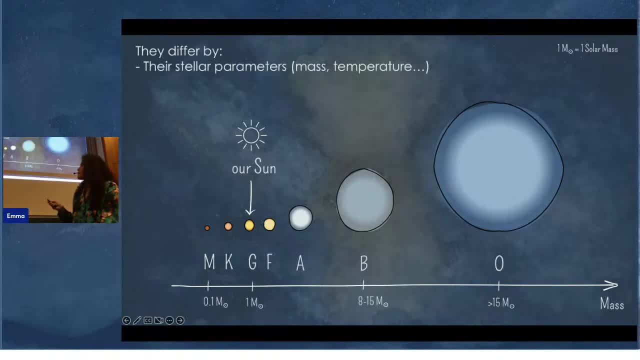 And in astronomy we usually take the sun as a reference, always. So. if we consider that the sun has a mass of one solar mass, then it will form stars as light as 0.1, even 0.01 solar mass, up to dozens or even hundreds of solar mass. 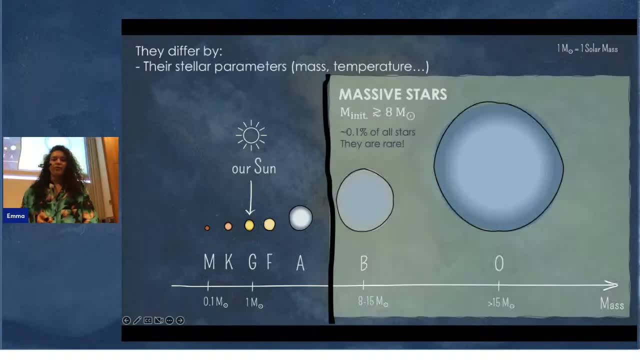 And so we have stars that mass usually in three different categories: low mass, intermediate and high mass. And in the remainder of this presentation and in the thesis and I think probably all the massive star community we agree that we call the massive star any star with a solar mass greater than eight. 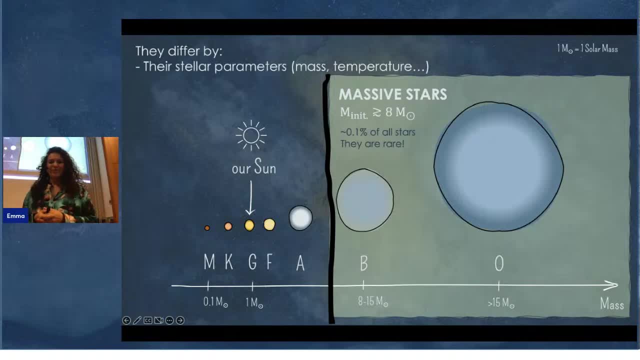 when it's born. All these stars fall into this category, And all the rest. for this presentation, I will call it low mass. We have this whole spectrum of masses, but given the limited amount of available material in the initial class, we will form way more low mass stars than massive stars. 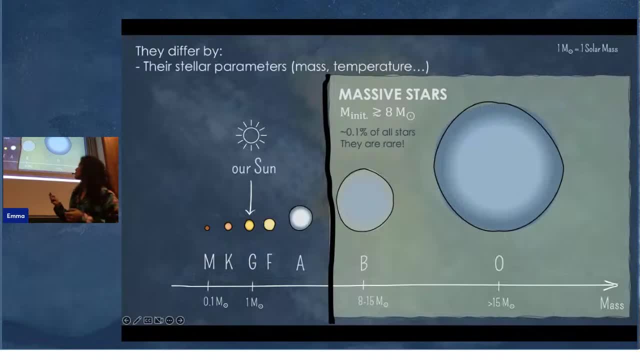 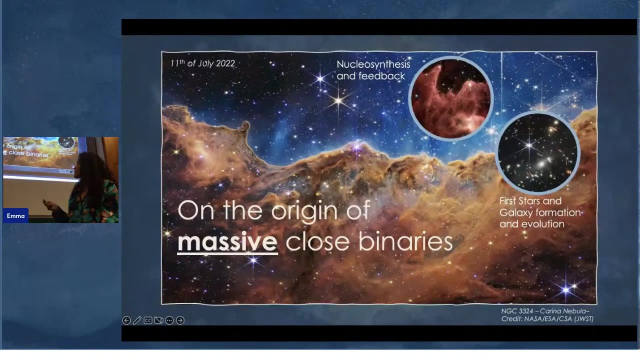 such that in the end, when we have a population of stars, only 0.1% of them will be of high mass, So they are really rare. So here you already understand a second star, if it wants to be a star which is massive. 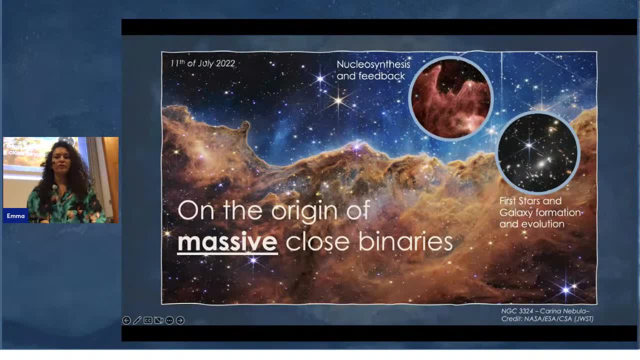 So massive stars are really important when we study the universe because they are powerful machines And their study is relevant in a lot of different fields in astronomy. First, because the very, very first stars that were born in the universe were of very high mass. 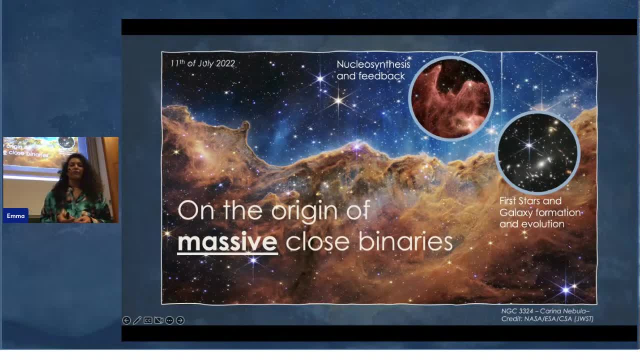 And they were known to have created very first galaxies and to have contributed to the re-alienization of the universe, which means when the universe became visible. Their study is also of great interest because they end their life in supernova. I will come back to this later. 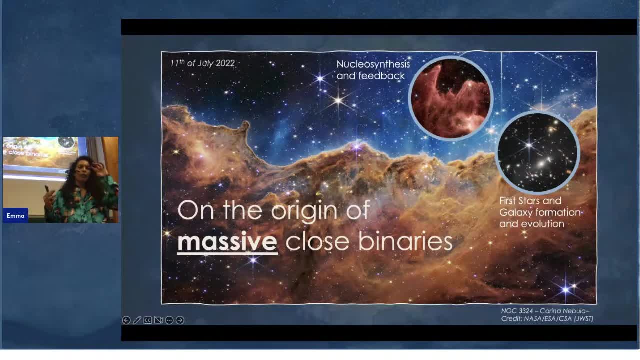 So that all the chemical elements that are created inside the stars are then spread around the industrial medium And that way you fit this cycle of star formation and all the heavy elements that are made of all that you can see around you all come from massive stars. 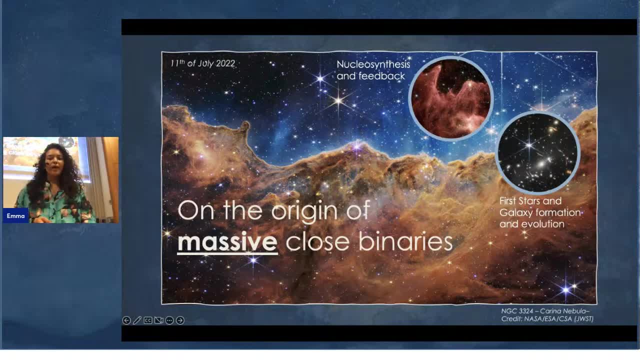 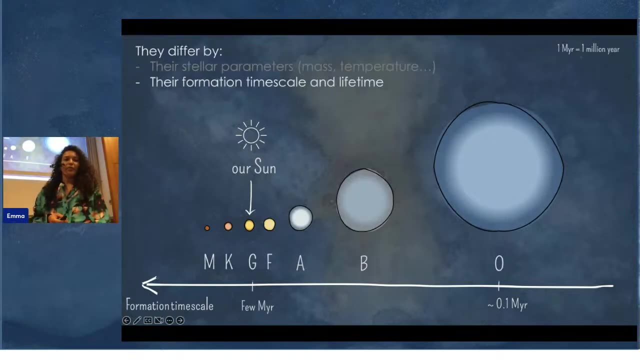 So they are really important And, of course, they also hit the interstellar medium and they can also trigger new phases of star formation. Okay, So if we continue with why we care about them and how they differ with their low mass counterparts, another thing that makes them very different is their formation timescale and left time. 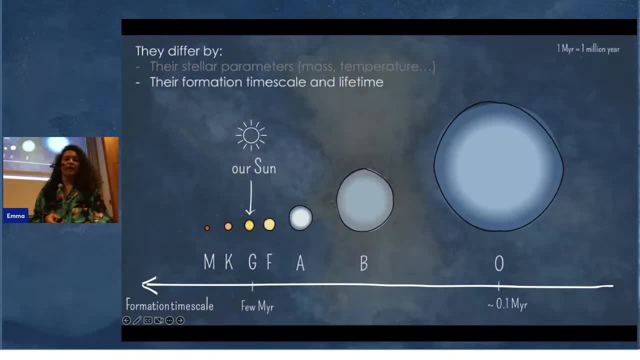 So, if you look at the formation timescale, stars like our sun will take a few million years to build up and to be created, while massive stars perform very fast, in about 100,000 years, So they are much faster to form. 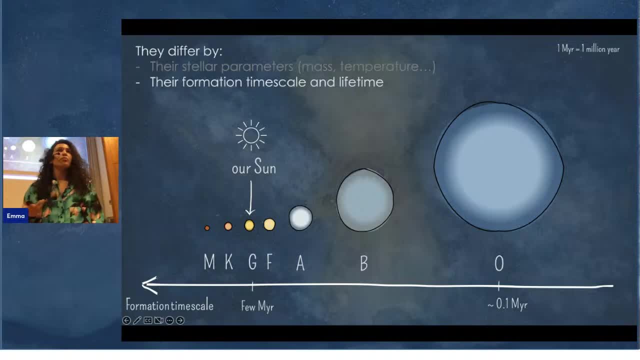 That also creates a problem, because we don't know how we can amass such amounts of material to build such a massive star in such a short amount of time. And then for the timescale. so the maturity of the life of a star is spent on what we call the main system, space. 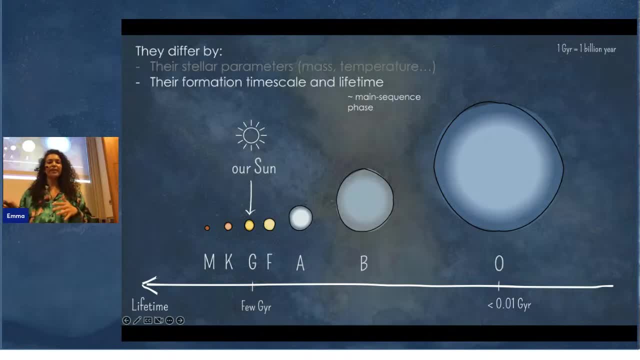 So it's a space that they enter when they start to emit hydrogen at their core And it ends when the hydrogen reserves go to the core and they start burning helium. At that time we consider that they are already entering the, the evolved space. 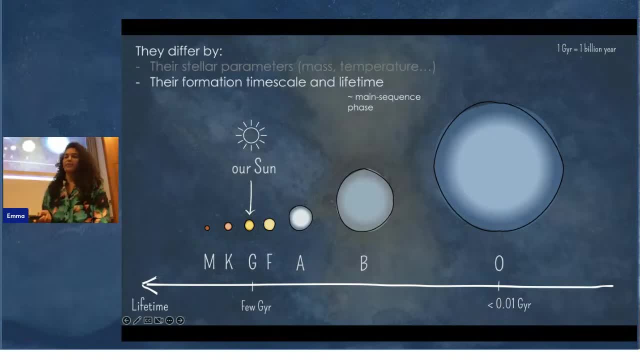 So the overall life of a sun-like star is estimated around 10 billion years. So we have time, because the sun is 1.6 billion years old, While massive stars will live around 10 billion years, more or less. So, to conclude, if we all now decide to build stars now, right now, and we build a low mass star and a star, by that time the low mass stars will be built. The massive star will already have gone through explosion and death. And this brings us to our next point. 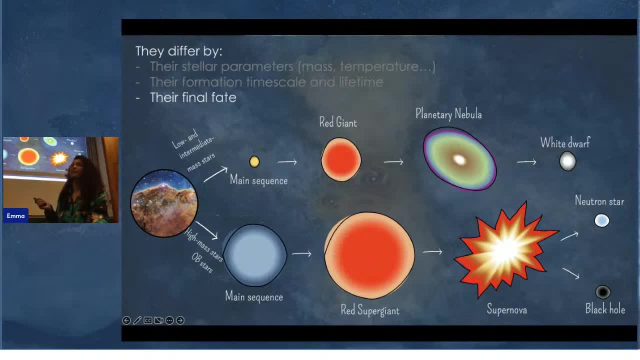 which is the final phase of stars, are really different depending on their mass, So low mass stars will go through this very challenging phase, which is what the sun is going to experience in 4 billion years more or less, And then also will go through this. 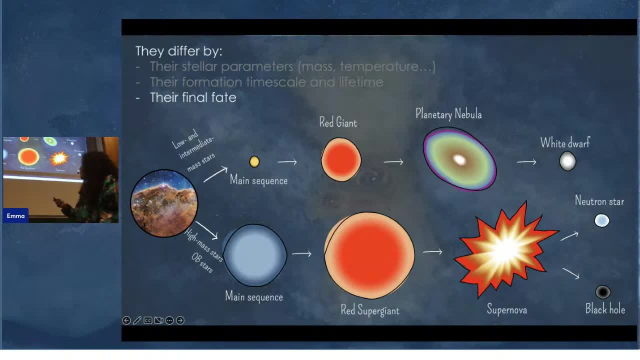 explosion and death as a white dwarf For high mass stars will also go through this wet super giant phase where, during this phase, during this phase, the, the star, will lose a lot of mass through winds and radiation. And this is also a phase where 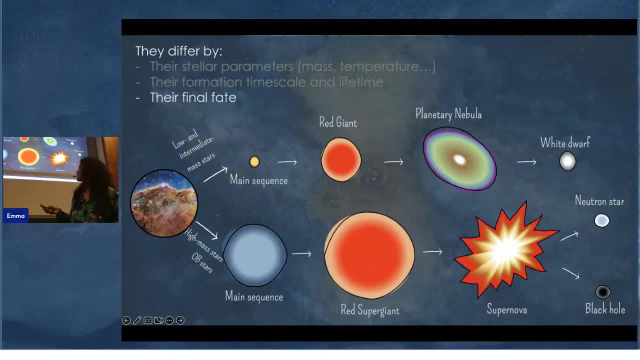 like the interstellar medium, is a lot enriched with the outer layers of the star and they become more intense. If we will go through supernova and, depending on the mass of the high star, it will either create a mutual storm or a black hole. 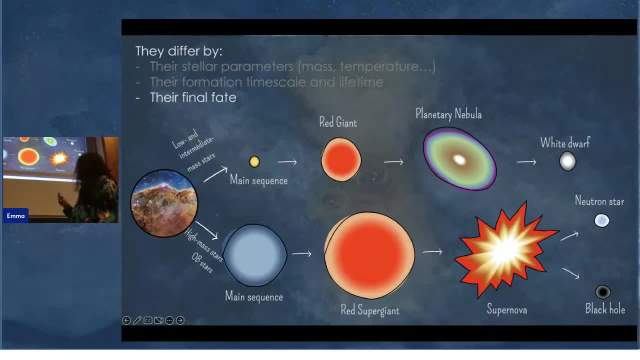 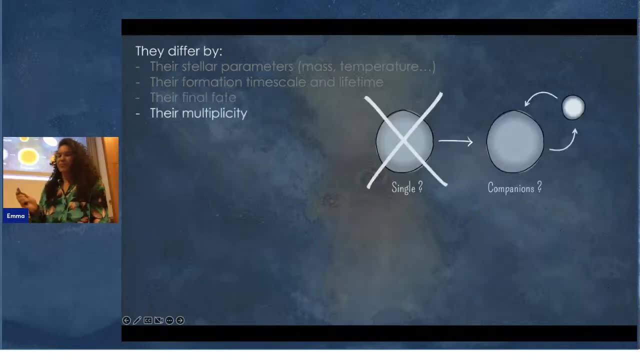 And these objects are like different- yeah, type of death stars. Good, And an important feature that we're going to deal with in the rest of the presentation is the degree of multiplicity of these stars. So usually so, multiplicity is defined as the number of observed central objects. 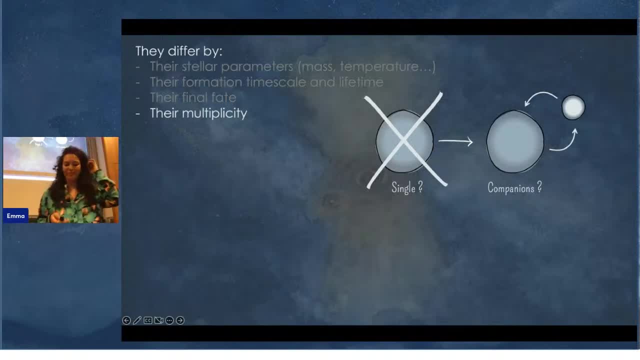 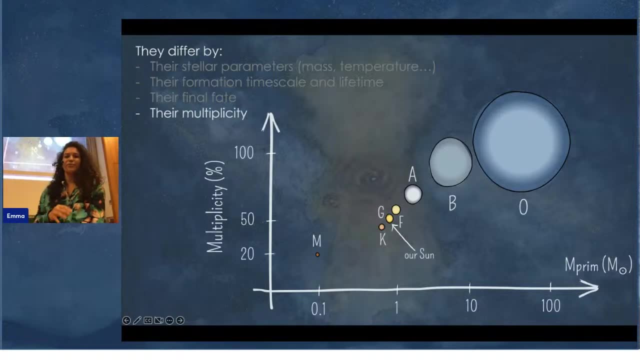 we around which we can spot atoms to be compiled. Okay, So if we look at the multiplicity across the rest of the masses, that is, here on the x-axis, we clearly observe that the most massive of the star the most likely it has a companion. 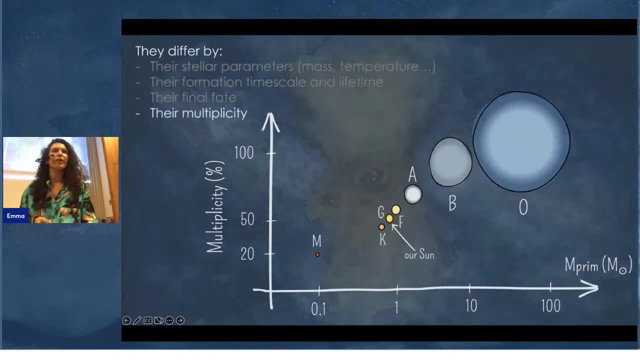 at least a companion Indeed, like for all stars, which is almost 100%, and then it decreases as the mass of the star decreases. And this is a rather recent statement. It's less than 20 years old, I would say. 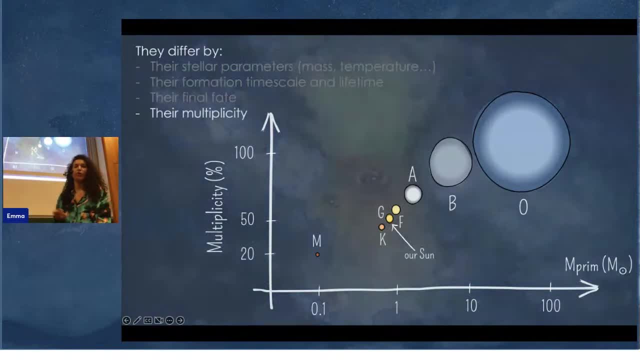 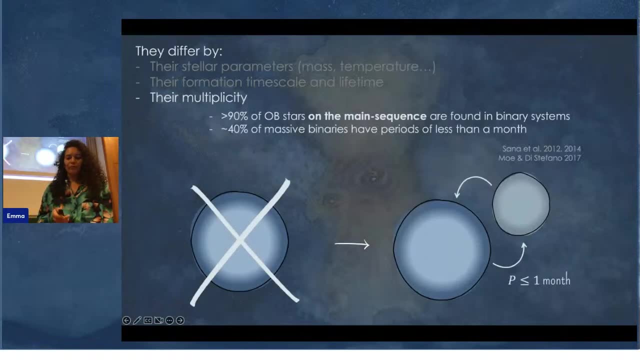 because before we had a lot of observations of certain capabilities to come to that very important result that affects the evolution of massive stars. So I was saying before, more than 90% of all these stars on the rain sequence, so in their main face. 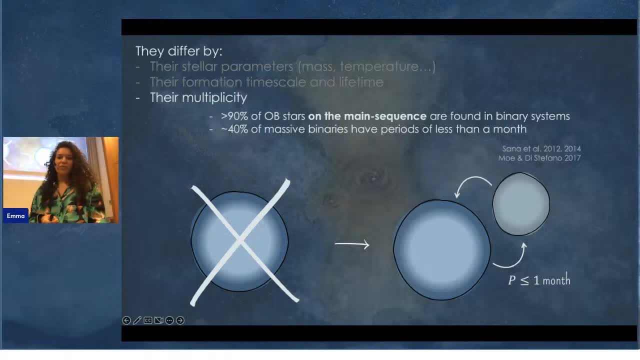 are found in binary systems And the measurements go even beyond the partnership. We were even able to measure what is the period of the separation, more or less, between these stars, And we found that 40% of massive binaries have periods of less than a month. 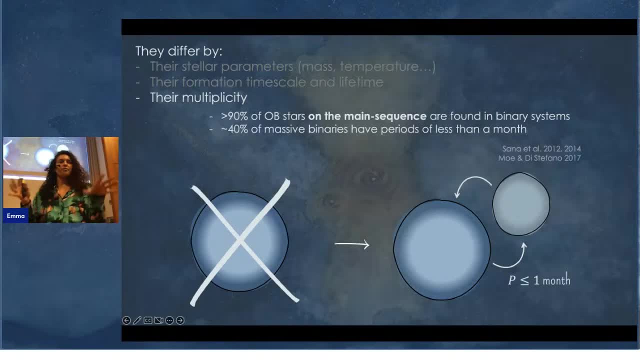 So, for example, it takes Earth, a planet, one year and a few hours to complete a full orbit around the Sun And these stars. they process around each other in less than a month, with sometimes periods as down as a few days. 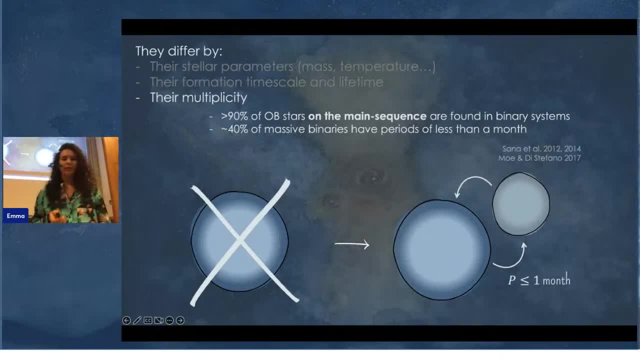 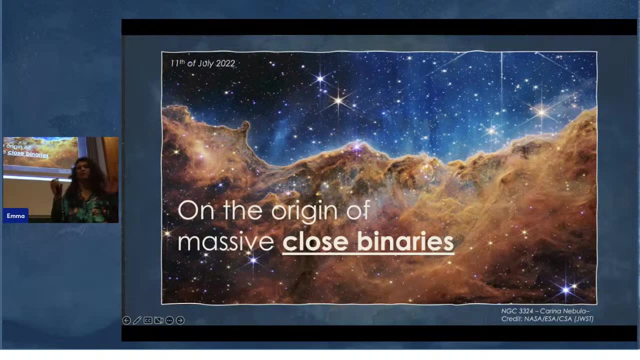 So they're really close to each other. their period is really short, And this is what I mean by closed binaries. It's a system composed of at least two stars- two stars for binaries, actually, and closed because their period is really short. 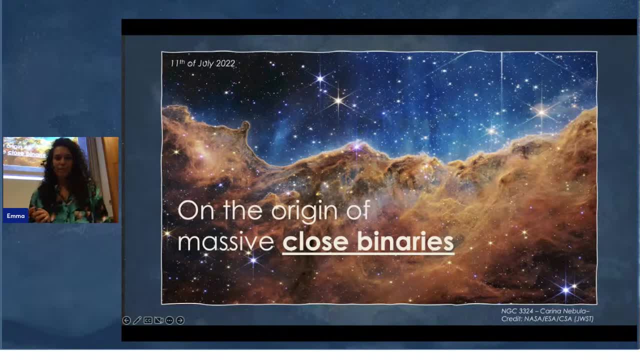 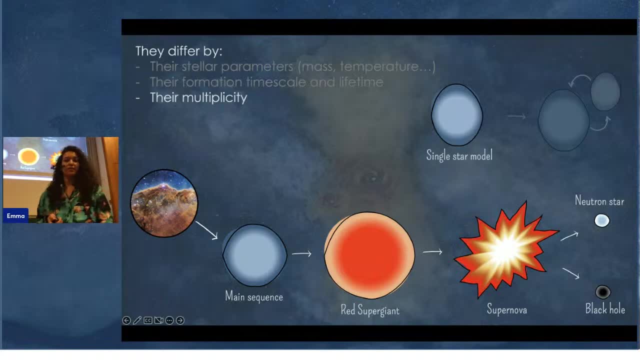 Okay, And these have really strong consequences on massive stars. actually, This is a really not insignificant feature when we deal with massive stars. The life of massive stars will be disturbed and influenced by the presence of a closed companion. So this sketch here is a solution for a single star. 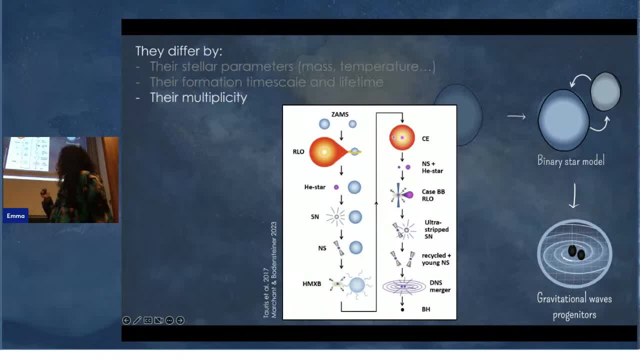 But this one. you see that it becomes much more difficult when we add the companion to the point that you might create a black hole or a binary from two black holes And this will generate a gravitational wave. So I will not go through all of this. 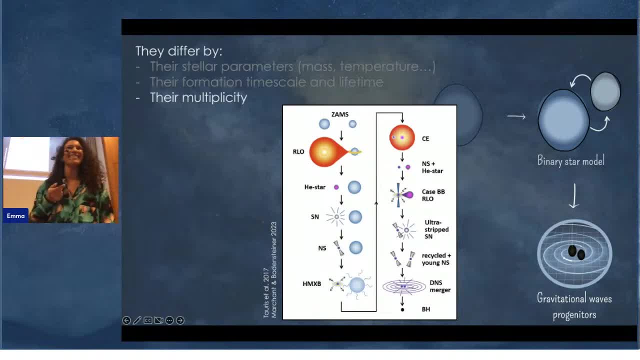 You can talk in the reception. there are a lot of experts in this auditorium about the evolution of binaries, But it's totally bottom line that the whole evolution will be affected. and then you can create coordinators of gravitational waves, which is a very vibrant topic at the moment. 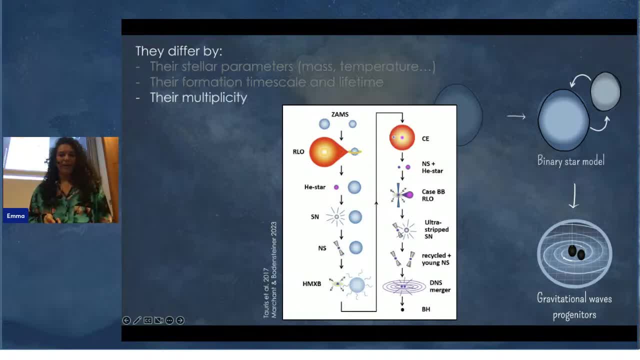 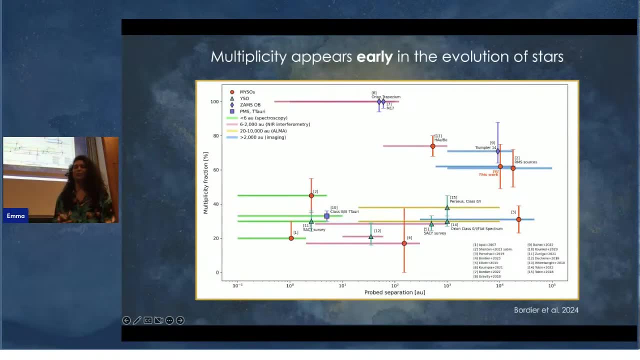 And, yeah, Good. So from different observational studies we know that no multiplicity appears early, very early in the evolution of stars, And that is not a property that they acquire during their evolution. They can have a ripple effect, but even early in the evolution 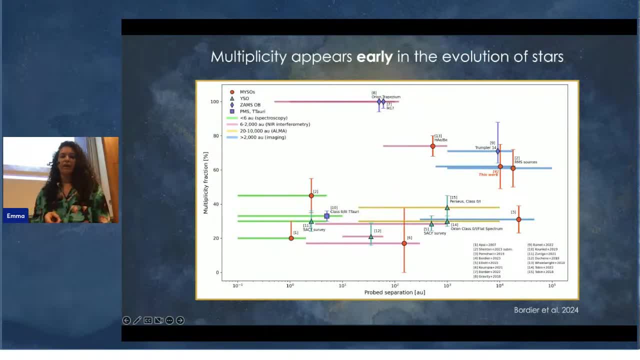 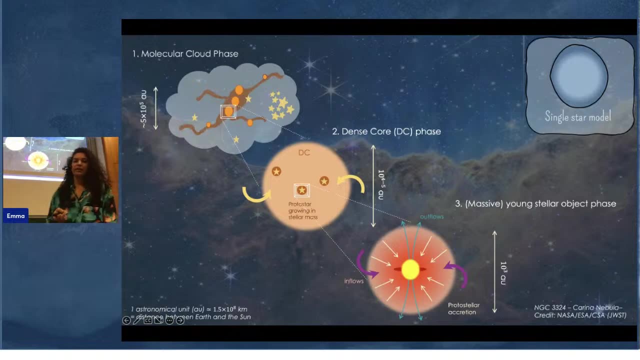 they acquire this characteristic. So several theories emerged, mainly from the theoretical point of view, to try to explain how we can form this mass scenario. So again, this sketch that I showed previously depicts the formation of a single star, massive star. 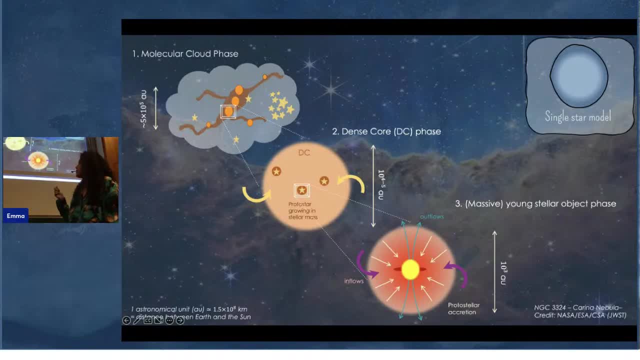 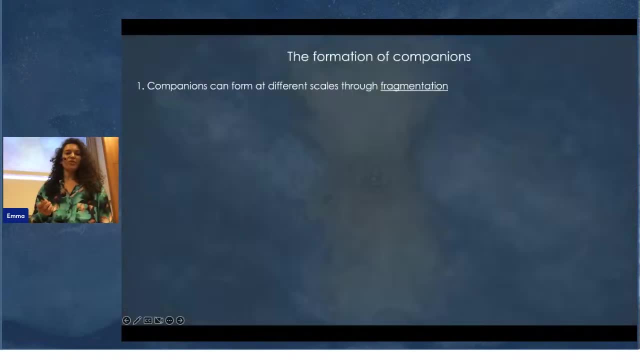 But we're in the phase in this to actually form another companion. But there are different processes. One of the processes is fragmentation. Fragmentation is a generic term used to define the process by which self-gravitating objects develop substructures And these substructures can evolve as a component. 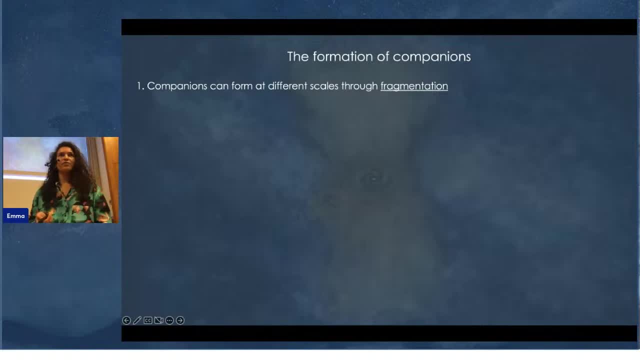 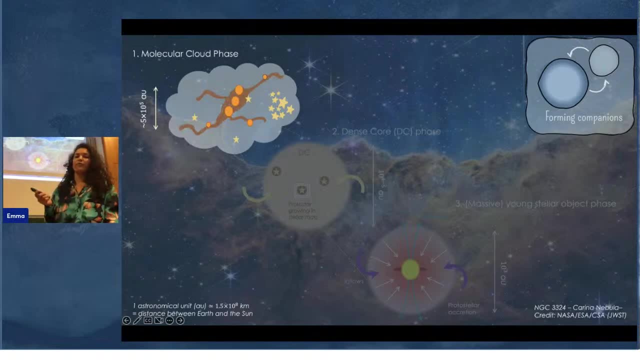 And this can occur at different times and scales during the formation process. First, you can have very clear during the formation process filament fragmentation. So this filament here will fragment into two. they will create two cores at very large situations And fragmentation can also happen. 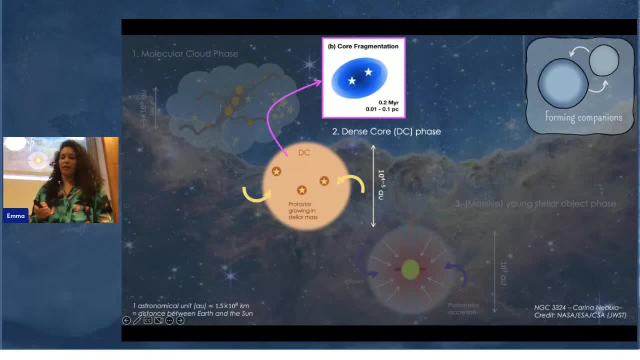 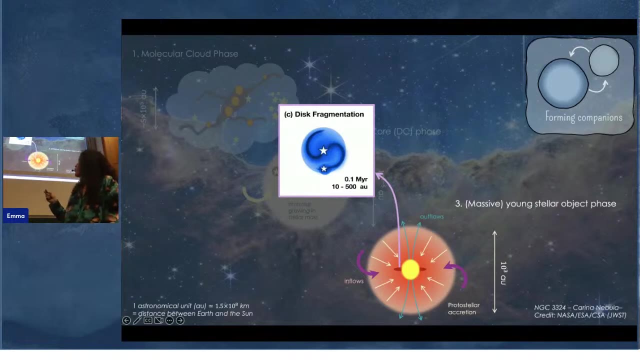 during the core phase. Here again, like this big core and this big base can fragment and create two stars, And at the smallest you can form within the operations. here you can form components to a process called dis-fragmentation. and this is how the form 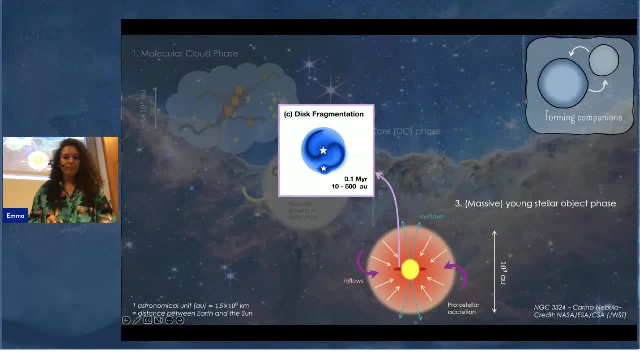 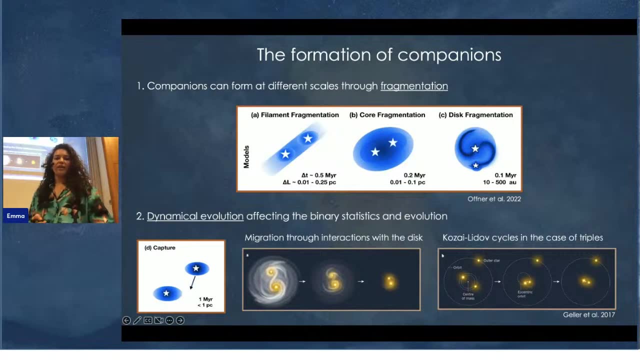 is composed by components- Good- And there is another channel that are the dynamical evolution. So dynamical evolution is due to the gravitational interaction between bodies and do not longer depend on the gravitational collapse. That depends on thermodynamics and fluid properties of the medium. 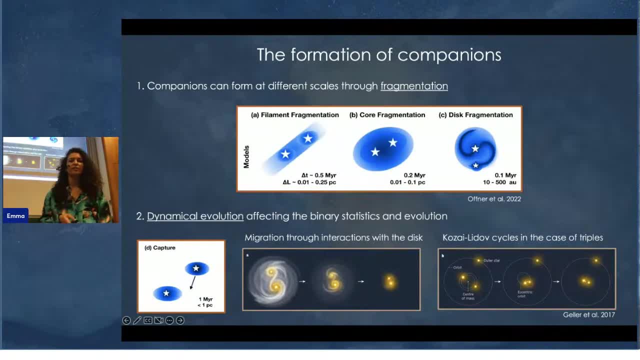 So it's really like dynamical interactions between the bodies themselves And for the formation of close binary physical processes that are most likely to play an important role are the migration through the disks that will form a component within the disk and that are like migration processes. 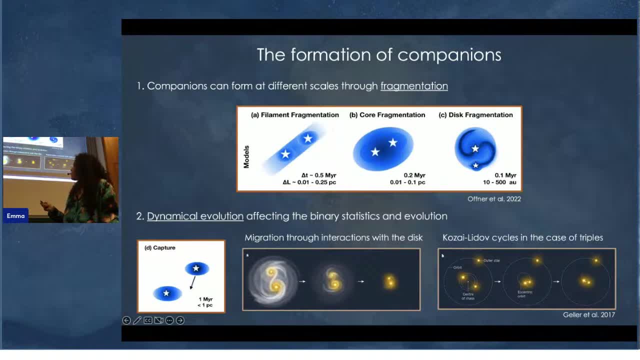 that will push the second component towards the central one And it will live like a tight binary in the end. Another process would be: you have the influence of another component, so a single component that is outer and due to dynamics, dynamical evolution. 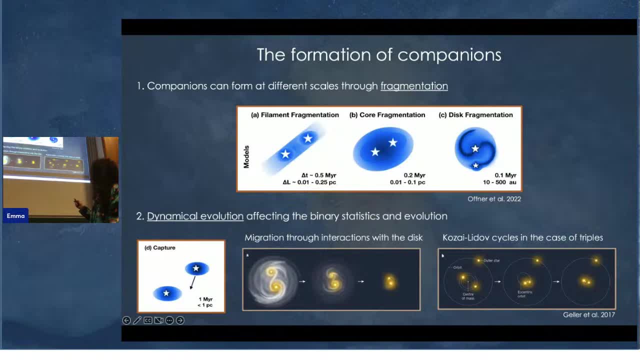 this outer component would strongly influence the orbits of the inner binary here, to the point that they might end up as a really tight binary. There is another process that we call capture, which is basically a store, and a companion binary system will attract another store that was not initially bound. 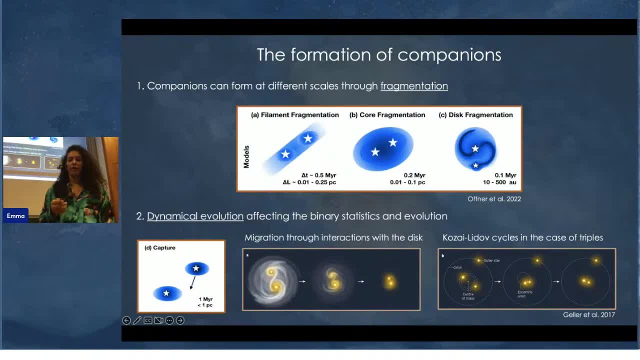 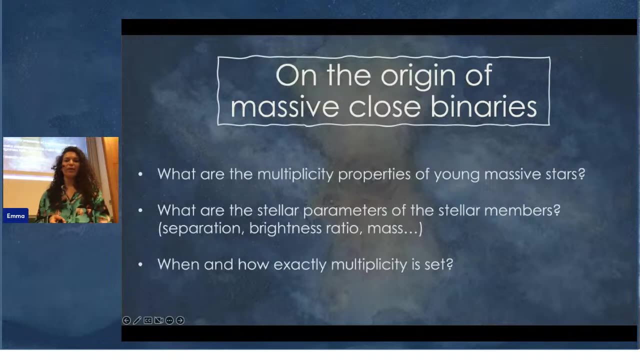 to that system and they will come together and be bound for the bit of their life. Good. So this is exactly where my PhD project comes in. So now that you understand all the terms of the title here, let me introduce you to the main objective of the thesis. 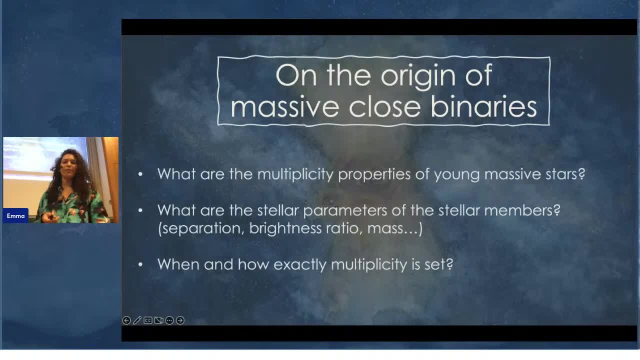 So, first and foremost, we need to evaluate multiplicity in non-populations of massive stars to know whether multiplicity is in fact or if multiplicity- sorry- in fact extends to the various stages of a massive star, And by doing so it mostly leads to our 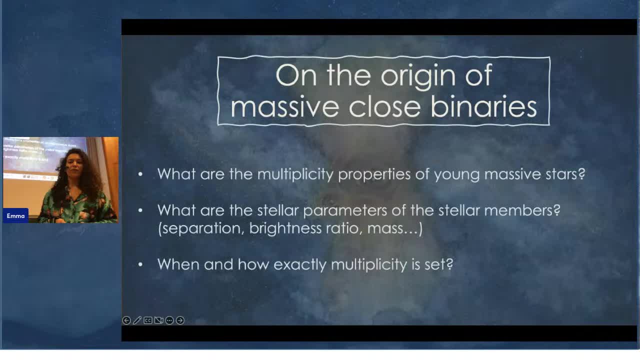 second main objective, which is to understand when and how exactly multiplicity is set. In particular, what are the pairing mechanisms? that leads- So yeah, it leads us to our second objective, which is to understand when and how exactly multiplicity is set. 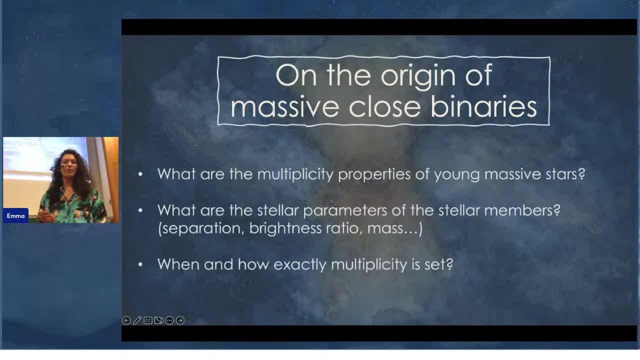 during the formation processes, and what are the pairing mechanisms for how we form multiples, and what are the observational imprints or signatures that could lead us to one or another formation mechanism? So these questions, of course, are not addressed accurately, but we'd rather try to keep. 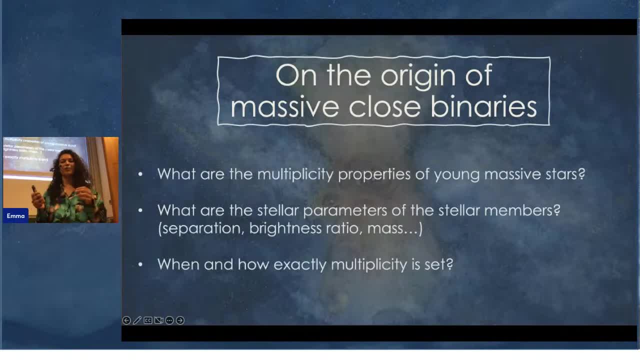 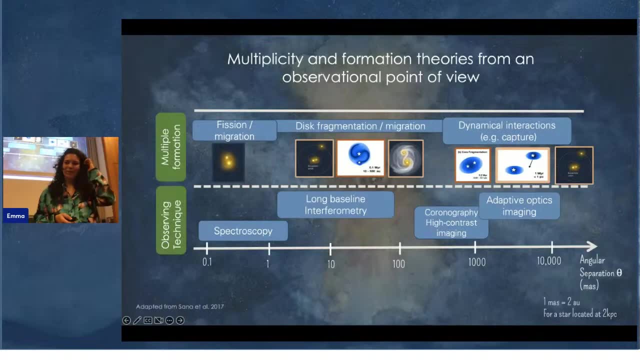 these three main questions as the driving line for each of the projects that we are conducting. Good So to me, these objectives. I will mainly rely on observations, However, just as mentioned earlier, the physical processes that lead to the formation of companions. 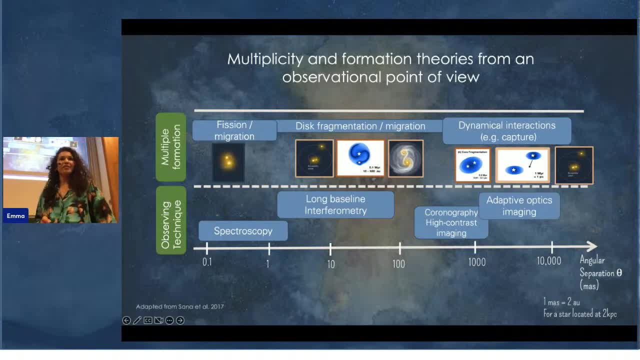 have different scales of action, which means that different observational techniques will be required. and those different observational techniques will trace different spatial scales around the star we are observing And, of course, it will trace different physical processes, just as I showed earlier. So one of the processes- 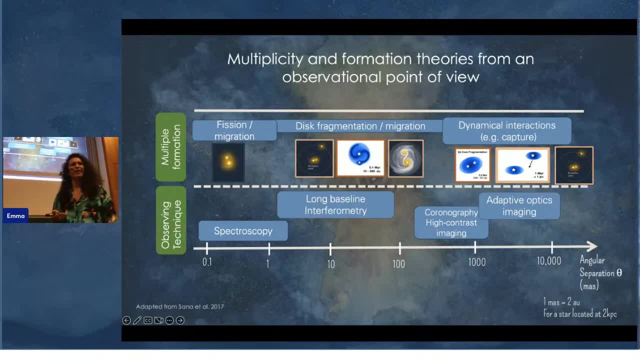 we first want to try to understand or test in more details is the inward migration that I showed you through the migration disk. So how can we do so? A good proxy for inward migration is the presence of at least one or more companions. So what we want to do, 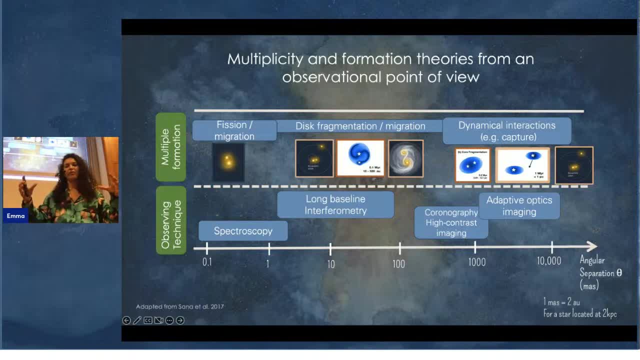 is to test the expected size of the accretion disk, And that accretion disk for a massive star can extend up to 500 AU. So we want to test actually what is the companionship in this range here. And you see that. 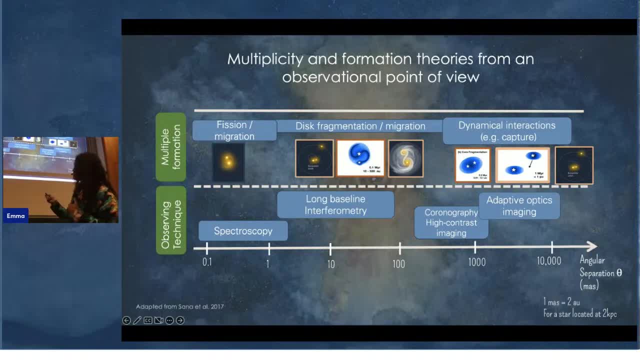 it exactly falls into the use of long baseline interferometry. So this is what we used in the first project. Now, maybe this is even more important than the first project. So this is what we used in the first project. Now, maybe this is. 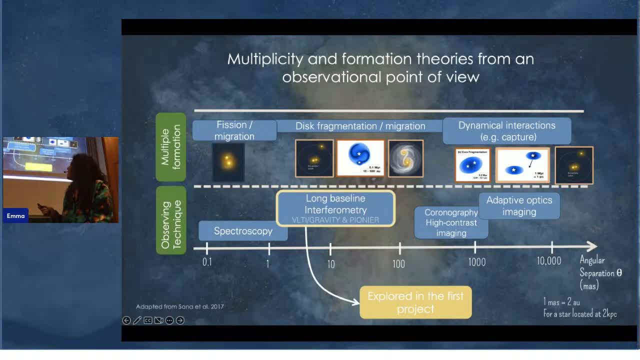 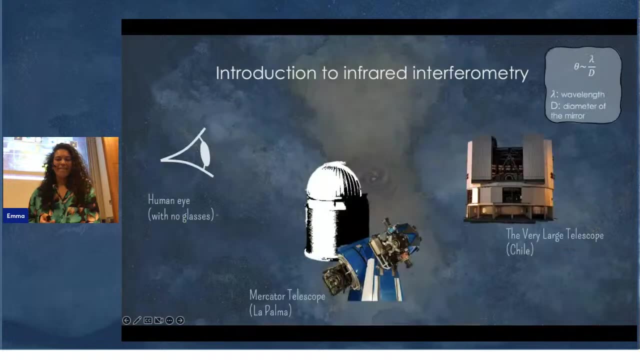 even more important than the first project. So this is what we used in the first project. Now, maybe this is even more less understandable for you, So we'll try to quickly explain what is long baseline interferometry. Okay, So we astronomers usually choose the telescope. 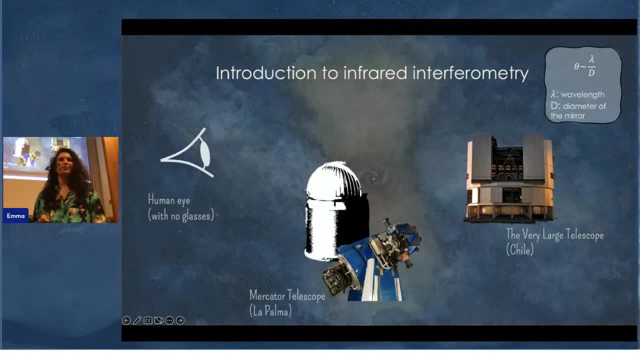 and the observing technique based on the angular resolution that it can deliver. So the angular resolution measures the ability of a telescope to distinguish small details on a celestial object. It is therefore defined as the theta here, which is lambda over d, So this parameter may depend on d. 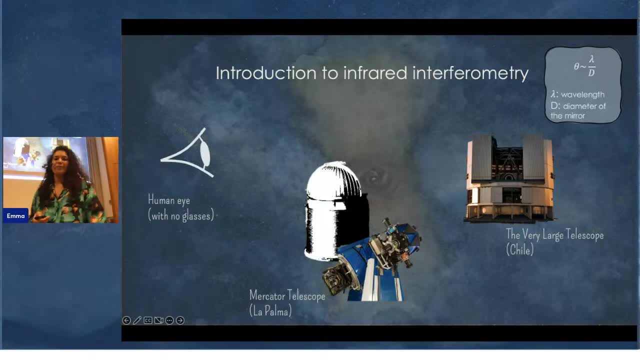 which is the diameter of the mirror of the telescope and the wavelength at which you are observing it. Good, So let's take an example. The human eye actually has a lens, is a telescope, and we have here these very famous three rocks that we can see. 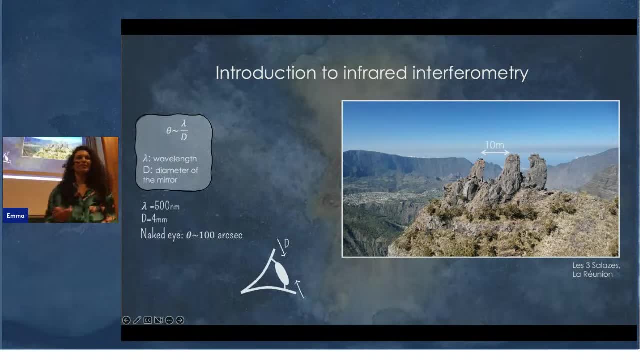 here. So this is the telescope, and we have here these very famous three rocks in La Réunion that are called Les Trois-Salins, and they are separated by more or less 10 meters. So the human eye has a resolving power of 100 arc seconds. 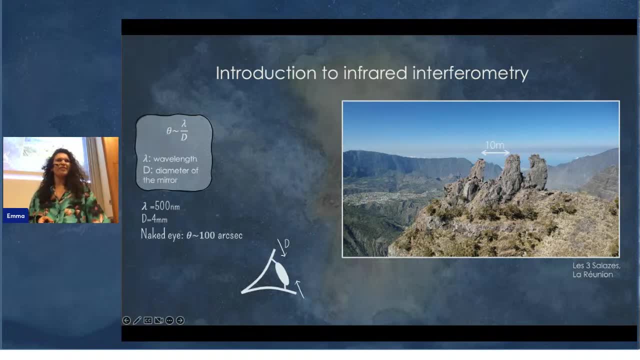 considering that the pupil size of the eye- someone that doesn't wear glasses and doesn't have any autism- is 4 millimeters, It can actually vary between 2 and 9.. I made some research on that, So the human eye has a resolution. 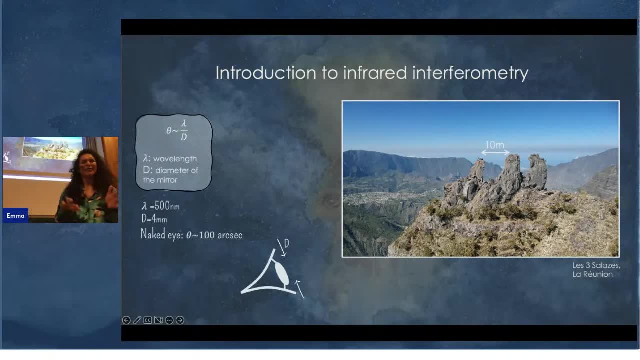 power of 100 arc seconds, considering that the pupil size of the eye is 4 millimeters. So everything can be found in nature. So we wonder how far can we go, or how far can we also be, so that it still distinguish the two peaks? 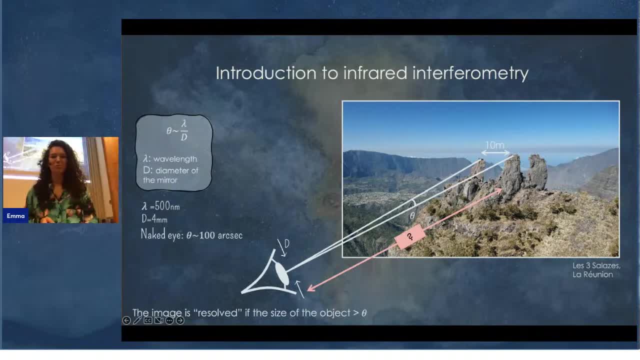 and that it's just a massive rock or massive shape that you would see. So, for the human eye, at the limit distance of 20 kilometers you can still see the two peaks of the mountain, and I did some calculation for my friends in La Réunion. 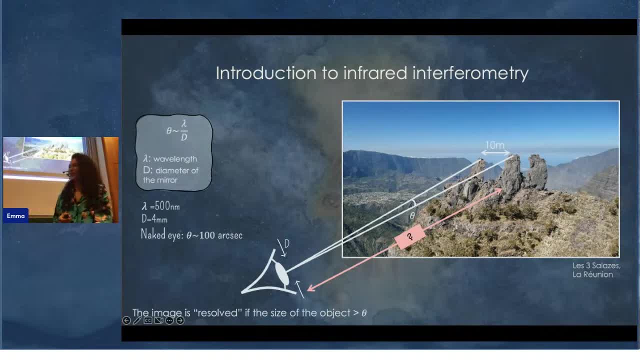 to go to the viewpoints of Camp Noir. you should still be able to see the two peaks, and if you don't, maybe you can push an appointment to the doctor. Good Then, yeah, we have another very famous telescope, that is at Cahiers d'Aubin. 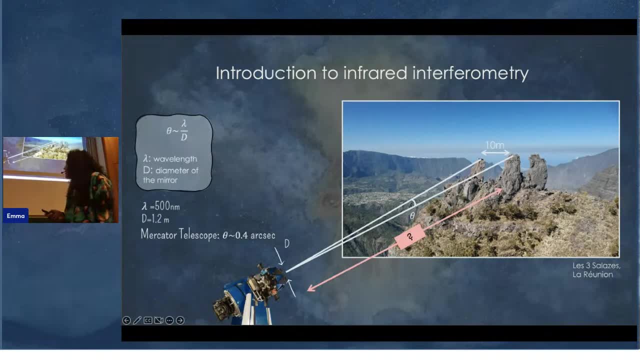 which is 14. In La Palma. So this telescope has a diameter of one point meter and is operated by, I guess, in the Canary Islands. So here the resolving power draws two time form, arc seconds. so it mainly says that at a distance of 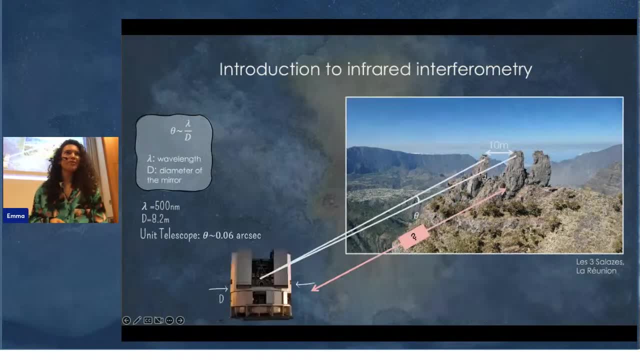 35,000 kilometers, you will still distinguish this two peaks from the other two peaks. and then we go even bigger with the telescopes in Chile that have a diameter of eight point two meters. so this two peaks and 35,000 meters, to have an idea. 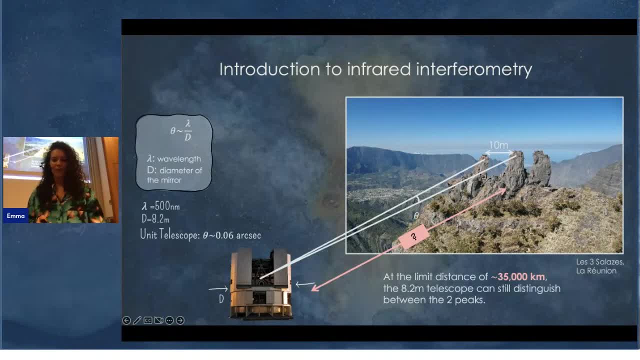 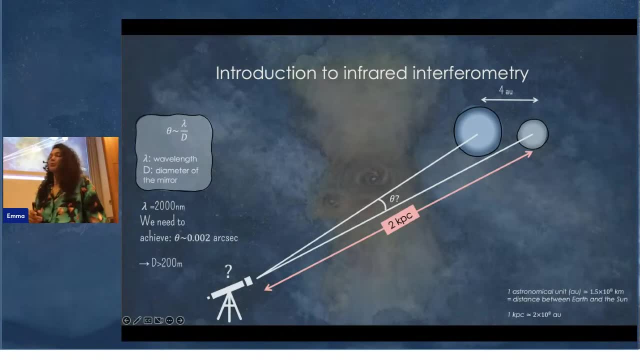 is almost twice the distance between the north and the south pole. Good, Now let's reverse the problem and look at what resolution we would need to perceive two stars that compose a binary system. that is one astronomical unit. so one astronomical unit is the distance between 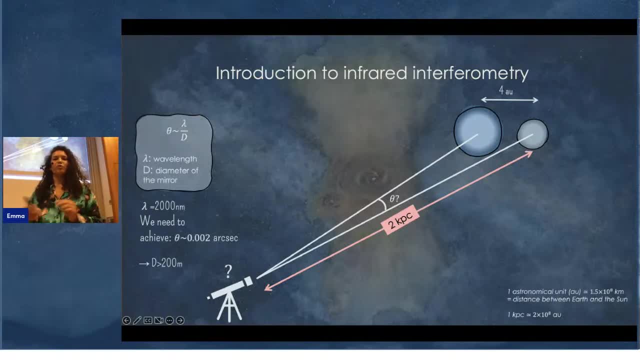 earth and the sun, and this binary system is located at two kiloparsec, which is a typical distance defined by six stars. so two kiloparsecs. so if we want to look at this system at such a big distance, we need a resolution of two. 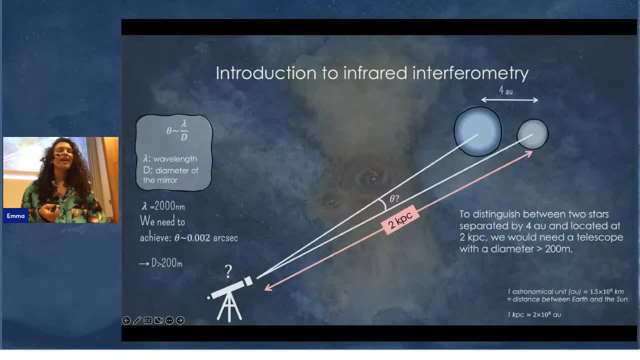 milli arc seconds, and this corresponds to a telescope with a mirror of over 200 meters. and we know that we have some problems because we cannot build this now. maybe in the future we will, but then we still want to see this type of object. so we 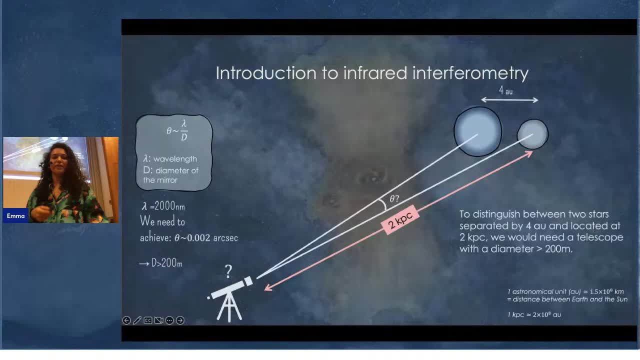 have to find about an idea, and this is how astronomers came with the idea of astronomy. oh, interferometry, sorry so. interferometry is a physical tool that is used to combine the light of different telescopes to try to understand or to see the satellites and the asteroids. 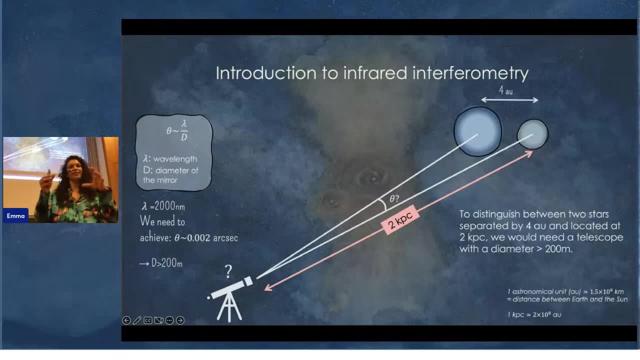 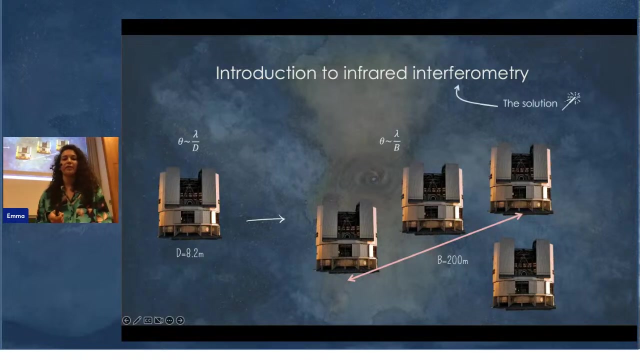 so you combine the light from different telescopes- two or more- in such a way that you wish, and this is what was done um in different places in the world and, for example, here i will give the example of the VLTI, which is a very large telescope. 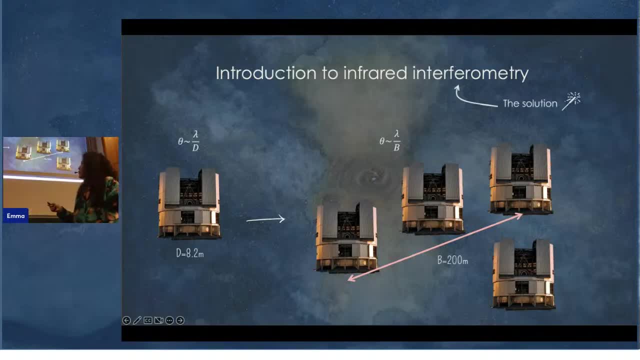 interferometer array in Chile. um, so this is how. basically, the base line is 200 meters and somehow we have created a telescope of the virtual size of 200 meter diameter. um, now, what matters is no longer, so, as you understood, the diameter of a single telescope. 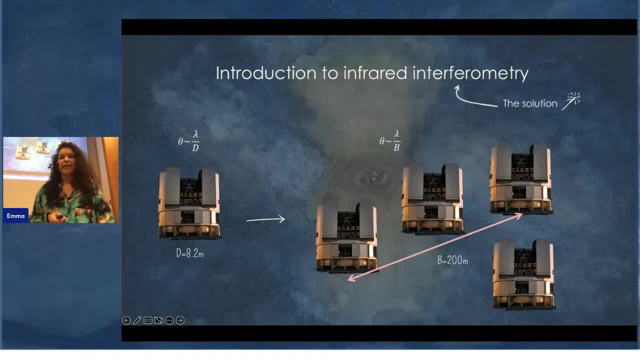 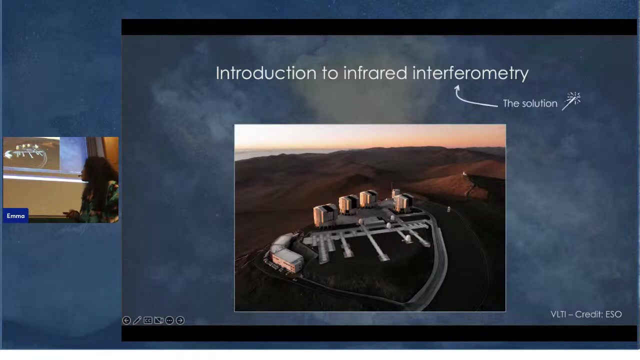 the separation between two stars or b, and that way we can distinguish between two stars of a binary system that will be located at two kilo parsecs, uh, and with a separation of four astronomical units. good, so this is a very nice picture of the telescope is recombined. 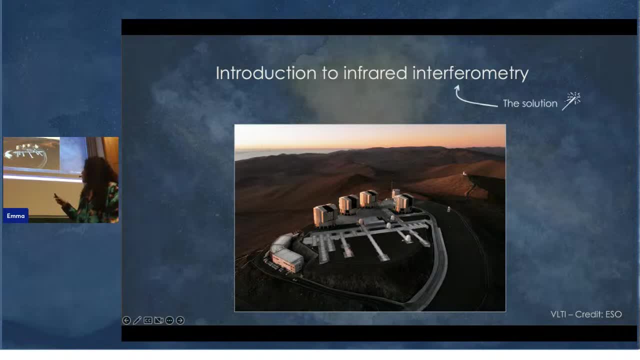 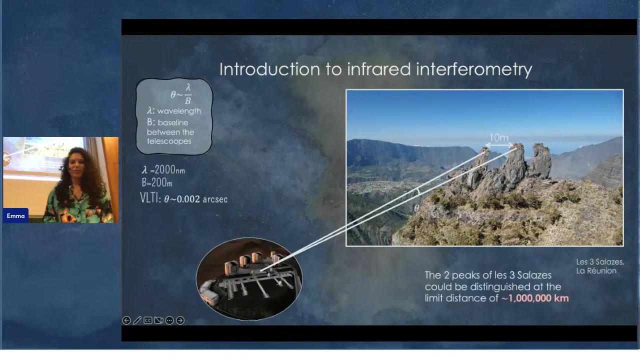 in this lab here that you see. so thanks to like data lines that are located uh under this platform. um, we use delay line to make all the beams uh interfere together and then this is what we made from the detectors. so if we use the lti, then the 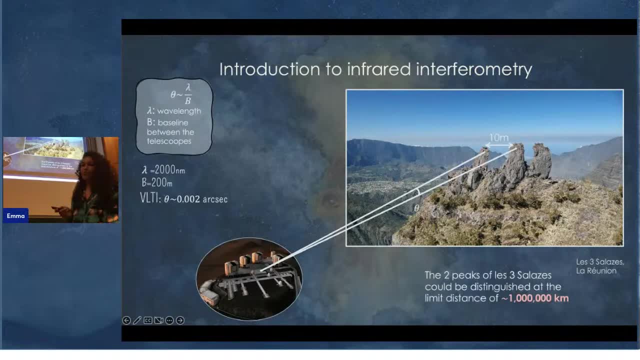 two peaks of the frozen earth um could be distinguished at a distance of one million kilometers. it is three times the distance from earth to moon, also the distance between us and the james. but we could also see that would be standing on top of one of the two. 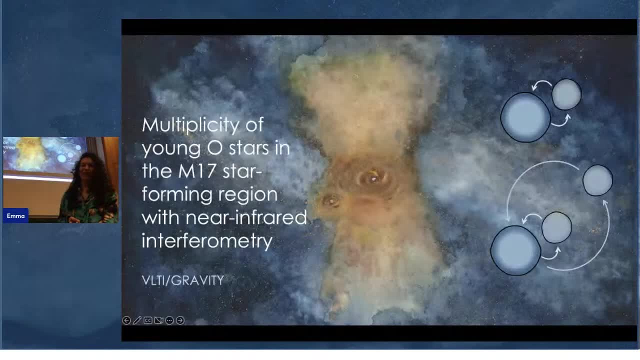 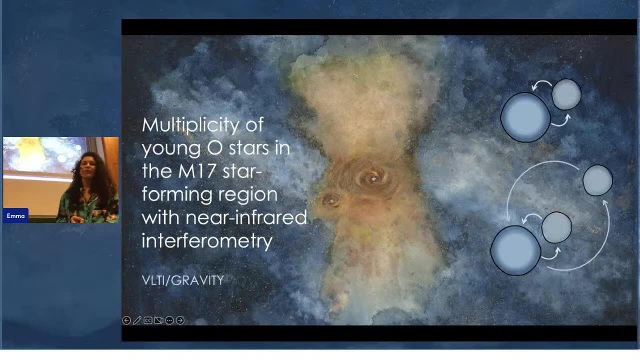 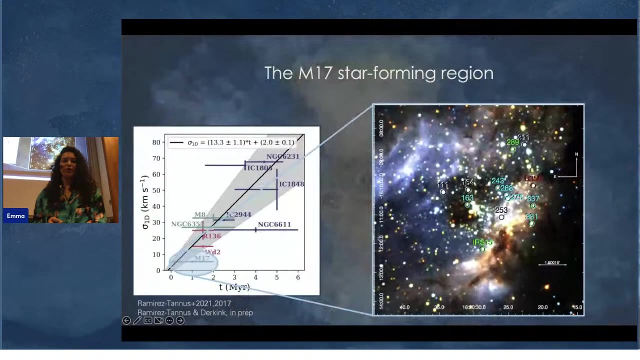 peaks. good, with all this information in hand, let's talk about science and the project i conducted. so i looked at the multiplicity of young posters using near red interferometry and i wanted to test the migration scenario. so we use this star formulation here: m17 that. 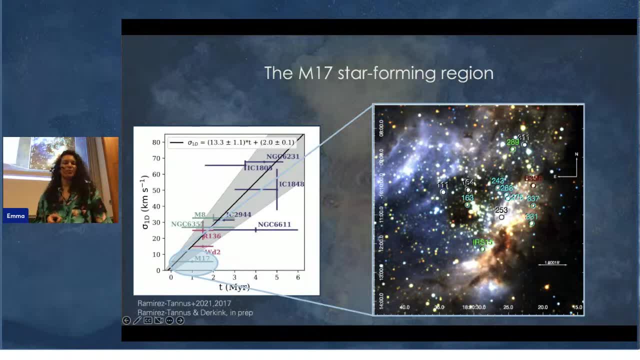 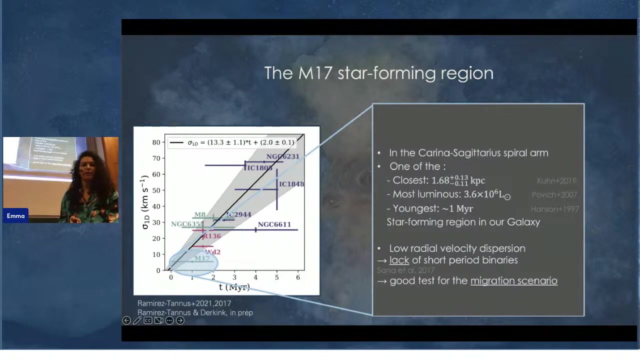 um shows very low radial velocity dispersion. so here the terms are more technical, but it mainly means that most of the boundaries in this are rather um large separations and periods. um in the carina sagittarius spiral arm is one of the closest, most communist and youngest. 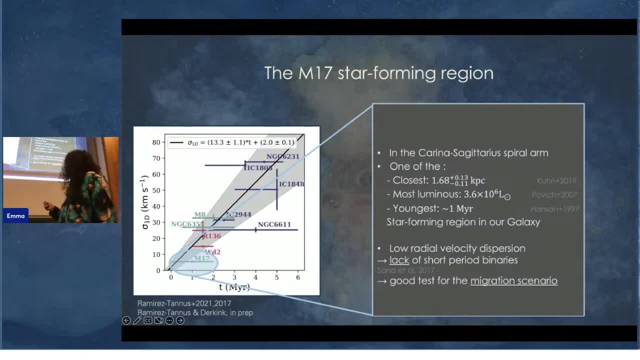 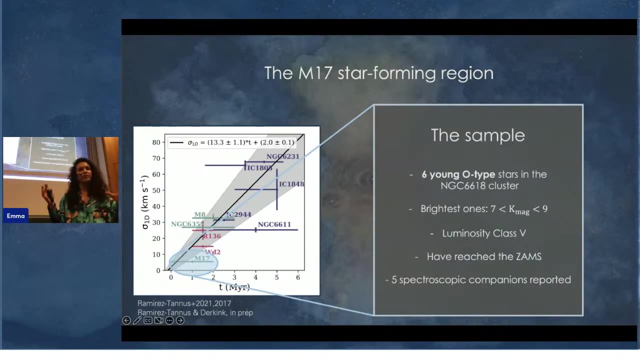 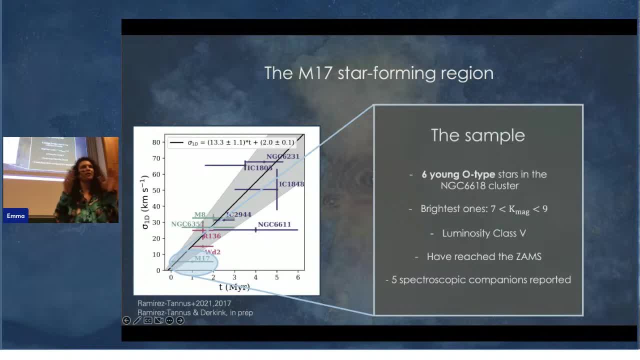 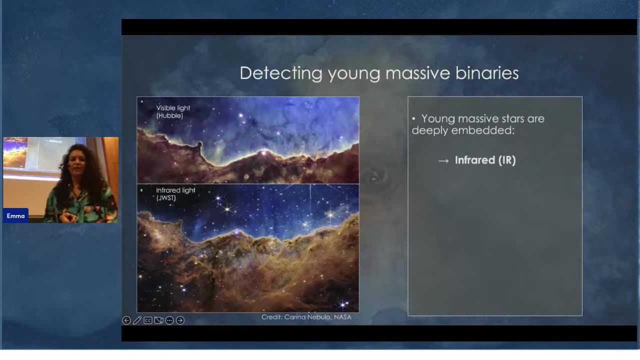 the, the, the, the, the, the, the uh, the uh links to miejsc of uh and and changing to different última tons um. this um: you have um and in the mid-infrared with a James Webb Space Telescope, And you clearly see more stars in the bottom image. 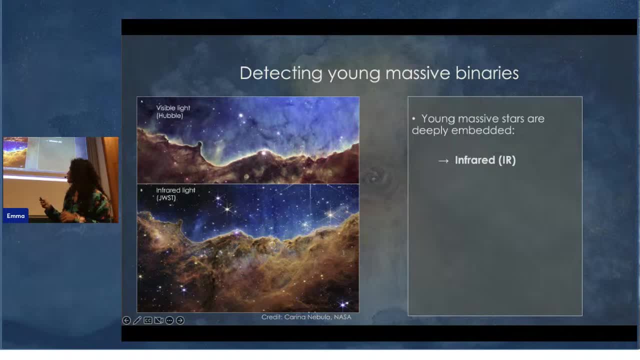 than in this image. For example, if you take the region here in that mountain on this curve here, you see that you can see you can go deeper. It is the same for massive stars. So, on top of being located in such regions, 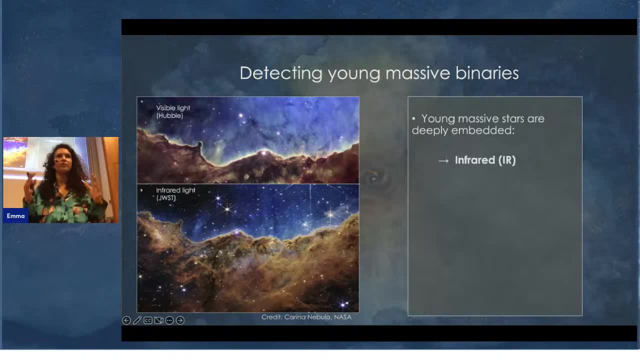 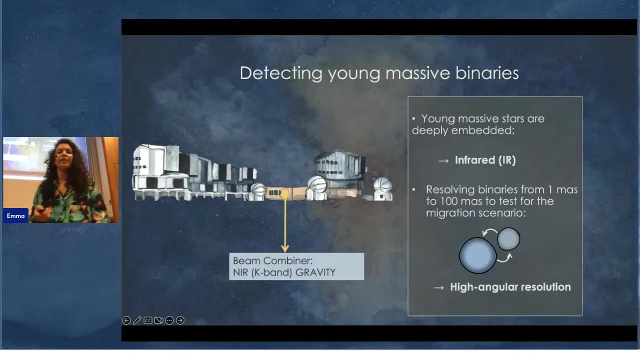 young massive stars are also embedded in their own dusty envelope, So we really need to observe them in the infrared to try to see inside this envelope. And then, of course, we want to resolve binaries from one milliard-second to 100 milliard-second. 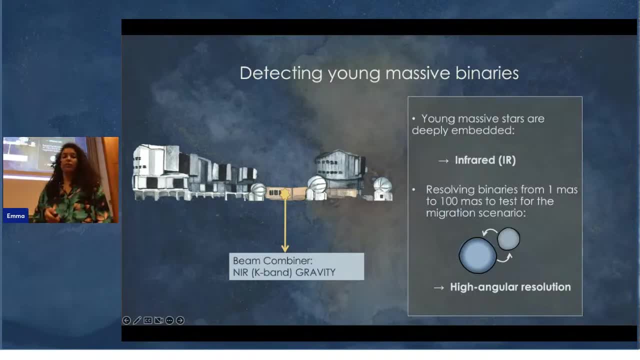 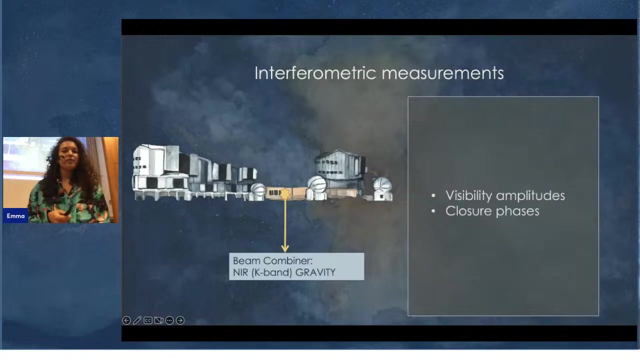 to match the size of the disk And we require. So we used the VLTI, The four UT telescopes, And we used the instrument gravity, which operates in the K band, so it's 2.16 micron And with that interferometer actually. 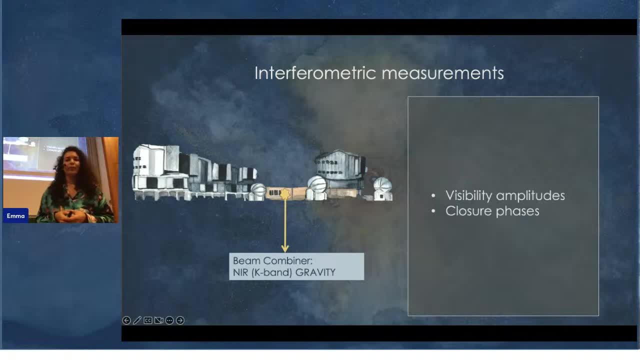 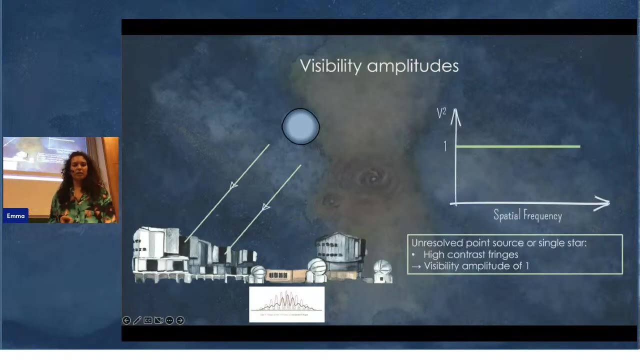 it does not produce a direct image. It provides the observer with two main interferometric measurements. So I will try to explain you quickly what type of data we get with the interferometer. Most common measurement in optical and infrared interferometry is the measurement of the amplitude of the fringes. 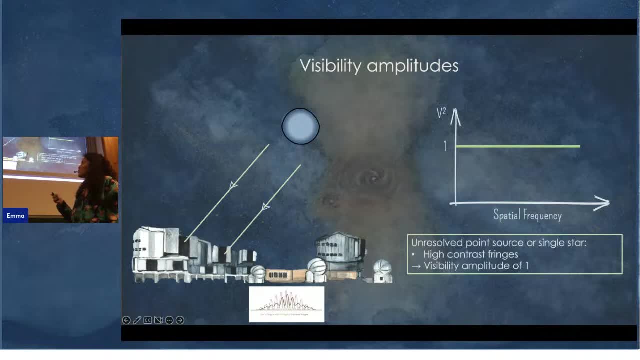 So, as I said earlier, we will collect the light. So I just put two bins here, But of course it goes to the four telescopes And then this time from the four telescopes if we combine in this bin combiner. 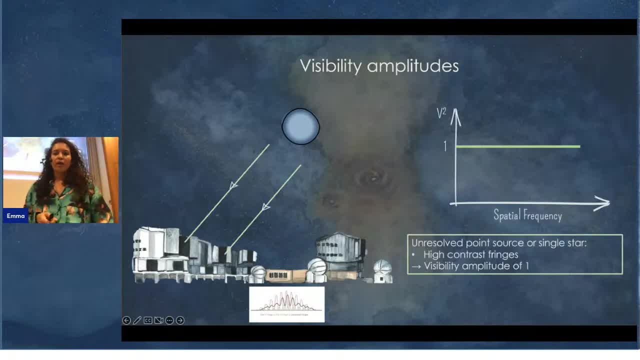 and we get this interferogram here And what we measure is the fringe control, The fringe contrast that we call the visibility of the fringes. So in a resolved point source we have a high contrast fringes and a normalized visibility of 1.. 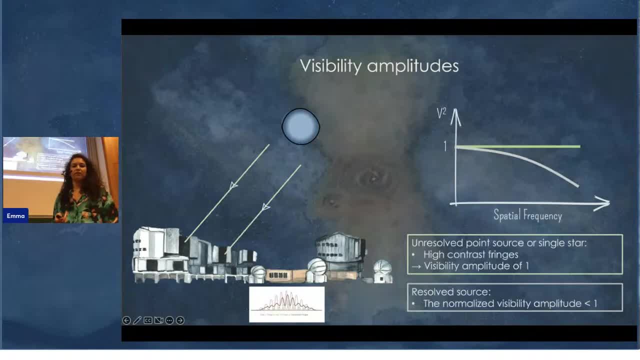 For a specially resolved star, which means that the theta, well the size of the star, bigger than the resolution of the VLTI light from across the star surface. So we take that surface combines in inherently and this will cause a decrease in the French. 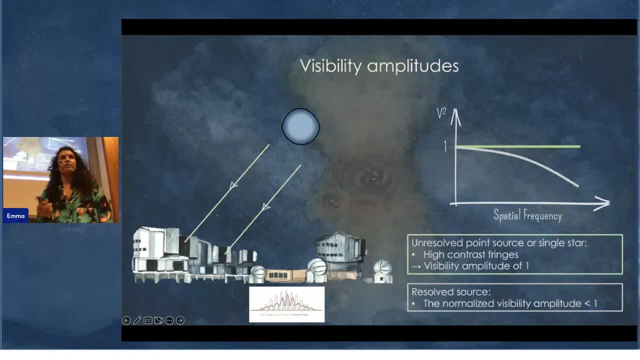 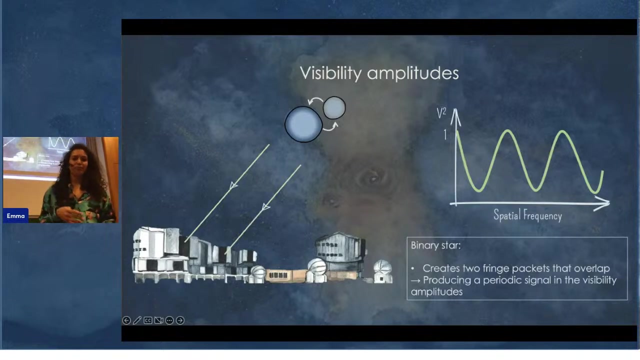 contrast that measure and therefore a drop in the city and you so the normalized visibility amplitude for result stores. now for binary system. so binary star will produce two which packets? and one for each star in the system. so if the separation between stars is small enough, the French packets. 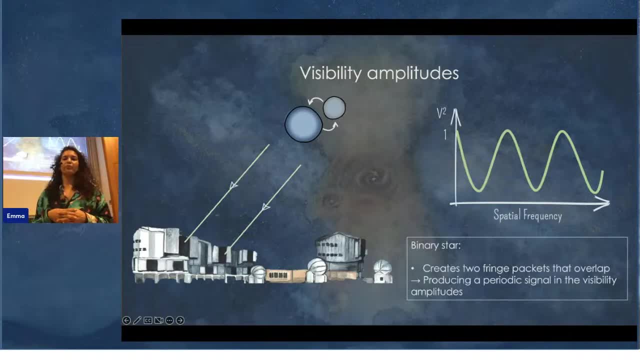 from each start, they will overlap and will produce a periodic signal in the visibility. the separation between the peaks in the visibility, in the visibility curve, provides a measurement of the binary separation and measures the trust ratio of the binary system. and this is exactly the type of signal and then we have a. 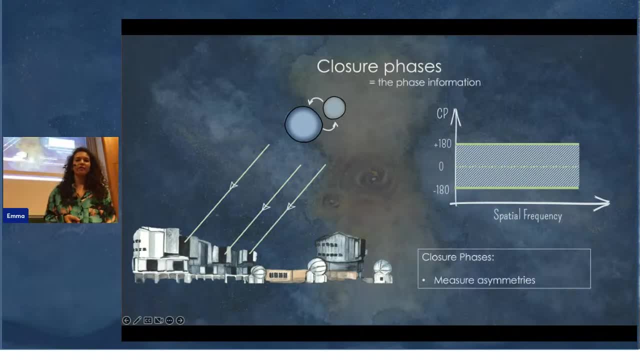 second, in parametric measurements that we call the closure faces and it gives us the face information. I talk too much about this, but basically, if you have a single in the current basis, it's my very- between minus one right and um, it's you information about the asymmetry in the system, such as like: 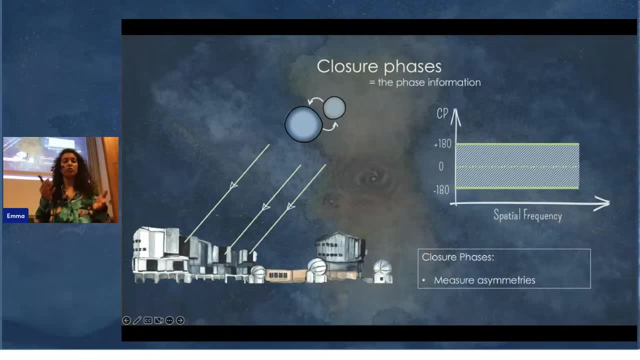 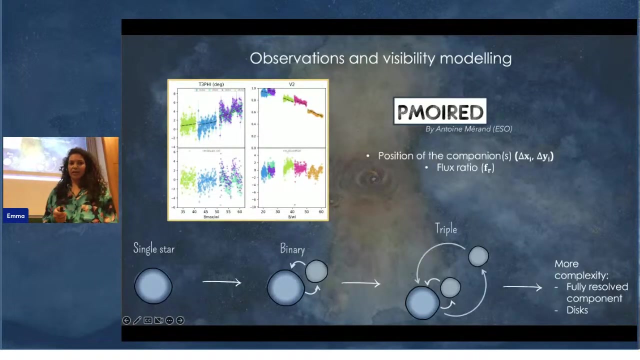 a difference in the brightness, in the, in the different in the two components. a star with a brighter? that's probably the reason. asymmetric this or this one of the stars? yeah, so it gives additional information on the structure of the source. good, So in practice this is how it looks in performative measurement. so you have here the proper basis and here the validity. 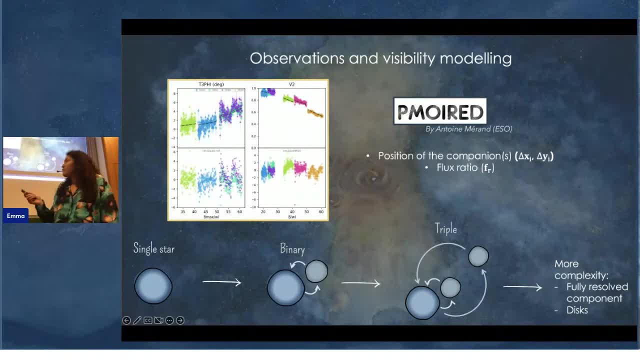 For each system, so we have six of these, because we have six sources, so we have six sets of data, and for each system we use a modeling tool to try to recover the structure of the objects that we are looking at. So we use models for that. so we kind of build our models to try to reconstruct either a single form, a binary form, a triple system, a quadruple system. 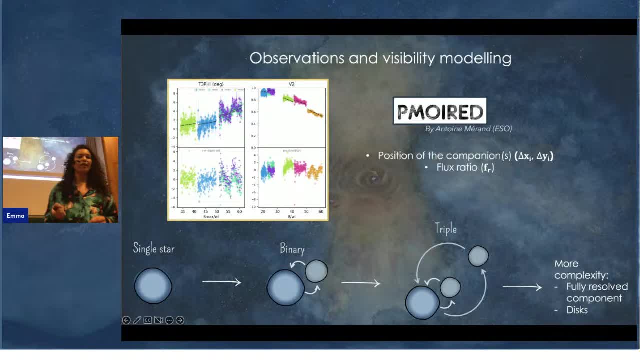 until we are satisfied by our calc score, which means that the model really fits Well, the data. and then we can say, okay, I found a binary system, a single star, because I don't have a signal. and then you can also add more complexity, such as full-risk components, disks or whatever. 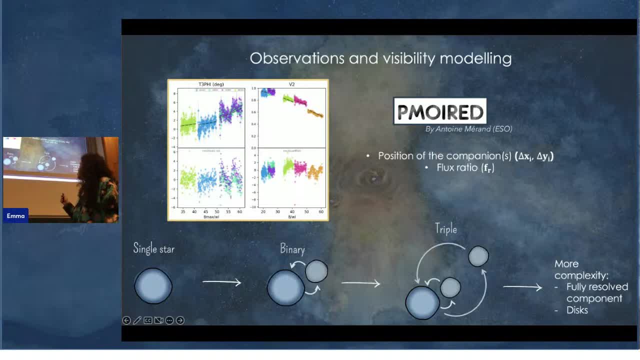 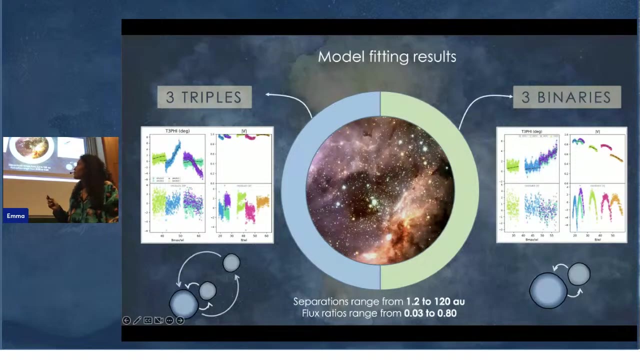 So the main parameters that we measure are the position of the compilers and the flux ratio between the central star and its companion. What we find In our data sets is three triple systems and two binaries, all of them having a separation range from 1.2 to 128,. 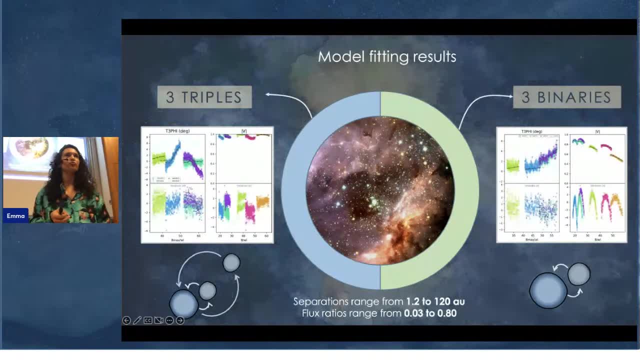 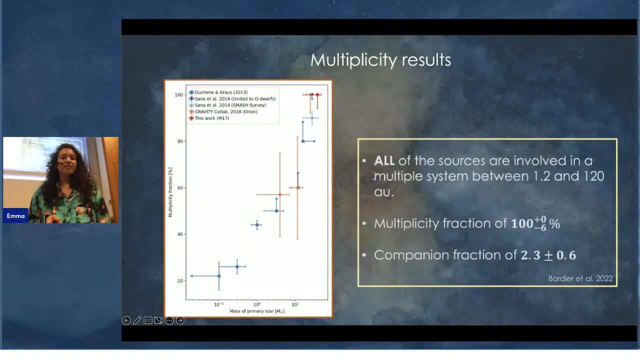 and flux ratios ranging from 0.03 to 80%. So all of the sources are multiple systems and with that we can compute the multiplicity fraction, which is the number of multiples out of the total number of objects that we observe. 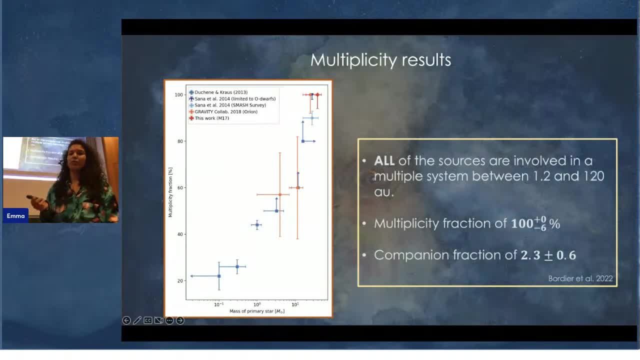 So all of them were found in a multiple system. So we can say that there is a 100% of multiplicity fraction. And if we account for the other companions that are found in HHR, if you remember the spectroscopic companions- 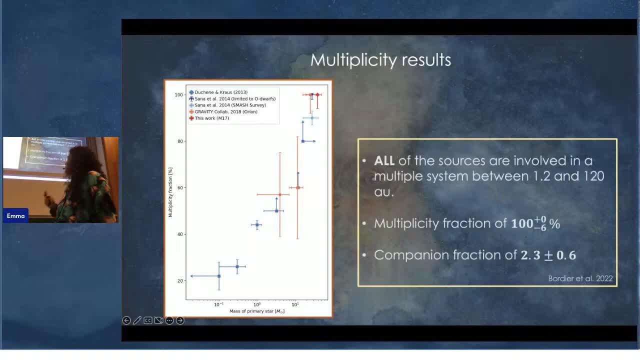 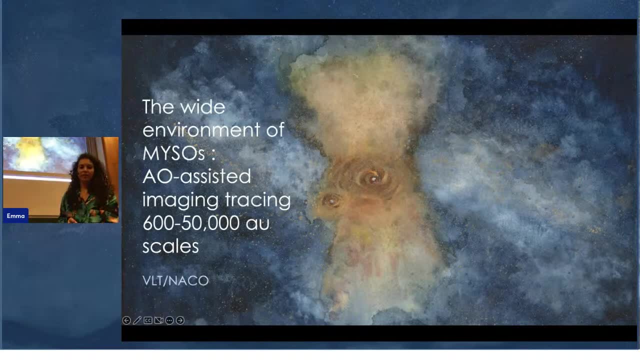 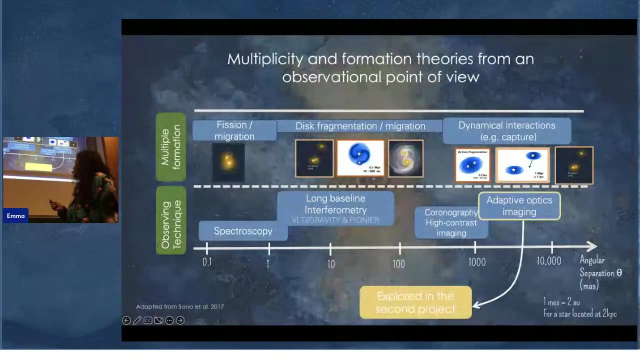 then we go to a companion fraction greater than We went a bit further in the investigation and tried to understand whether this multiplicity extends at younger stages and wider separations. So if I come back to this diagram here, we explored this range of separations, basically up to 128,. 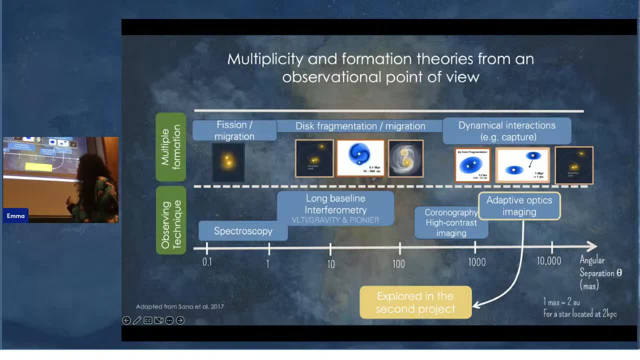 and now we want to see if we also see components at wider separations, And if we do so, then we might have hints of one of these star forming areas. So this is what was explored in the second project. So this time we make use of just one telescope, a single-dish telescope. 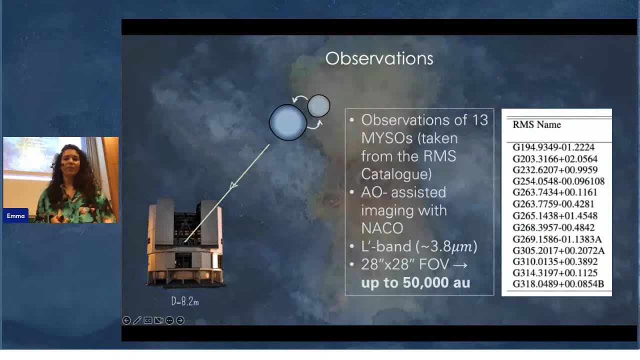 but which is assisted by adaptive optics. So when passing through the atmosphere, the wavefront that comes from the objects is a bit distorted because of turbulence, And there is a technique called adaptive optics that consists of a series of analysis and in real-time tests. 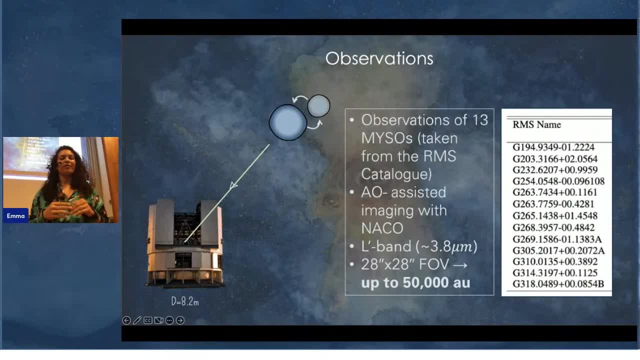 to make, also in real-time corrections, And this is done by basically moving or changing slightly the surface plane of the mirror so that you will be correct for the distorted wavefront. So this image that was maybe looking blurry at first, it now really is neater and closer to the frame of the telescope. 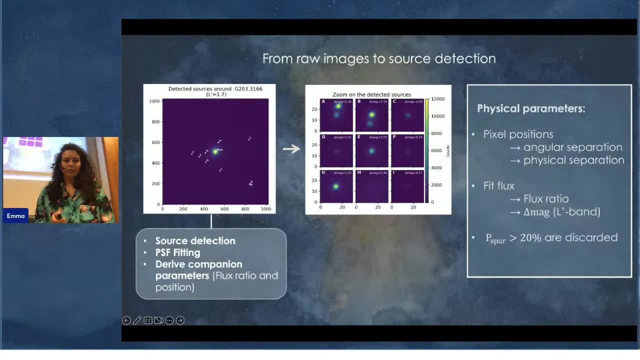 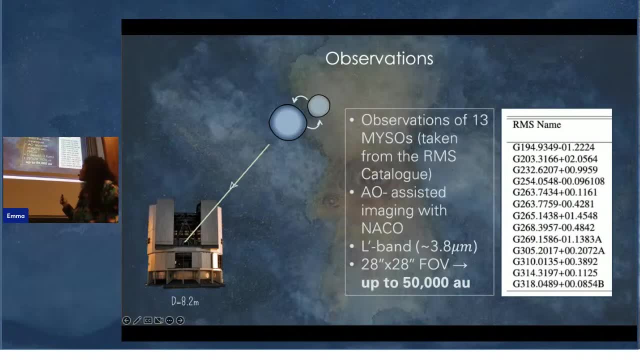 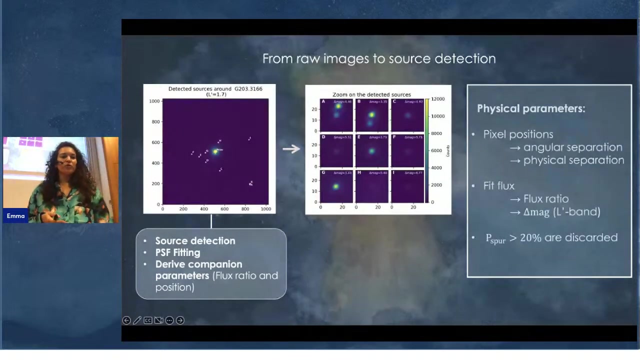 So we obtain- Sorry, I think Yeah. So we have now a set of 13 young stars and we are looking for components at 50,000 AD. This is the type of images that we obtain here, So we perform some source detection in all of the images. 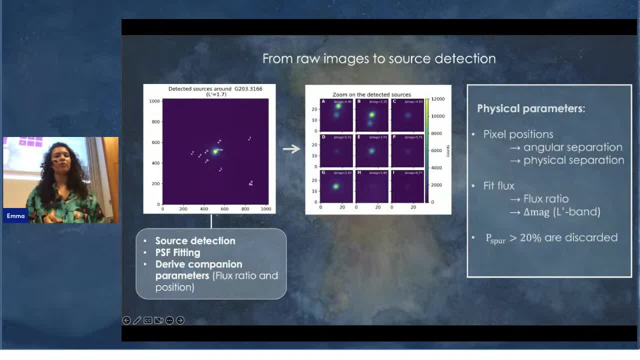 and some PSF fitting to retrieve the physical parameters of the stars which are presented here. So when we have this kind of image we try to spot all the different sources that are plotted here and then we get their flux and also their position. 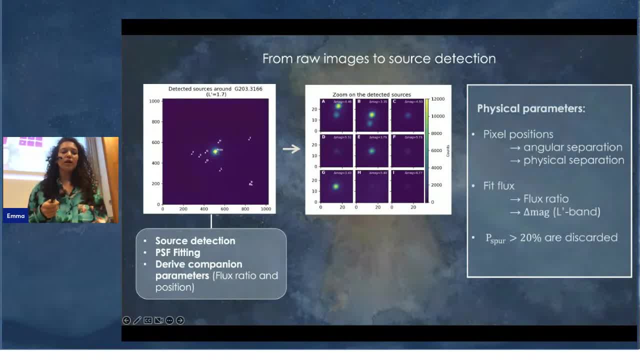 And an important thing that we did as well was to assess whether or not these stars are bound to the central star. here, For example, if I look at my home, which is in the middle of the auditorium, I take a picture. I will have foreground people and background people. 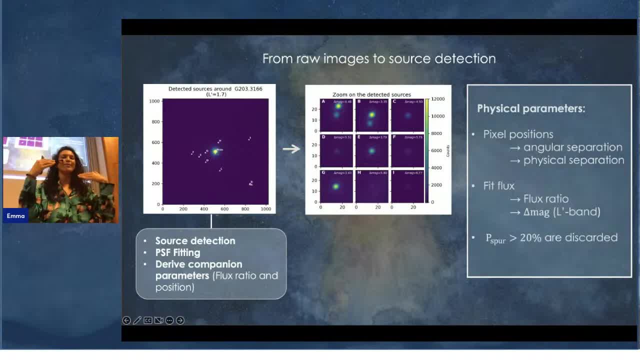 It's the same. when you look at the stars in the sky, You might have a foreground star and also a background star that has nothing to do with the star that you are observing And that are maybe polluting a bit your image. So you are not polluting an image. 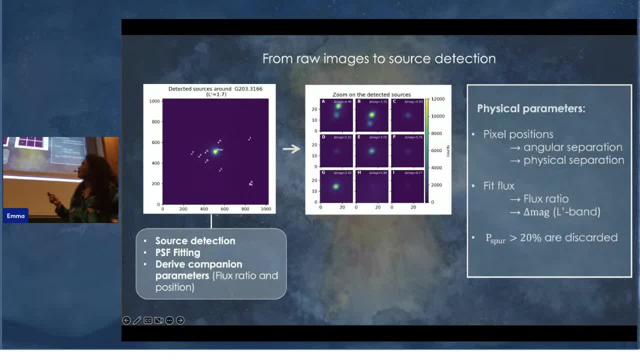 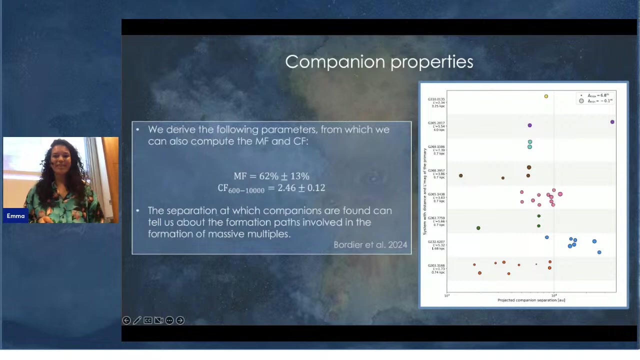 And this is done by some statistical resource, because we cannot really monitor the movement of all these stars- And if they have, like, a probability of being 4 or background source bigger than 20%, then we discarded them. for the rest of the analysis We could also for these 8 sources. 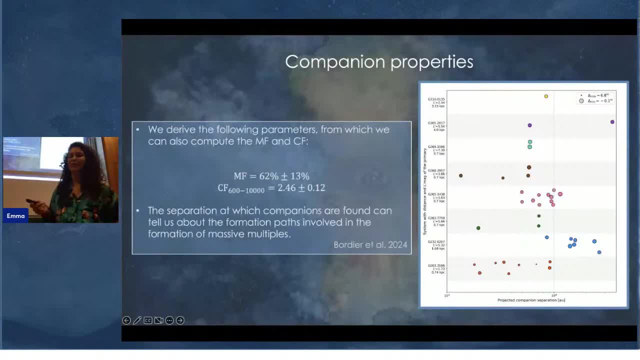 sorry, for these. 13 sources derive a multiplicity fraction, So only 8 of them appear to be in a multiple system. So it is still 62% of multiplicity And the companion fraction is also greater than 2.. 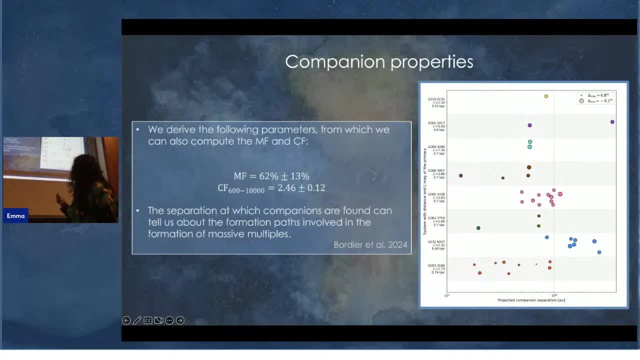 Here I display we can see how. what is the distribution, the separation distribution of the companions for each system And the separation at which companions are found can tell us about the formation path involved in the formation of massive multiples And the two previous projects. 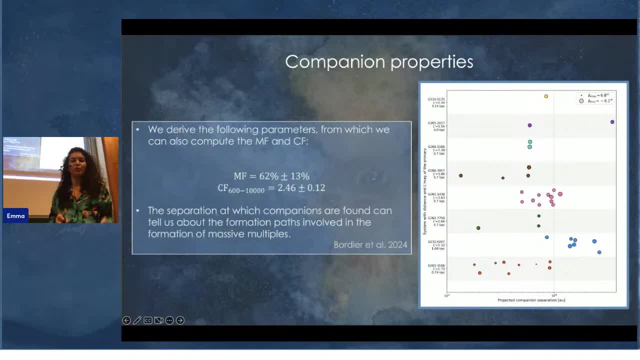 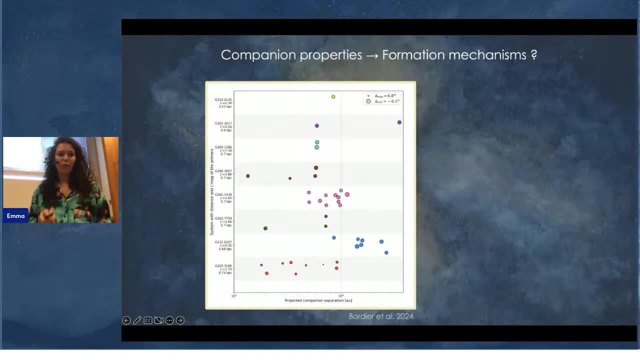 that I just presented already provide these valuable observational trends. So okay, So from all these properties, we can speculate as of the formation history. However, we have to keep in mind that the successful theory for multiple formation must both reproduce the observed multiplicity statistics. 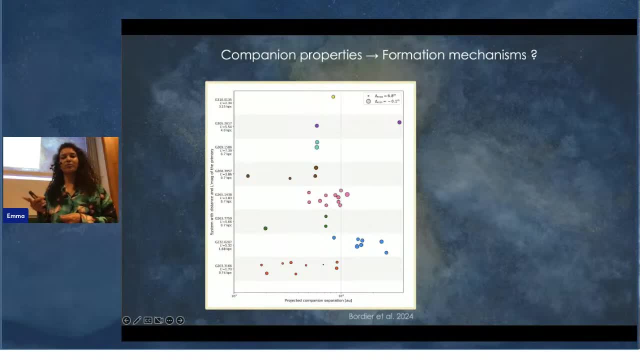 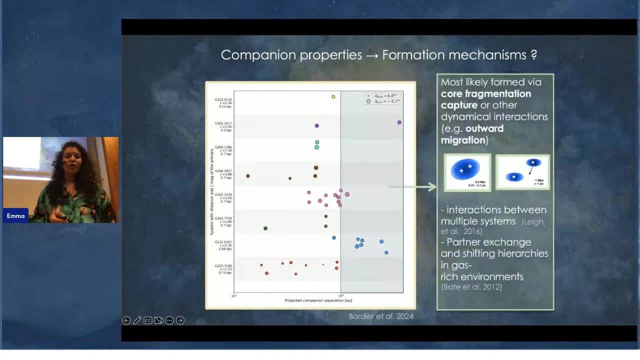 so the one that we see here, but can also be able to reproduce and model young and individual sources and how we form them. So, for example, if we look at at the, the wider, wider, sorry separations here. 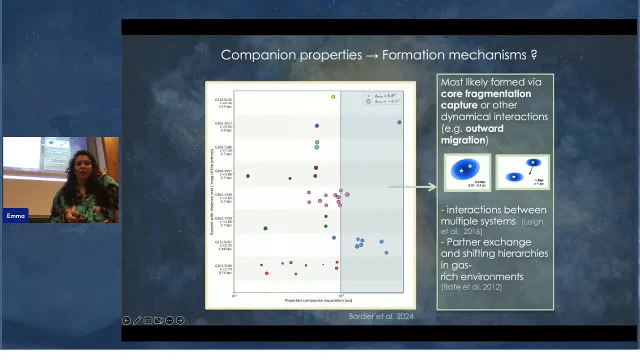 it is most likely that these stars have formed through co-fragmentation or or any other dynamical interaction, just given, like the, the, the parameters. So it might be in different multiple systems. It might also be some partner exchange. 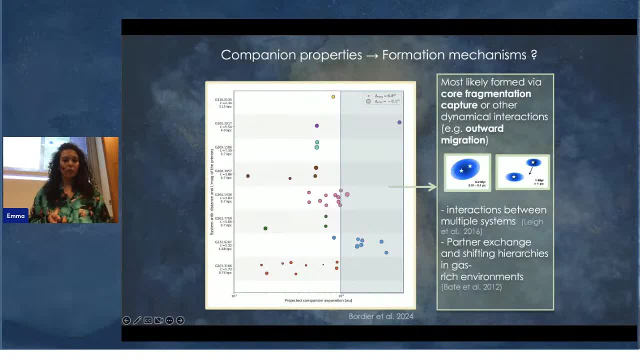 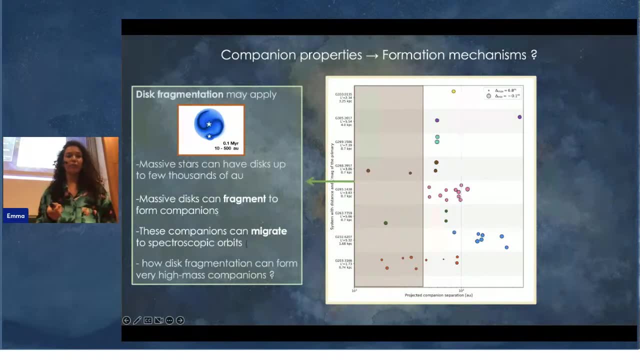 that shifted the hierarchies. If we look now at closer separations, this might this compiler might have formed through disk fragmentation. It is one of the channels that can apply, because we know that massive stars can have up to a few thousands of astronomical units. 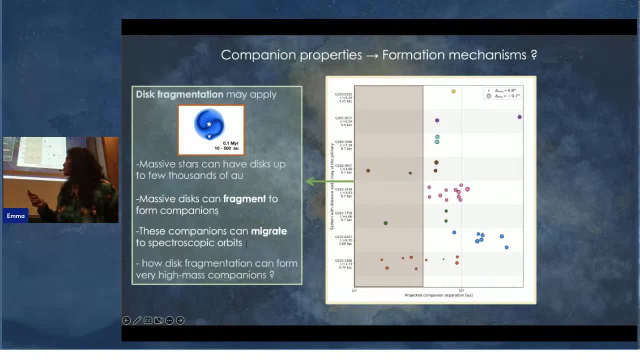 And these companions can migrate to spectroscopic orbits. I will come back to this later. still for this channel, We can still question ourselves that how fragmentation can form very high mass components. For the previous project it was conducted with gravity, So we look at even closer. 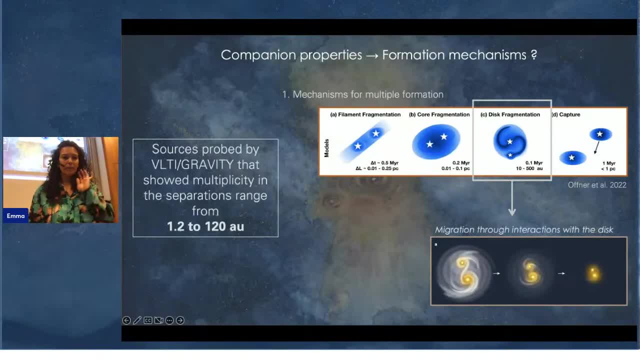 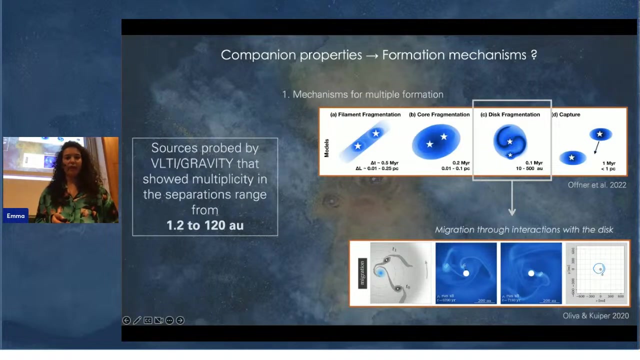 closer separations And for this, disk fragmentation. if you look at the processes of fragmentation, disk fragmentation could be a very good fraction of such components. This has been tested also through simulations by teams And they found that we can actually form close components. 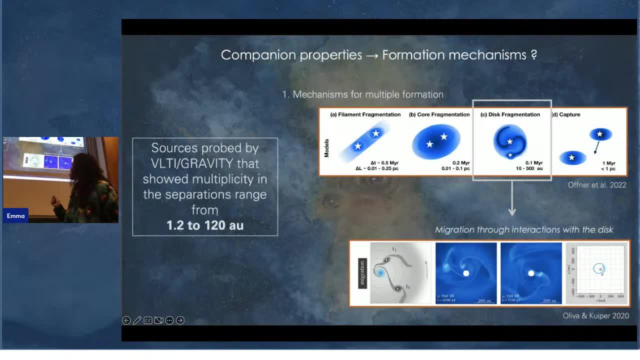 through this formation channel, So we might form components in the disk. At first they are just fragments And then, as they migrate, they also gain mass, And if they are not destroyed by any destruction process then they can become close components. 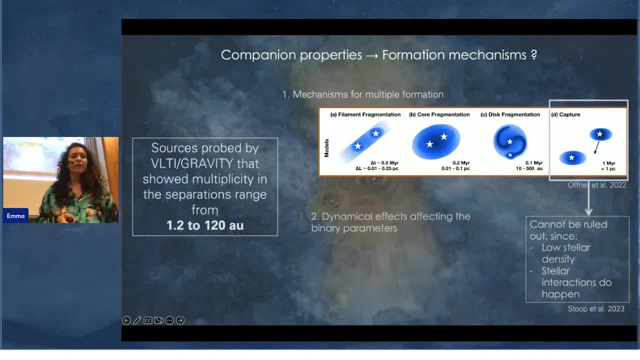 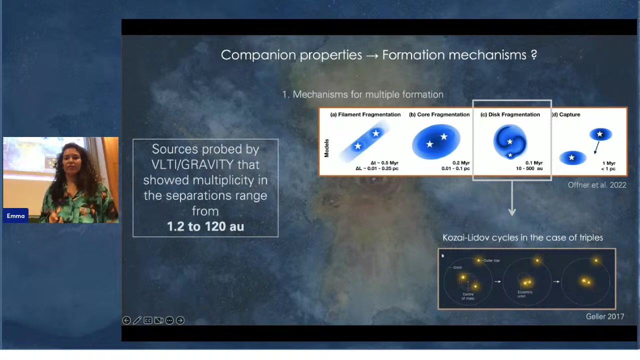 And, finally, we can completely rule out capture, because now we know that it also happens in low-sterile density environments And that in this kind of environment, such as N17, sterile interactions do happen, And also in the framework of forming these components. 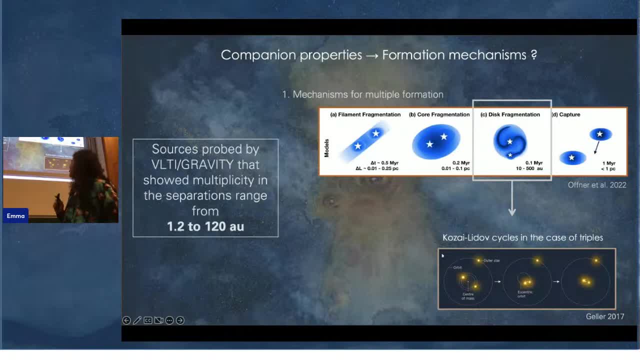 I don't know why there is this word here, so sorry. There are also other mechanisms, called quasi-read-off cycle in the case of triples, because we have seen that we have more than two components on average. So it means that there is like: 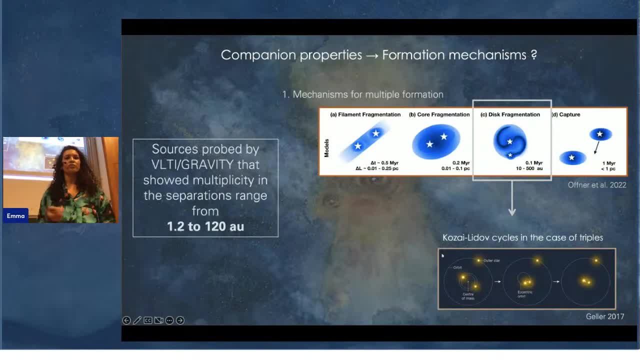 a third component involved in these systems and can, of course, influence the formation of close components. And one last thing that we are missing in this puzzle is the influence of a close of a tertiary companion, And this leads us to the third project. 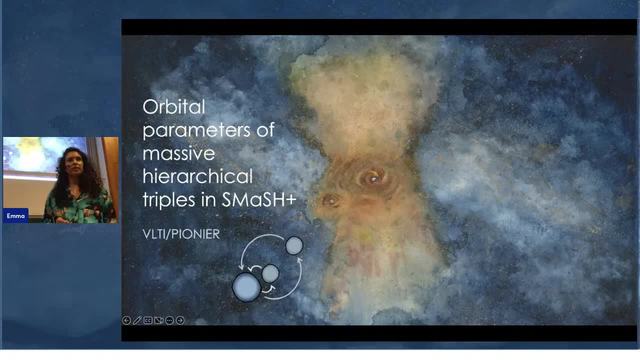 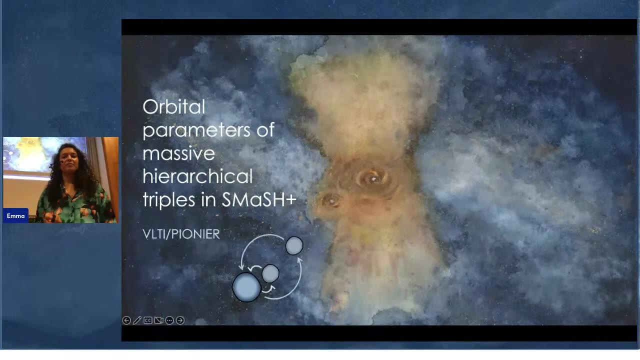 we conducted, which aims at studying triple systems, And this was motivated also by the fact that in both projects we have a companion fraction that is richer than two. So triples systems are more common than we initially thought, And for this project we worked. 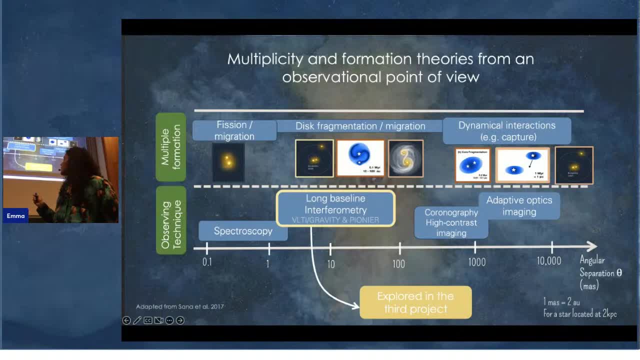 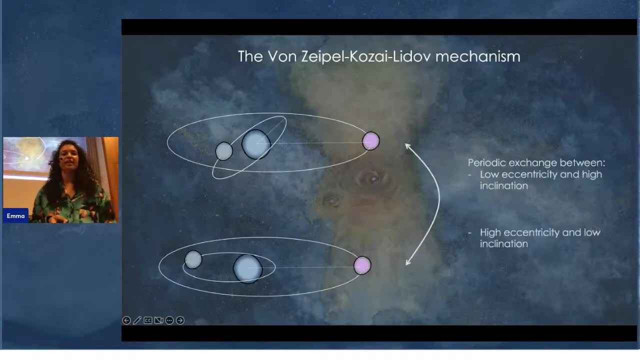 with a team of three, and we will also use again longer Cool. So, in short, in a triple system, that is say hierarchical, which is stable, a tight binary is orbited by a third companion, and they are usually 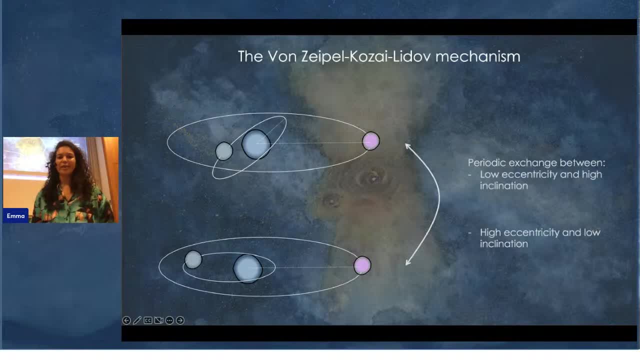 in a rather stable relationship, such that they don't merge or there is no one of the companion components that is ejected And in this stable situation dynamical effects can happen. So this is like an orbital phenomenon that was developed to explain the orbits. 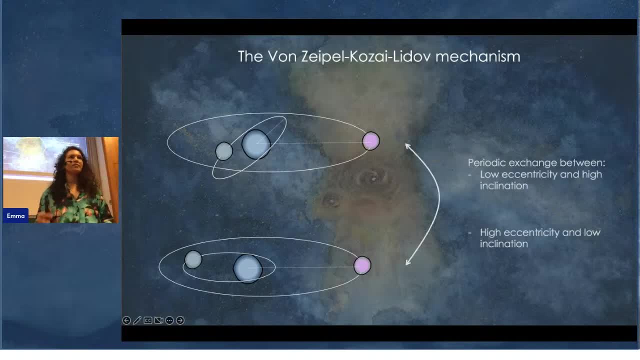 of certain planetary satellites by Lidov and Cosi in the 60s. So the Cosi-Lidov mechanism comes into play when we have at least three components, three sorry bodies in the system. So you have two bodies. 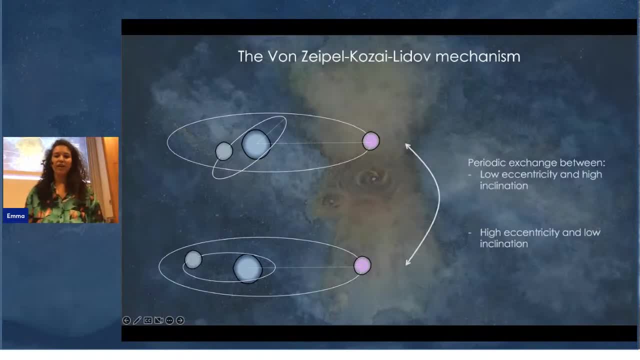 that orbit each other. here in the two situations and under certain conditions, the perturbation from the distant object can change the shape of the two main object orbits here, such that you will have a period exchange or oscillations between low stages of low eccentricity. 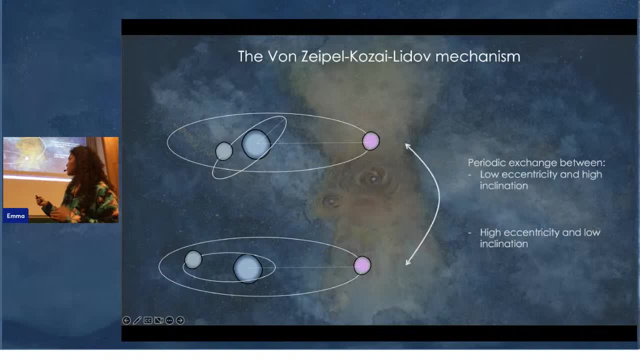 and high oscillation, or you have an external orbit that almost aligns with the plane of the third orbit. yeah, the third orbit, the outer orbit, sorry, The system will be considered stable if the period of the outer companion here is at least. 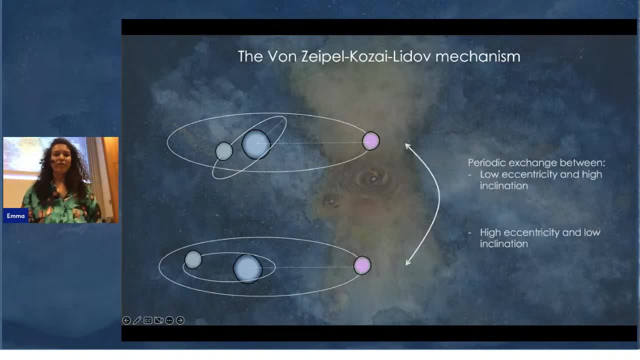 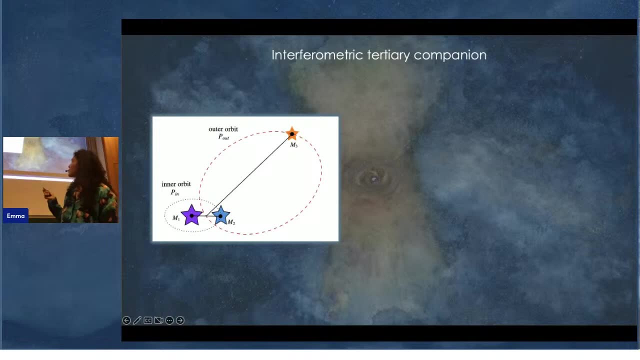 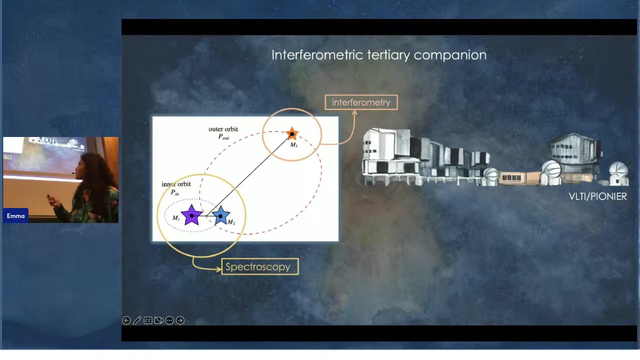 five times the period of the inner companion here. Good. So in this situation you have an outer- sorry, an inner system that is usually detected by spectroscopy because it's a very tight binary, And you have an outer companion that is detected. 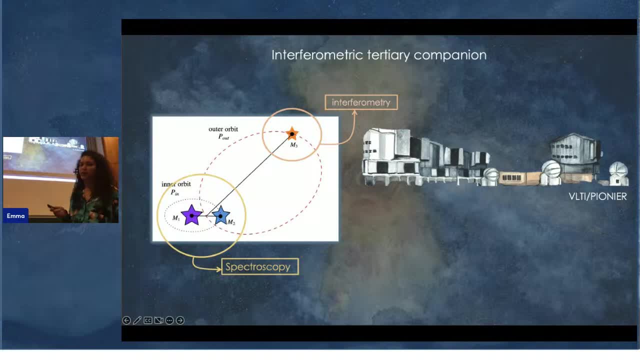 by because the situation here is really bad. So there was like a campaign that was conducted with VLTI to try to like detect the outer companion, And so in the sample, in the data set, we have 21 massive hierarchical 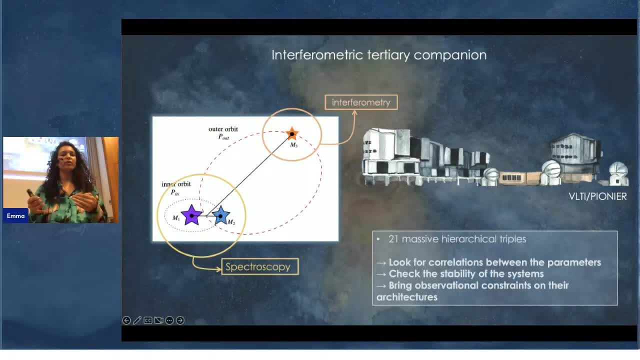 triples And we look for correlations between the parameters such as, like the mass of the outer companion, the separation of the inner binary, the separation of the outer binary. So this is the theoretical criteria of stability And we also bring observational 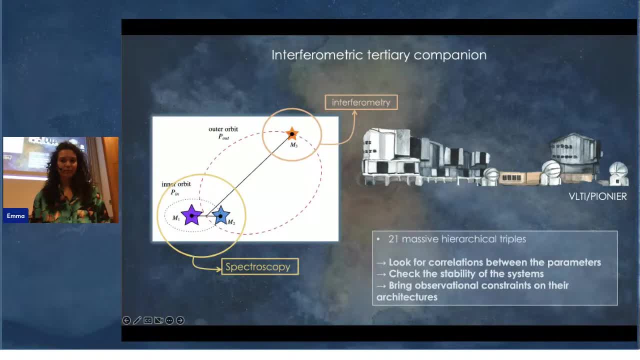 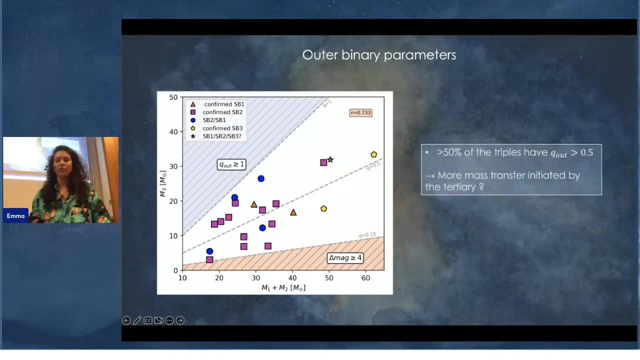 constraints on the architecture. Okay. So, for example, we find that more than half of mass ratio. so between the outer companion and the inner binary, we find that the inner binary is more stable than the outer companion. So the inner 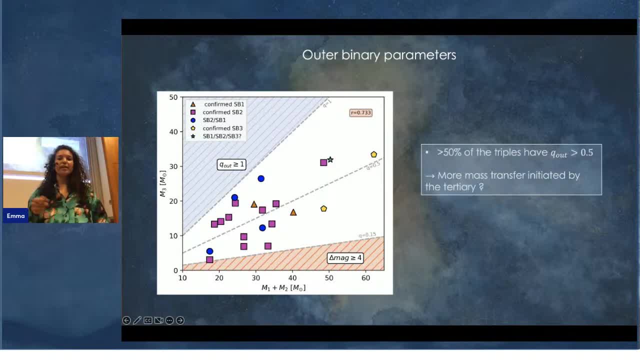 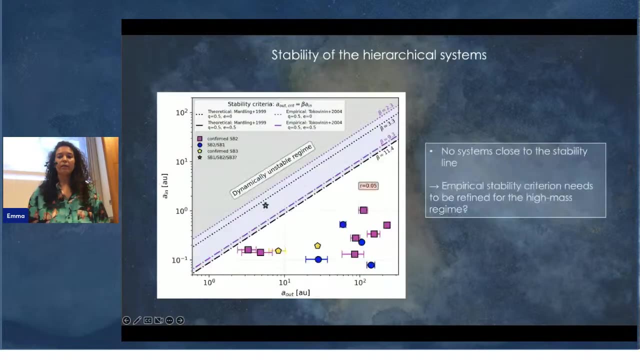 binary is more stable than the outer companion, So the inner binary is more stable than the outer companion. We also looked at then the stability of the hierarchical systems, And for this we used theoretical criteria. So this equation that I haven't 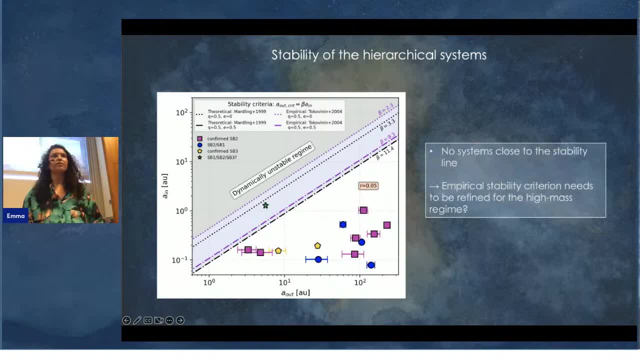 seen here, but it would- And this equation mainly shows that most systems are close to the stability line, which tends to show that this criteria- could We have a star here- that falls into the instability wall, but we still have doubts about this. 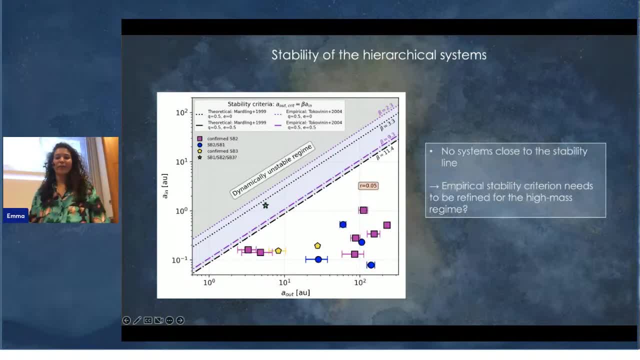 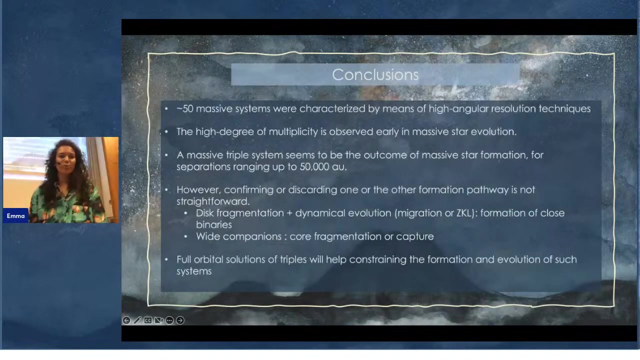 So this project is still ongoing and we aim at deriving the solutions that we don't have to make assumptions on, the, Which is something that we did here, And we also have some other points for the full orbit of the outer companion, and we 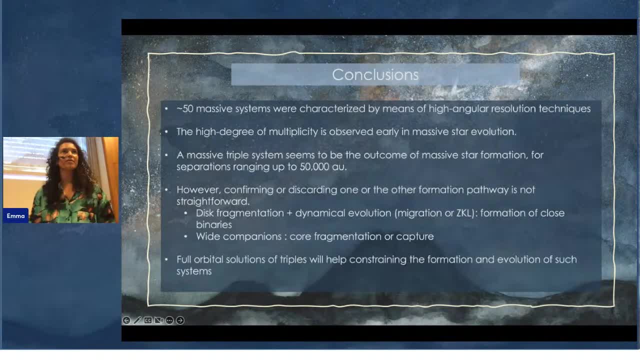 could eventually reproduce. So okay, In conclusion. so we studied more than 50 massive systems during the last two years And we also found that there are two or more, And we confirm against the high degree of multiplicity at young stages of. 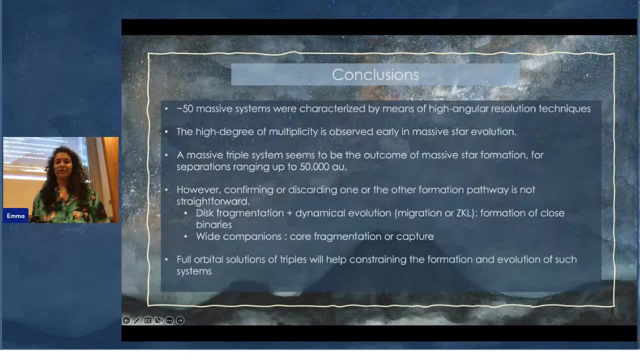 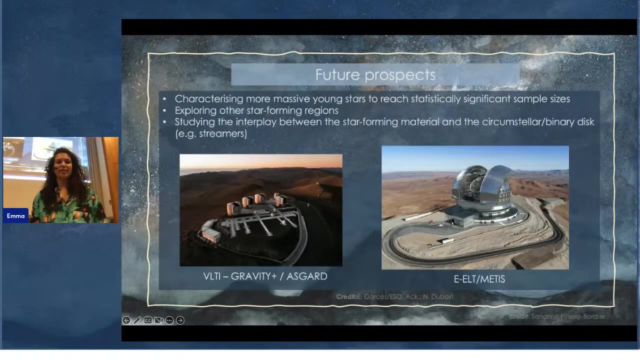 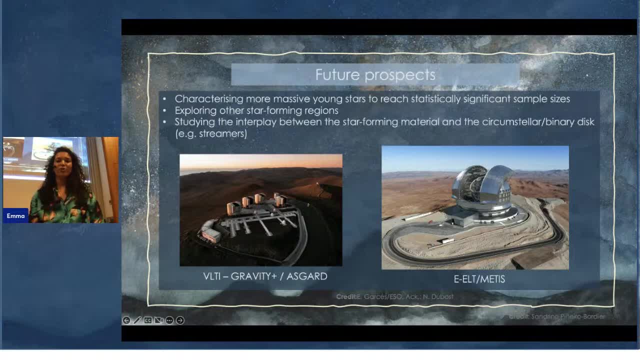 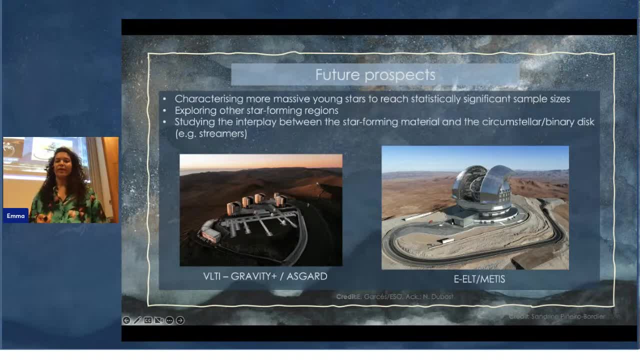 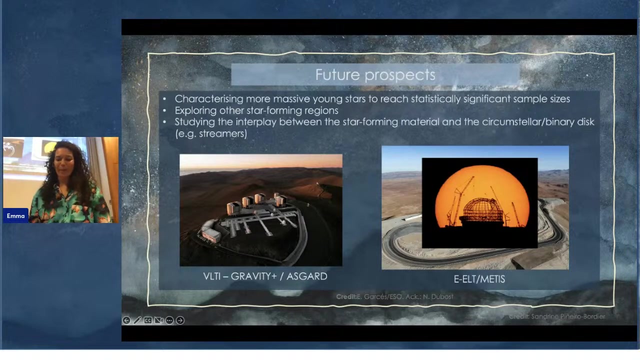 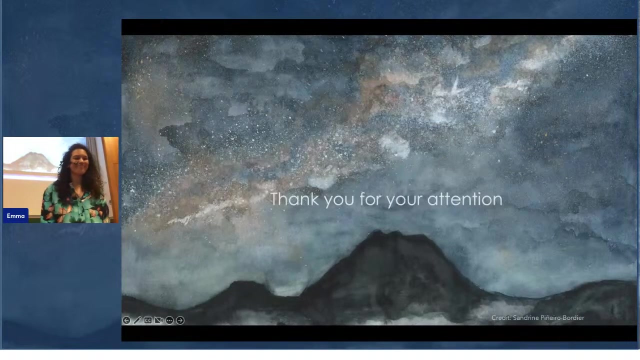 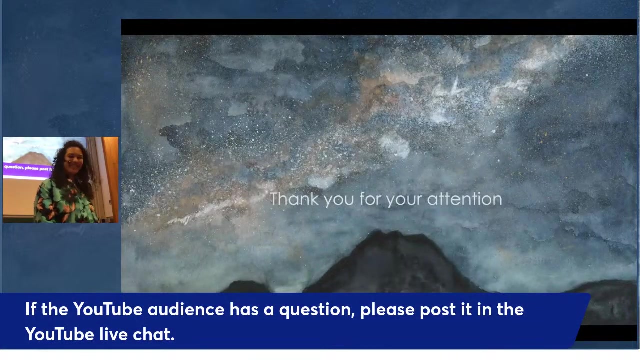 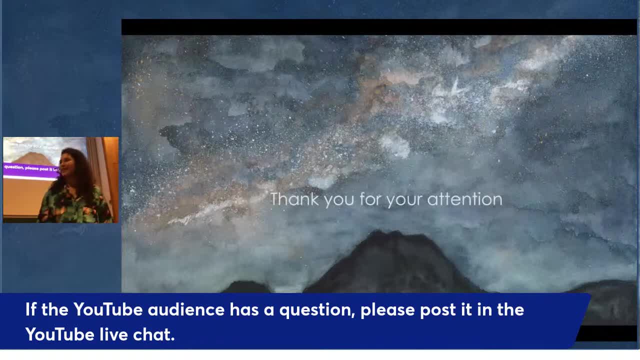 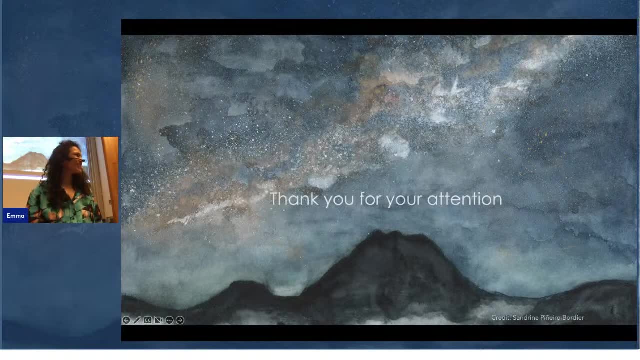 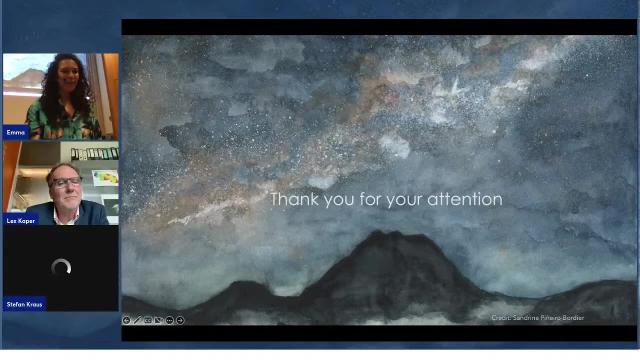 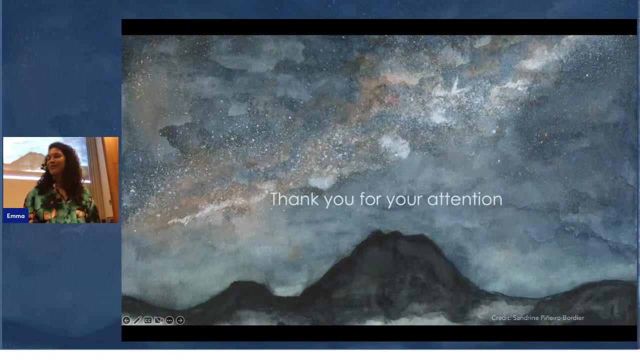 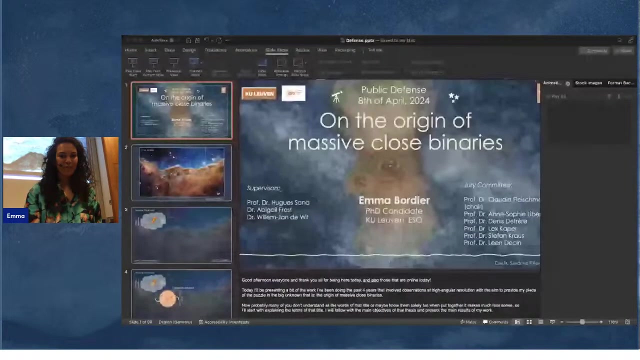 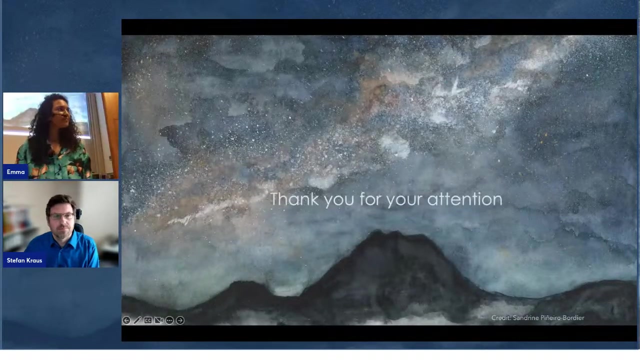 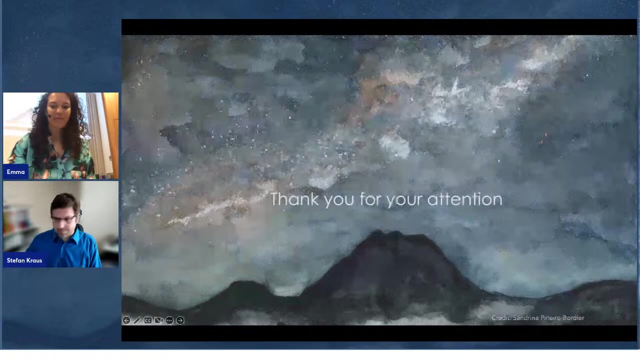 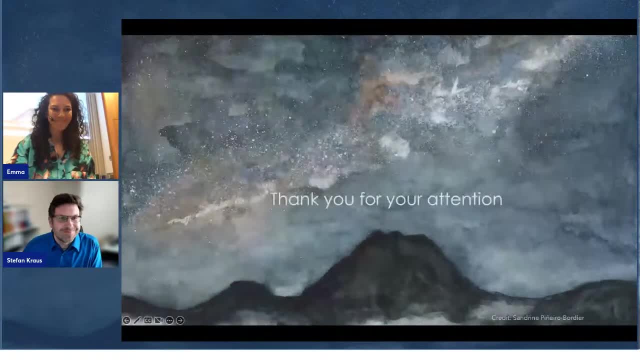 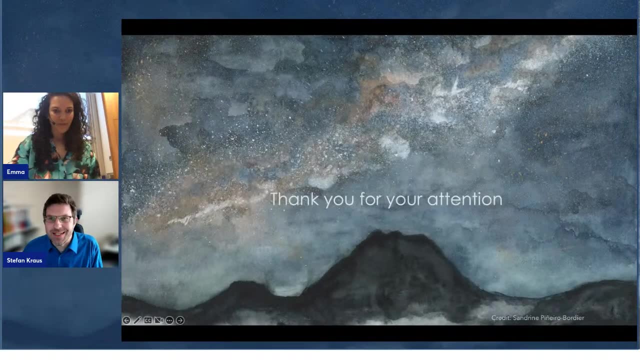 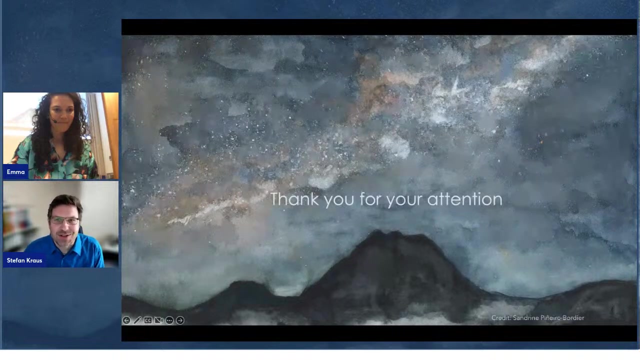 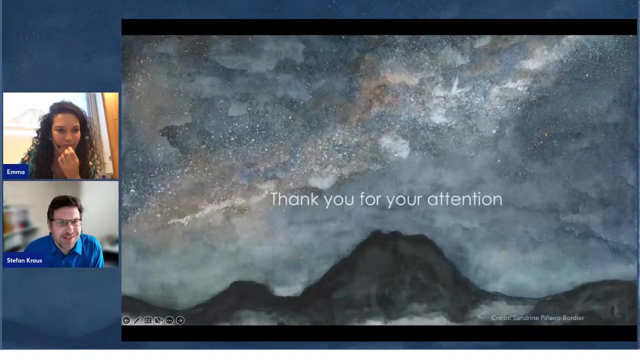 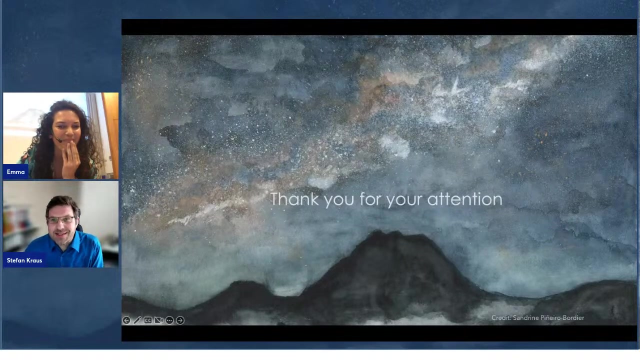 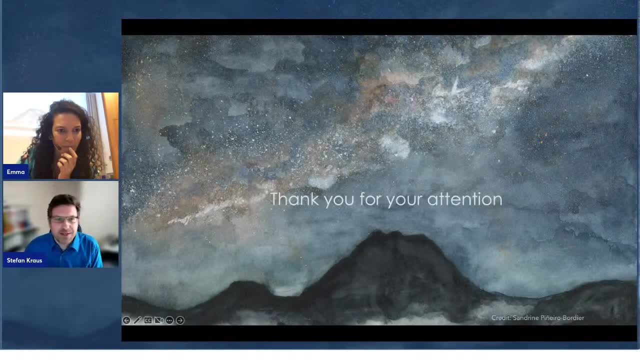 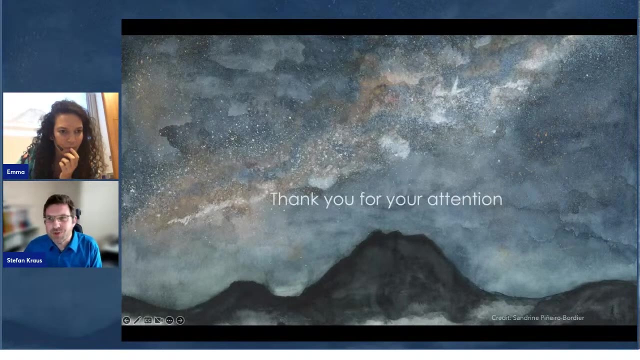 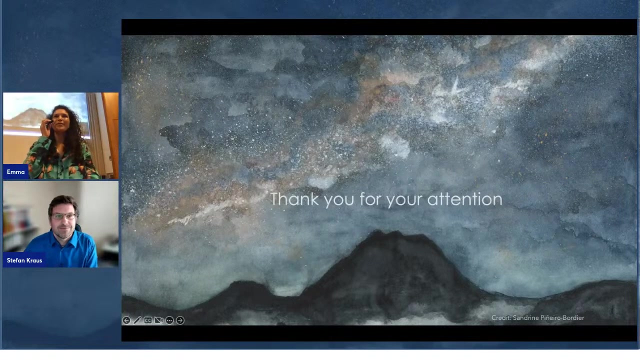 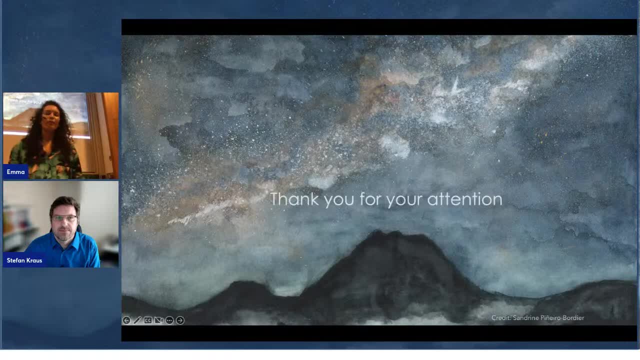 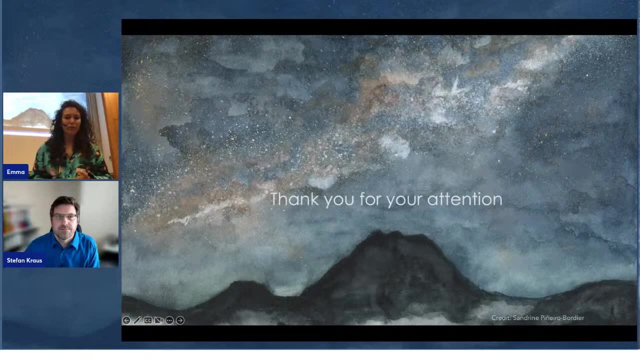 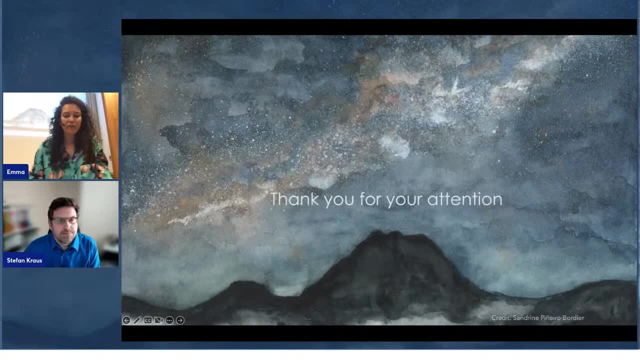 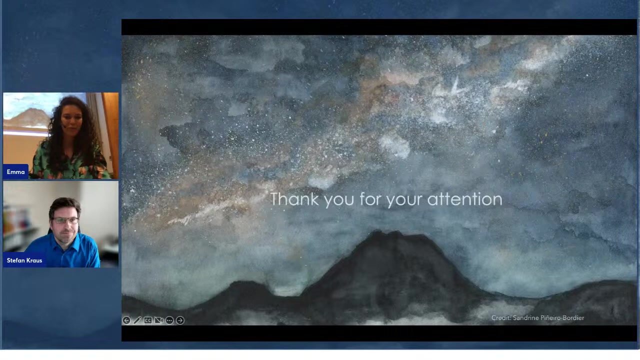 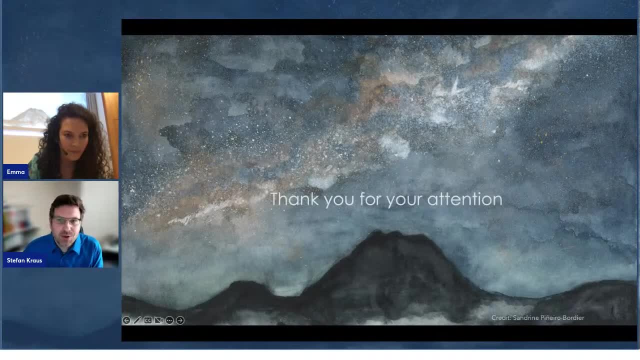 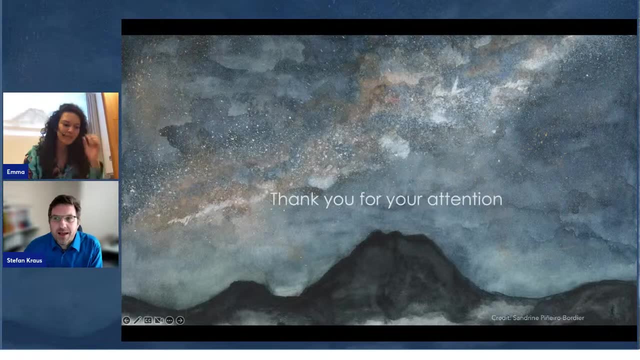 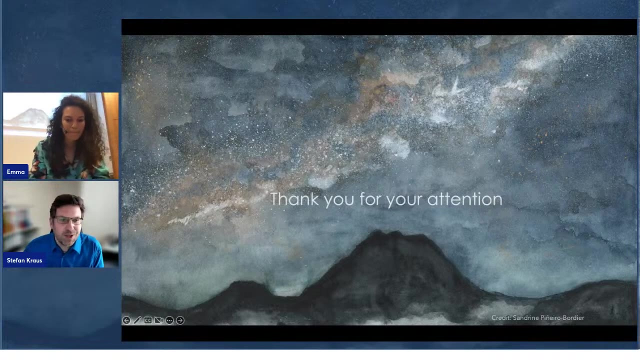 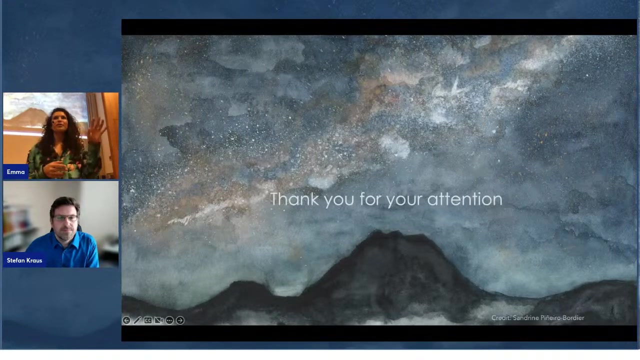 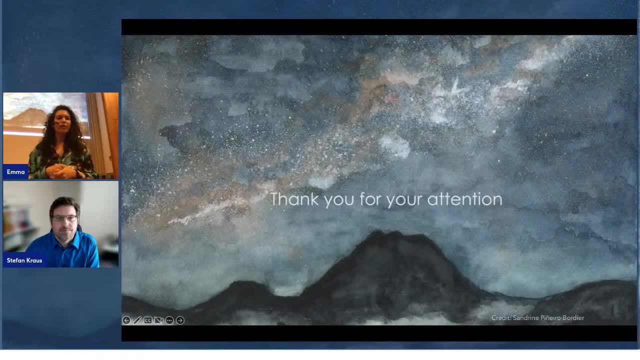 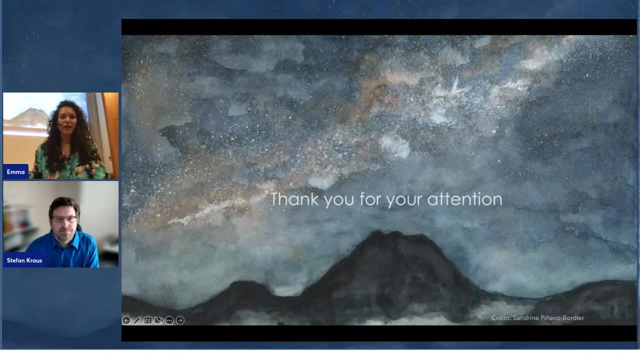 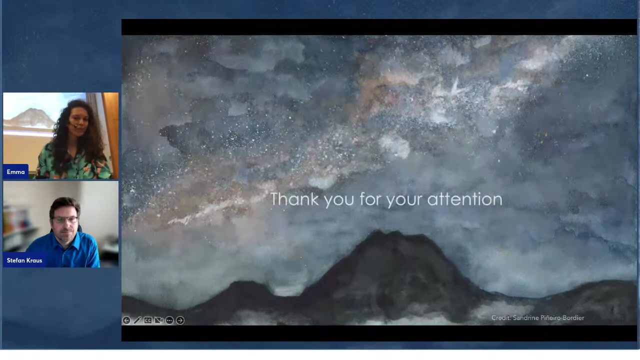 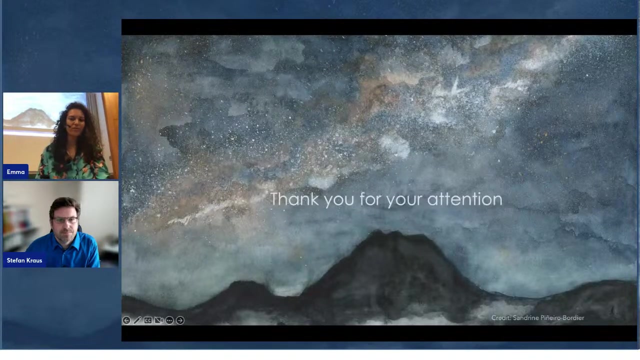 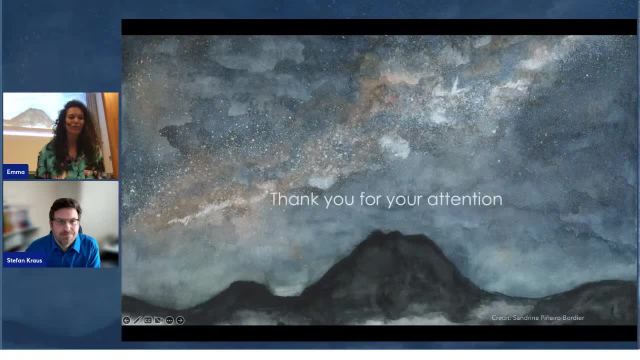 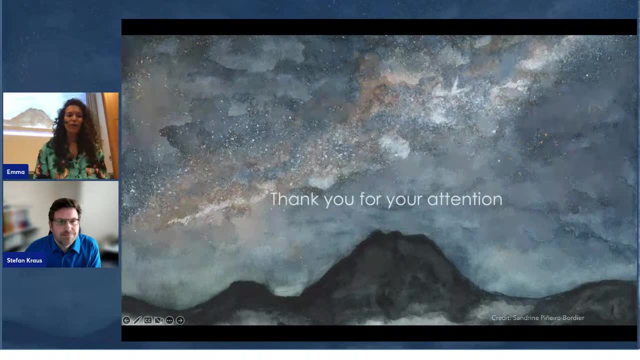 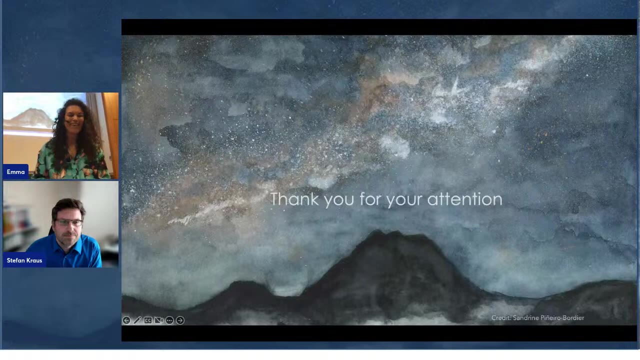 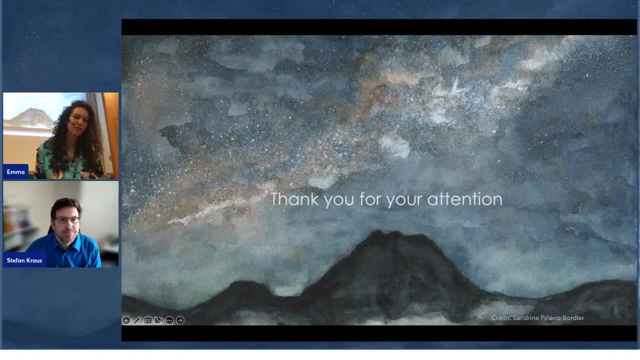 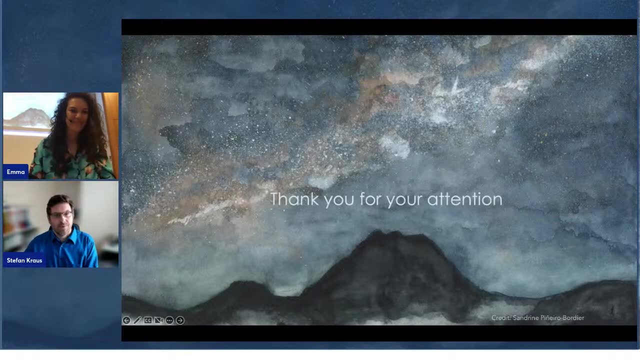 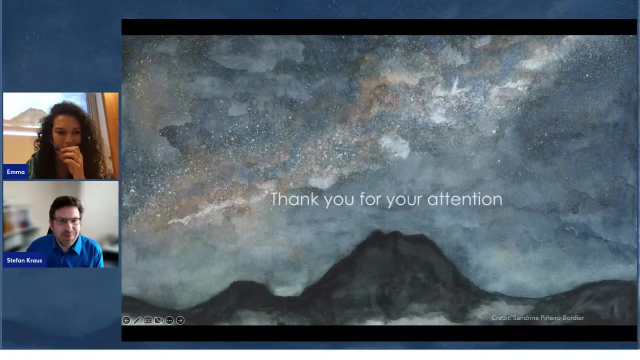 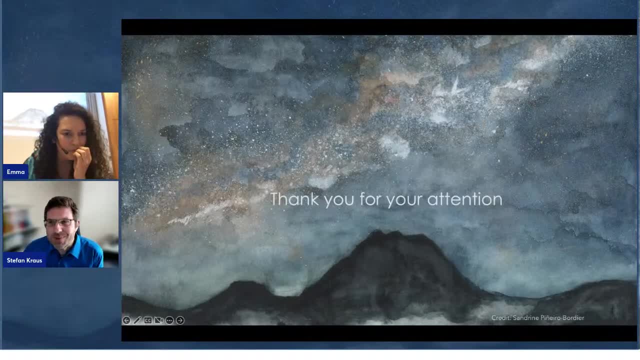 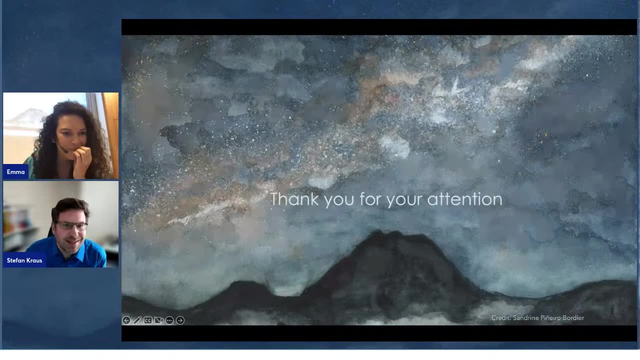 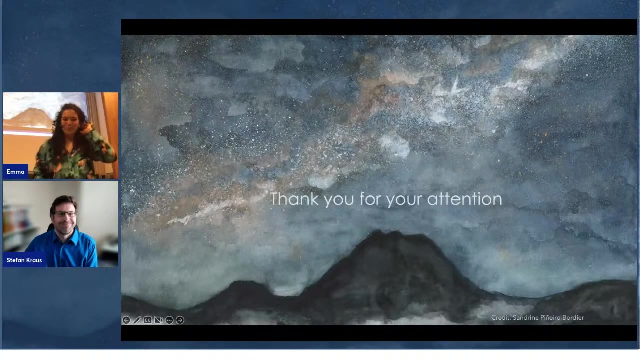 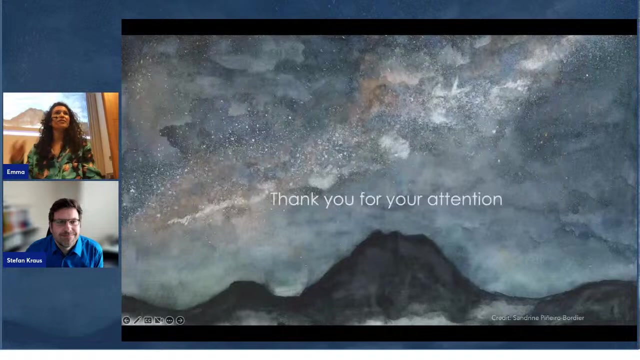 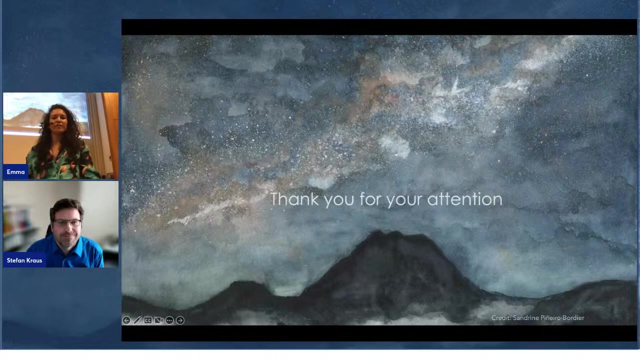 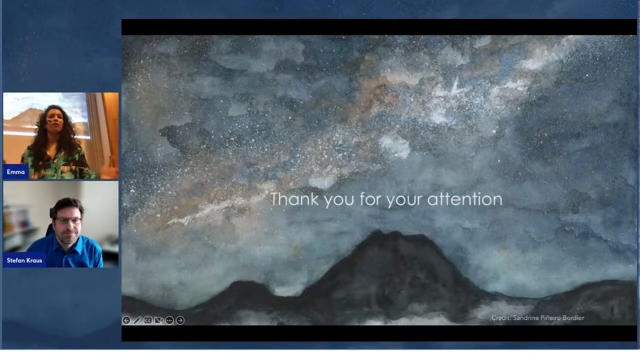 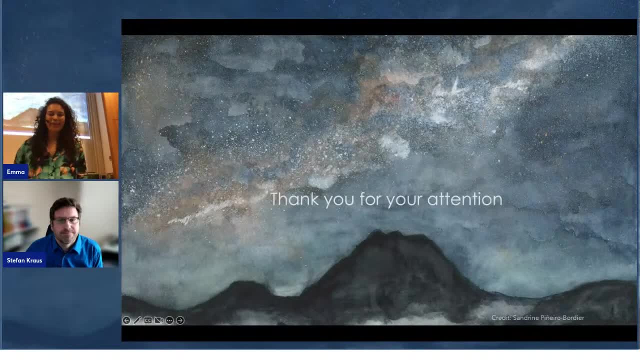 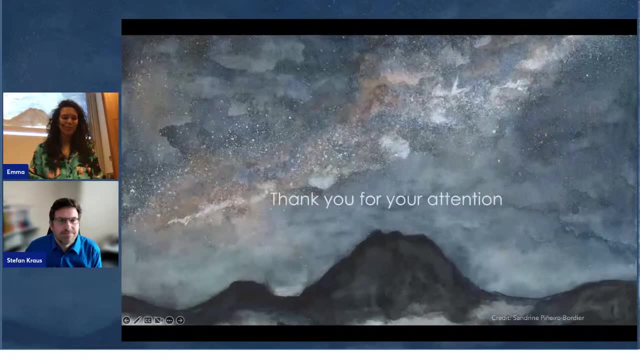 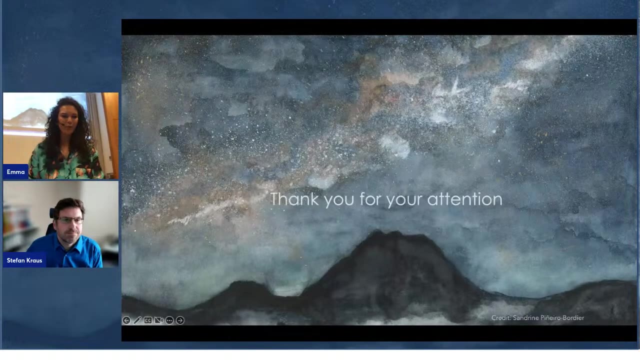 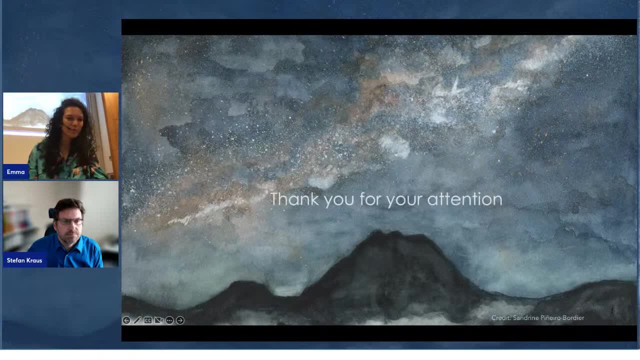 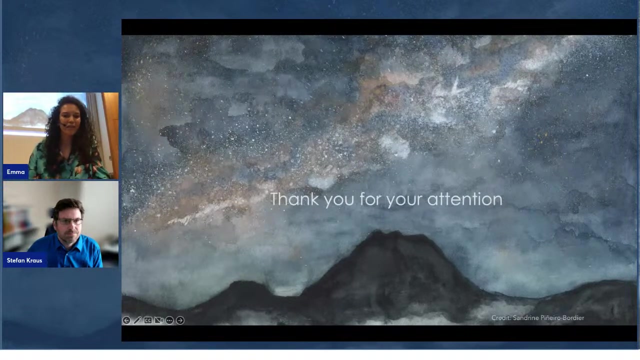 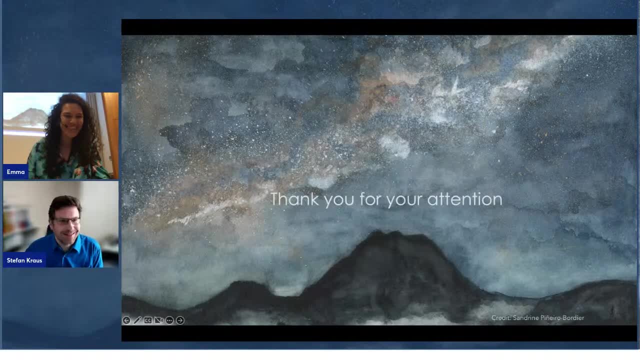 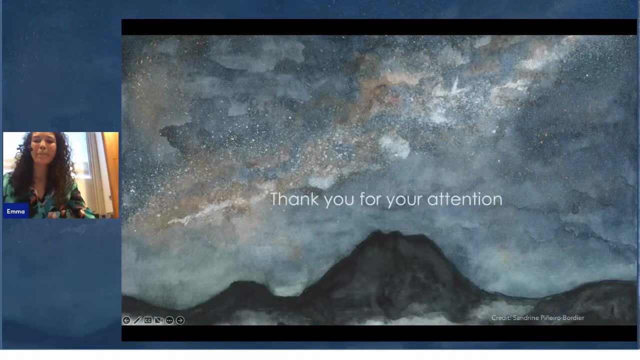 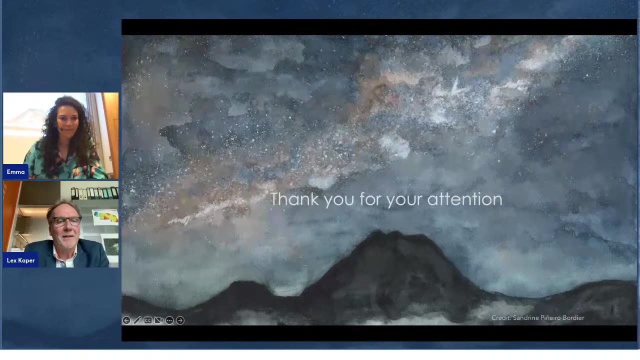 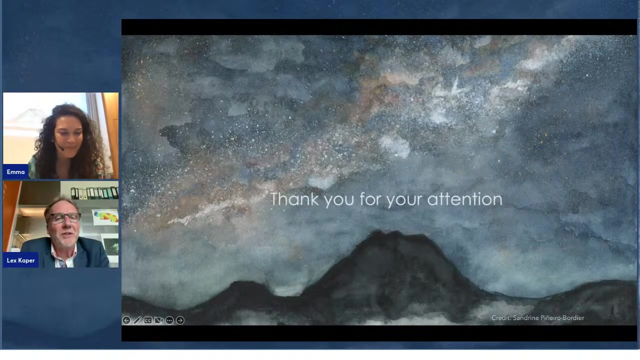 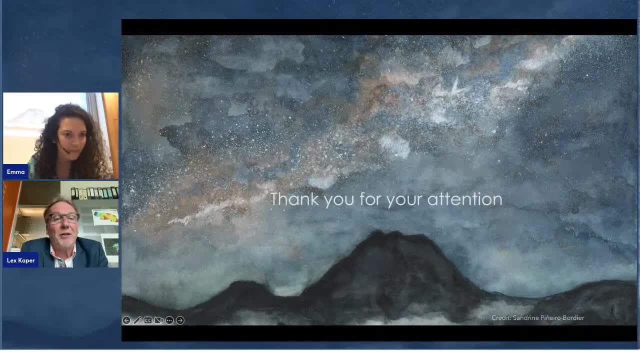 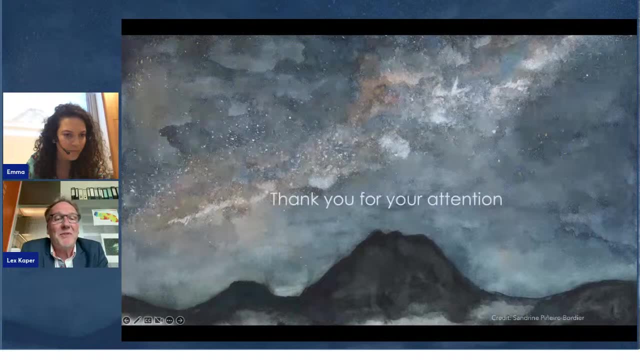 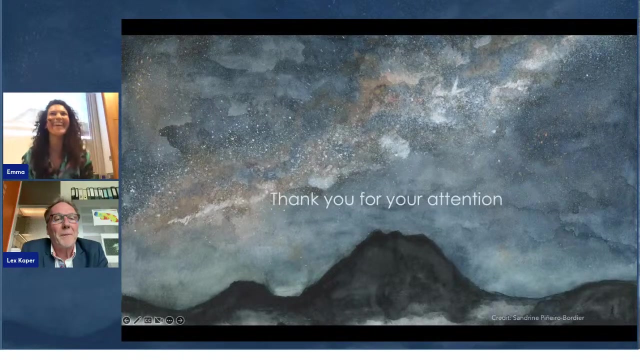 And it is actually quite difficult to form stars, especially massive stars, And Adriaan Blauw, a professor that you may have heard of from the Netherlands, almost half a century ago said that there is a very large number of young stars in 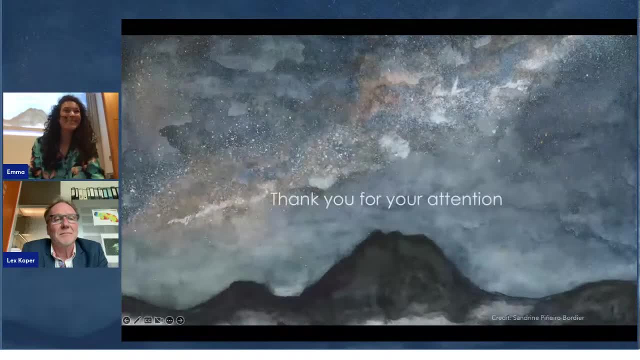 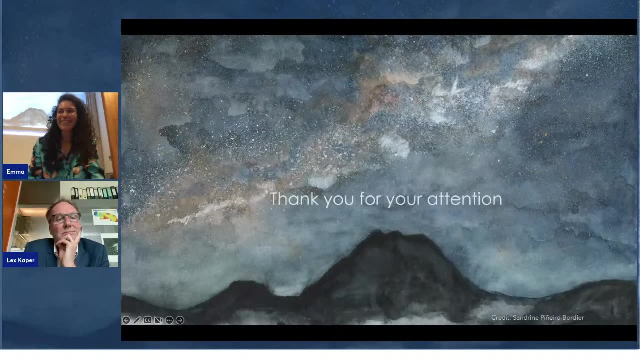 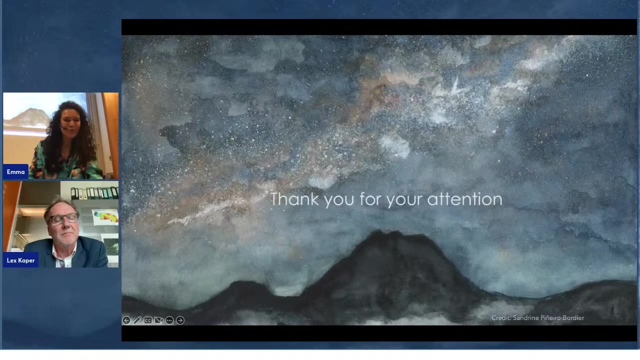 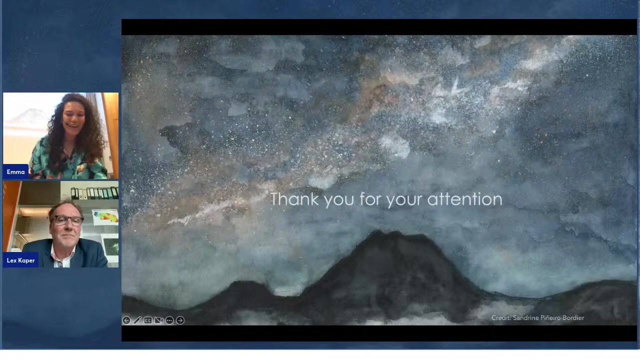 the outer companion And we also found that there is a very large number of young stars in the outer companion And there is a very large number of young stars in the outer companion And there is a very large number of young stars in the outer. 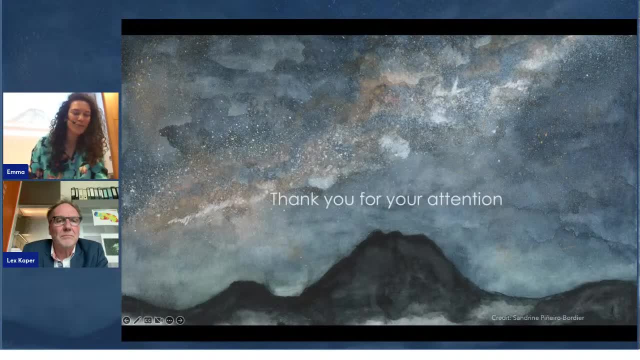 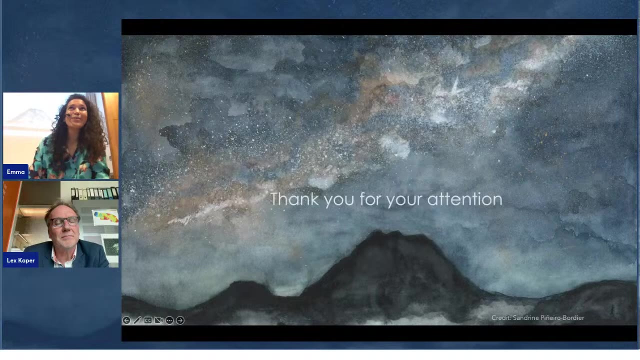 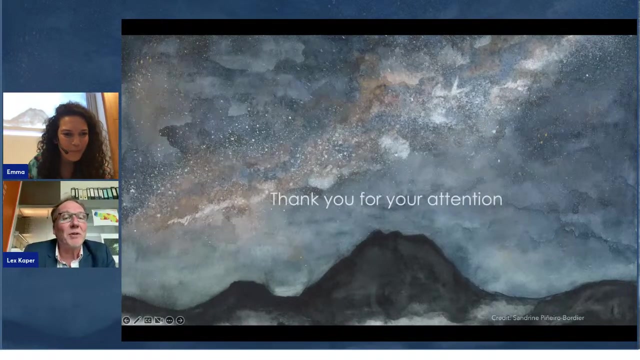 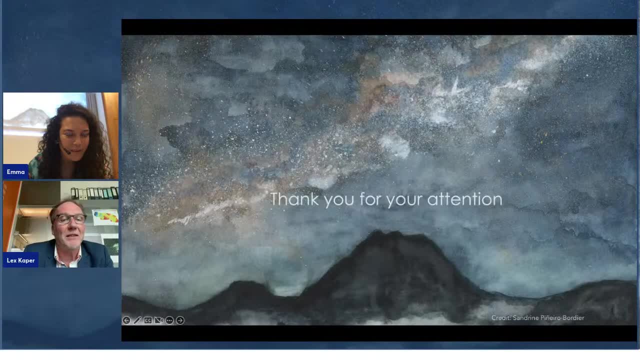 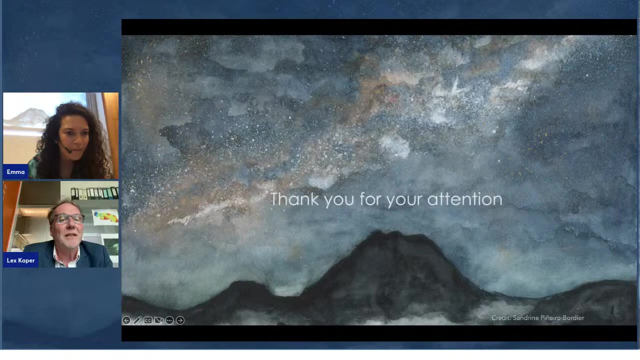 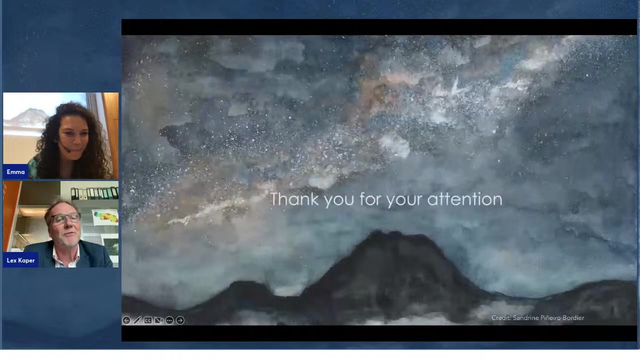 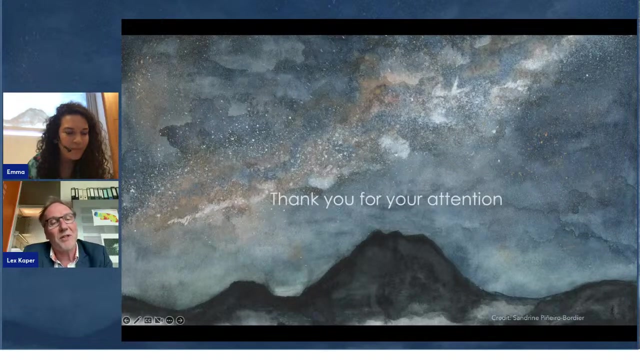 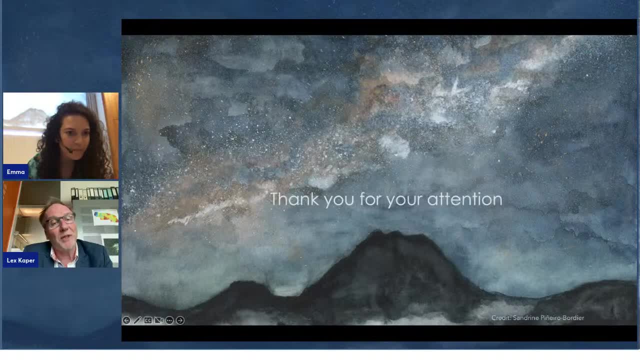 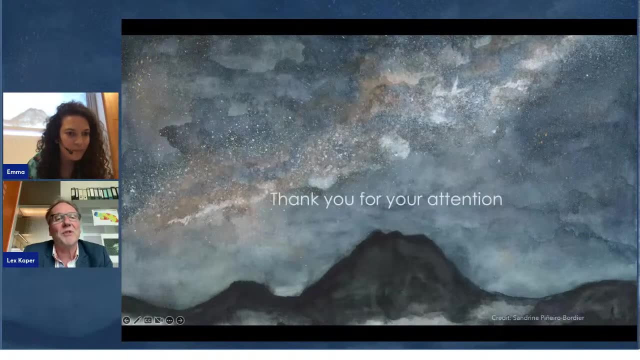 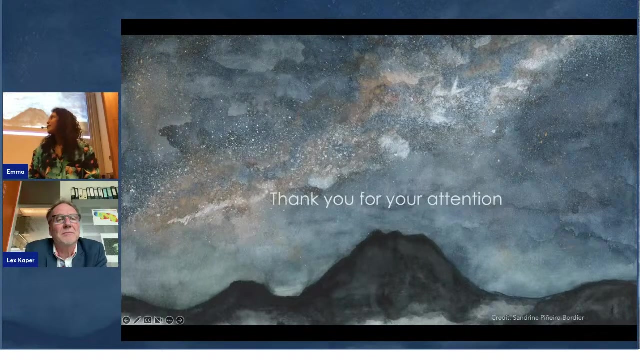 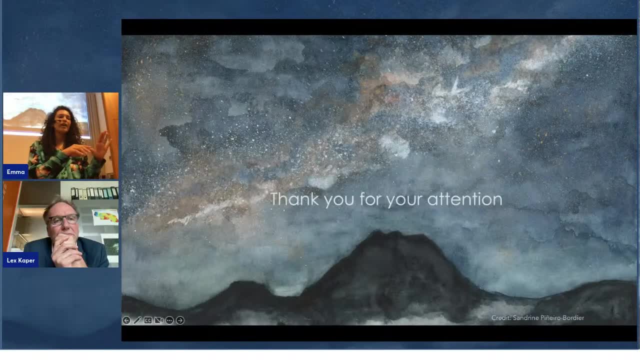 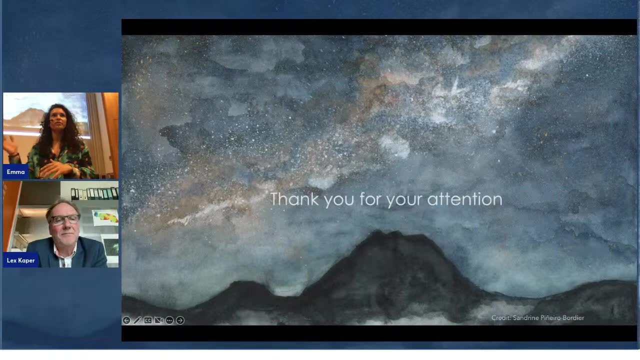 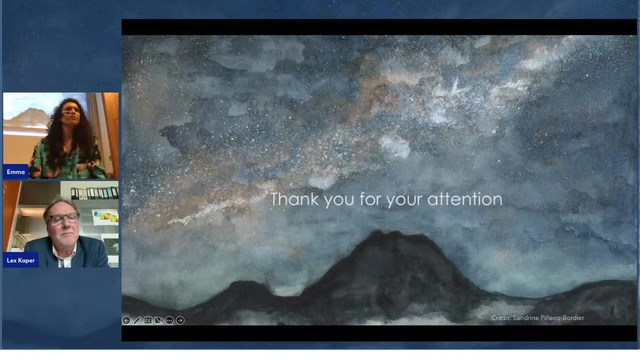 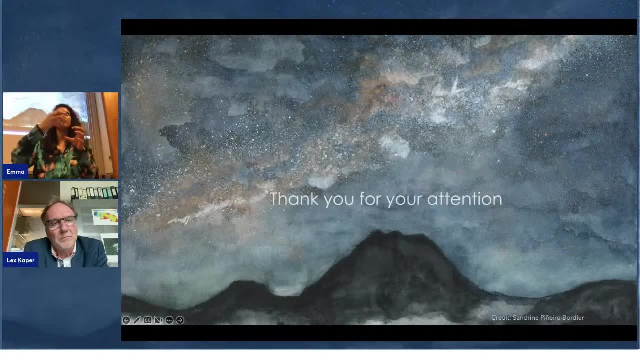 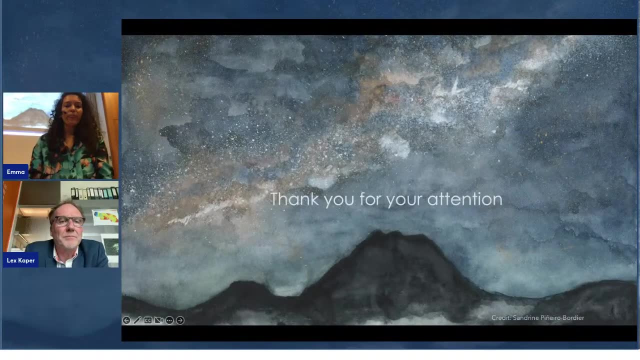 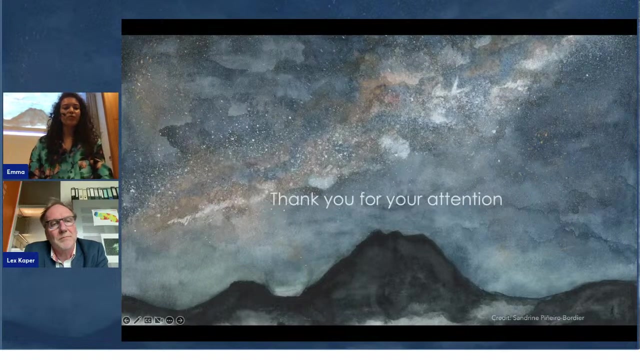 of young stars in the outer companion towards the central star, so that you have a tight system. And Professor asks what I think about this and if I can prove or disprove what she wrote in her paper. So this is a very large number. 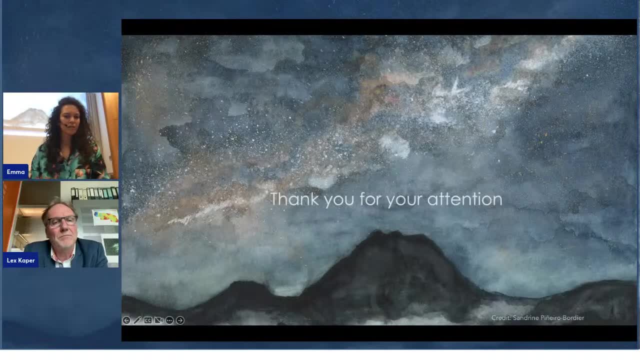 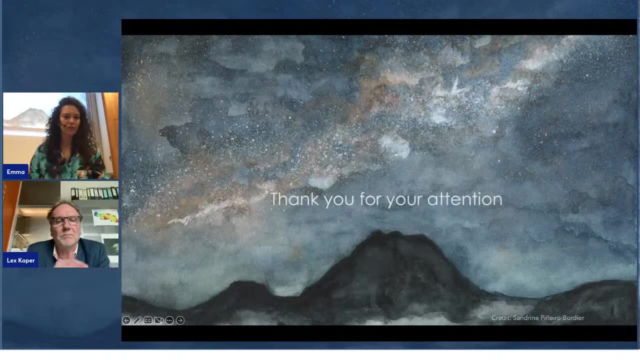 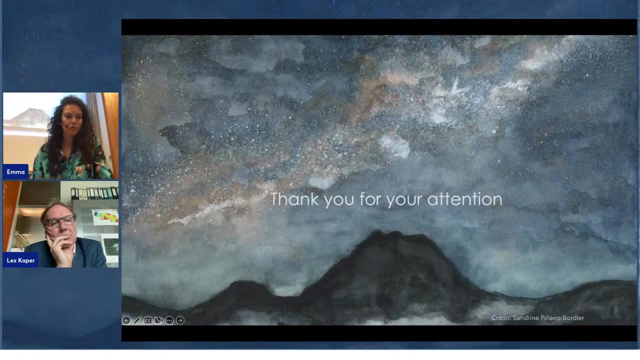 of stars in the outer companion And there is a very large number of stars in the outer companion And there is a very large number of stars in the outer companion. So this is a very large number of stars in the outer companion. So this: 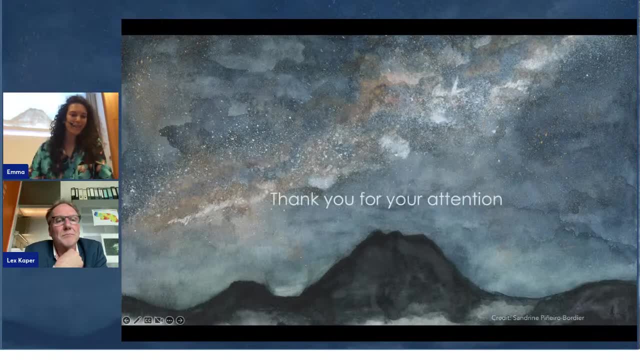 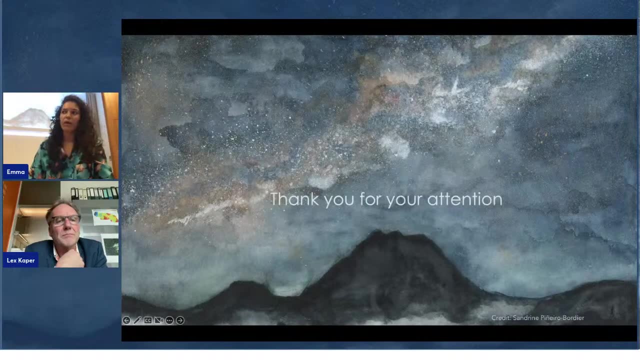 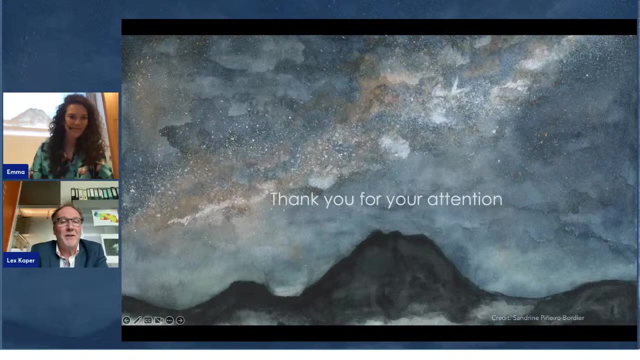 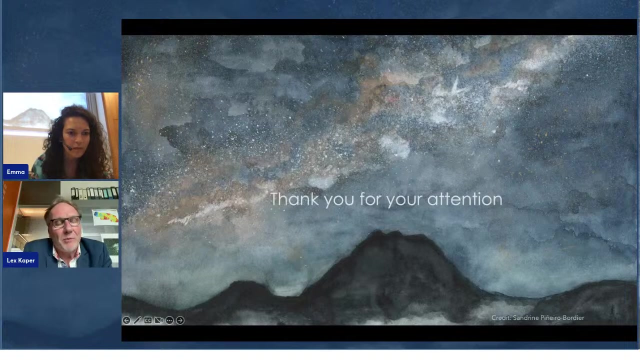 is a very large number of stars in the outer companion, And so, yeah, I would say that in the end, I will respond to that as well. Okay, thank you. And my final point is the most massive stars. I think you also alluded. 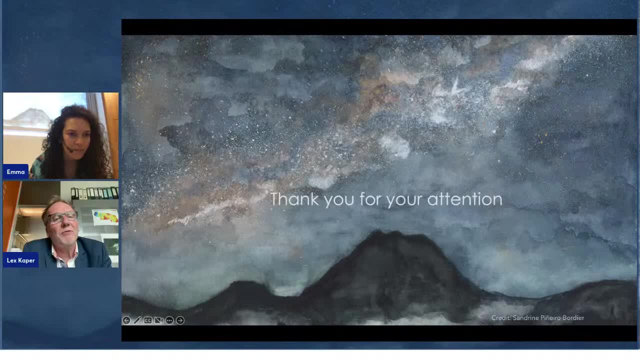 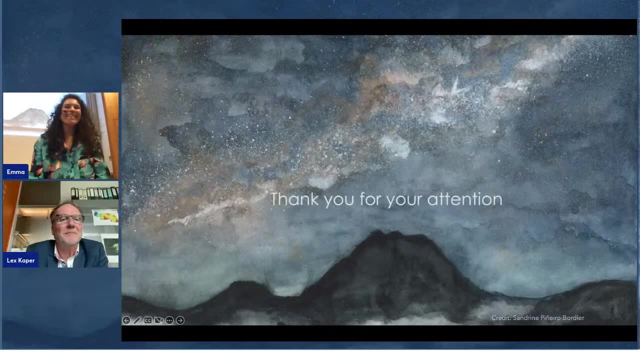 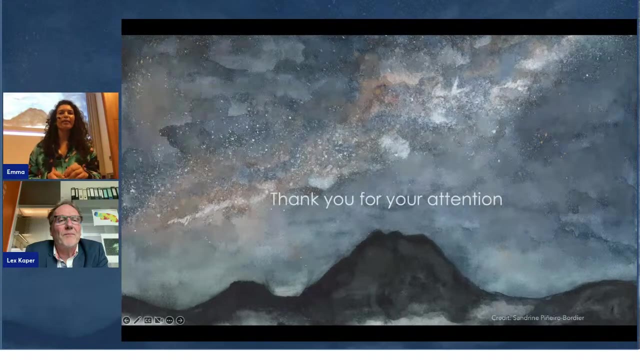 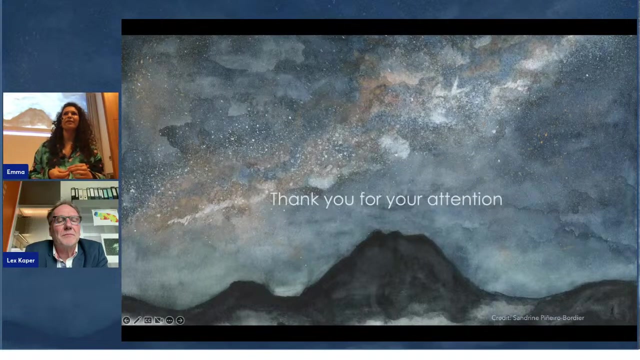 on that. is that actually the way we form the most massive stars? Okay, I will repeat: He said that the most massive stars might have been formed through mergers. So I think what he calls also theories of massive star formation, because we don't know. 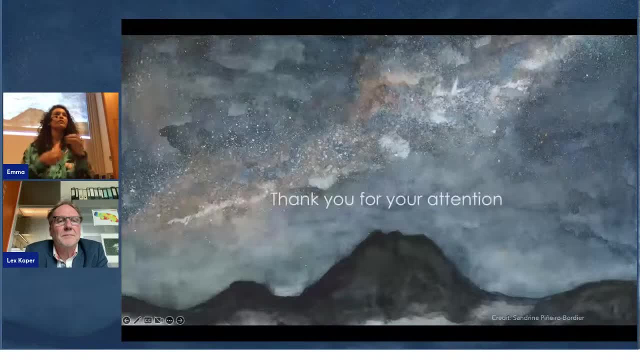 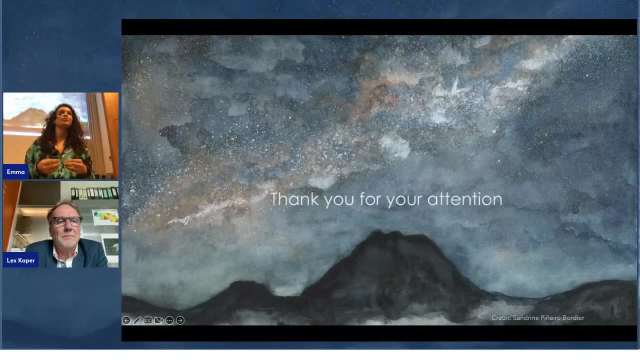 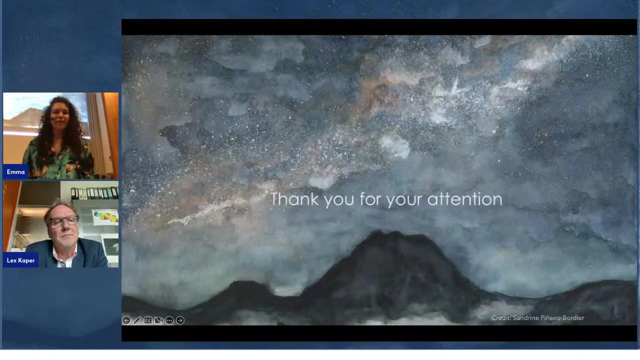 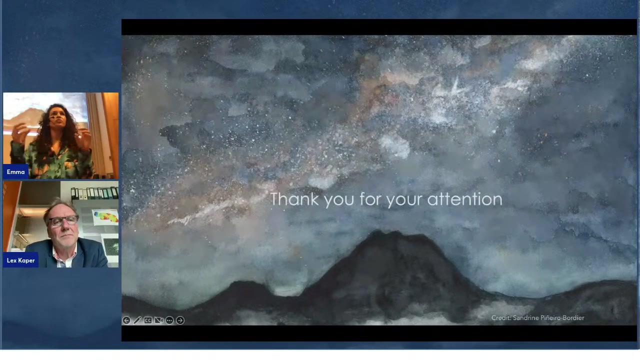 how all the material can actually be accreted and form such massive stars, especially because I showed that formation timescale is very short. You need really, really, really good mechanisms of accretion to build between two stars massive stars that then. merge and can create very high mass stars. And I'm trying to think about other processes, but I think on top of my mind. I would also suggest mergers to form massive accretions from the disk. You can build such massive stars. 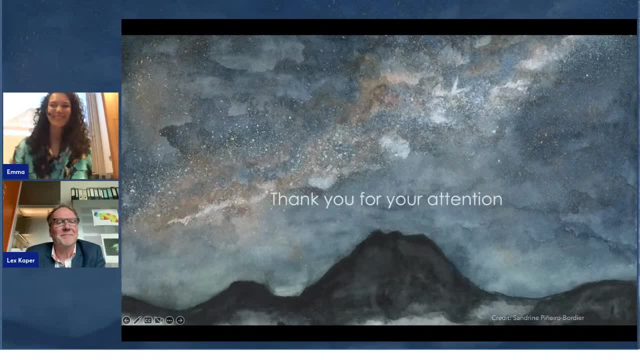 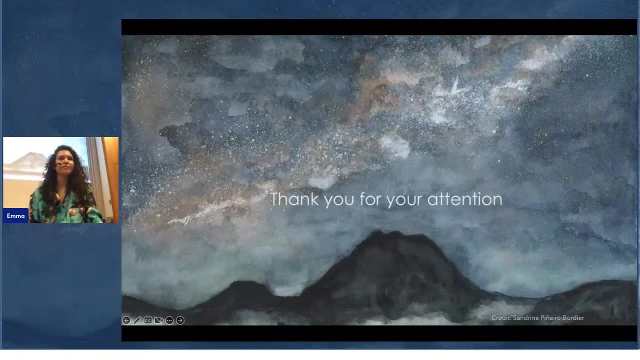 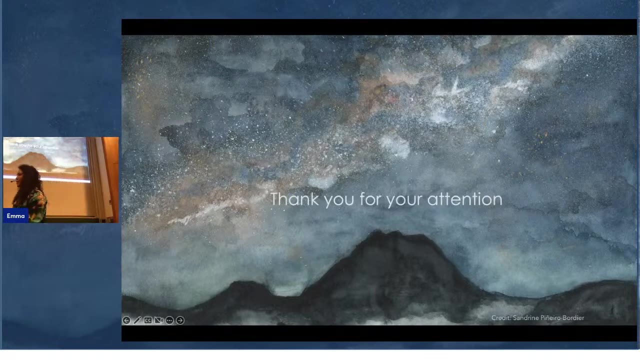 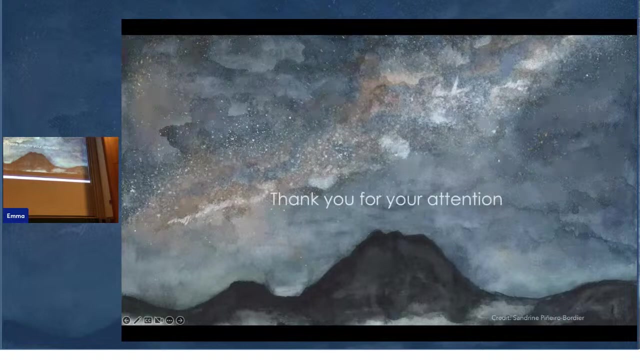 Yeah, Emma, thank you very much. Thank you, Lex. Thank you very much in the room, So that will be the first. I was from the University of London, Thank you. Thank you. My name is Helga. I'm from. 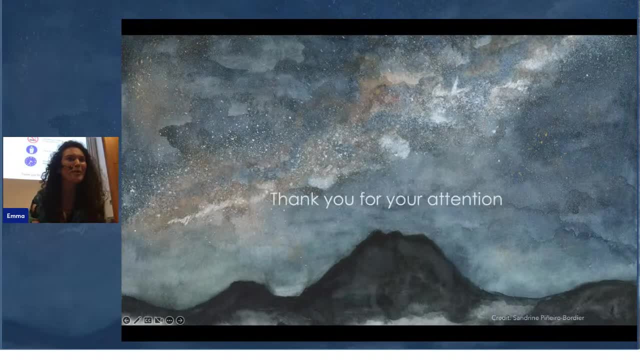 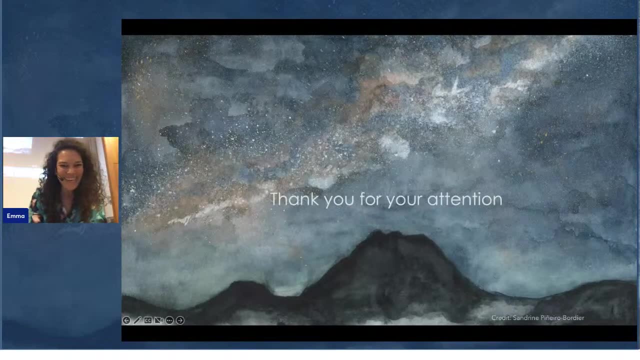 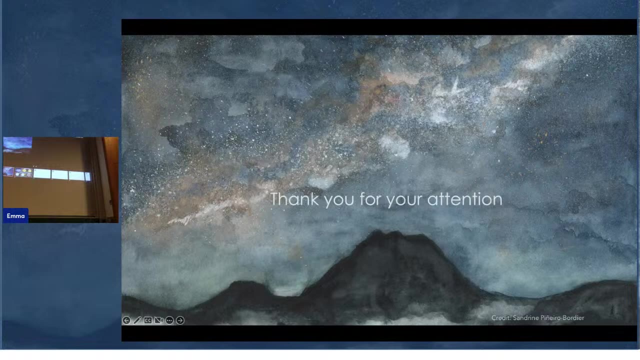 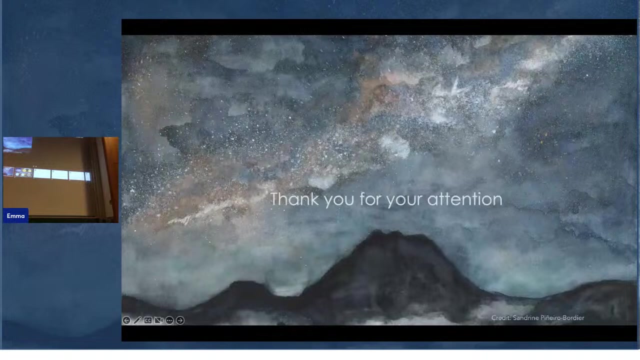 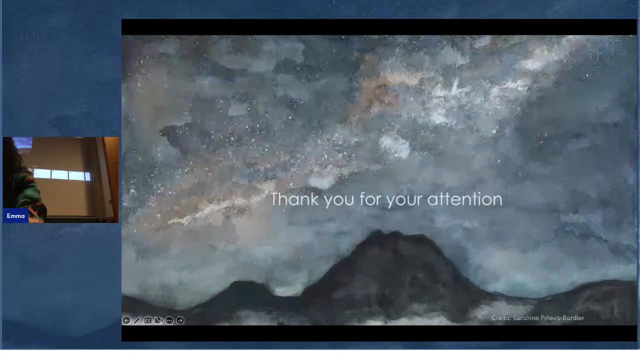 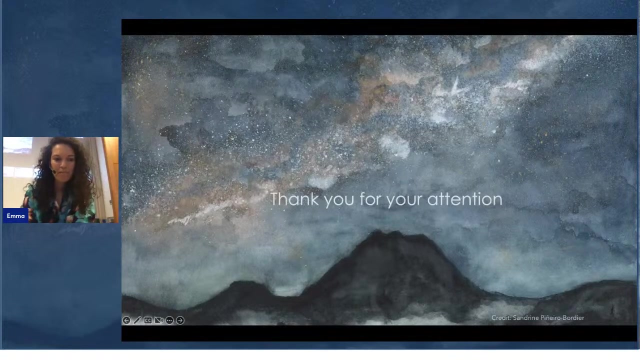 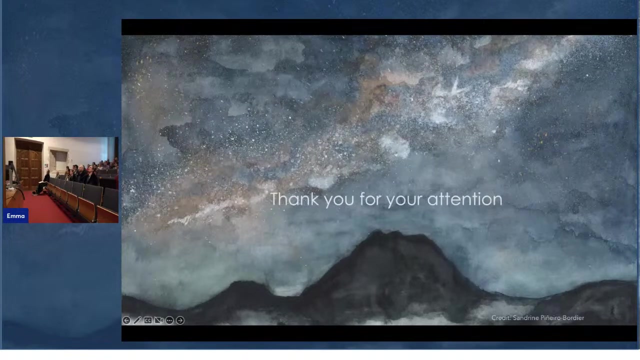 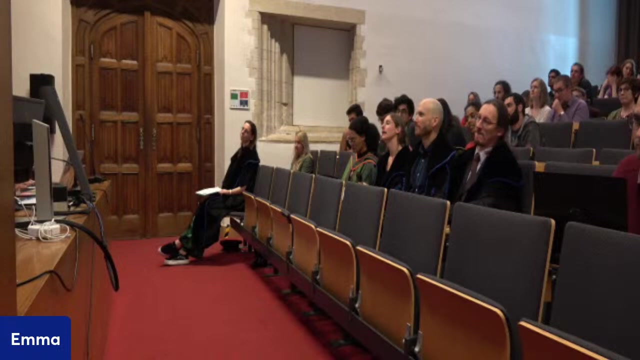 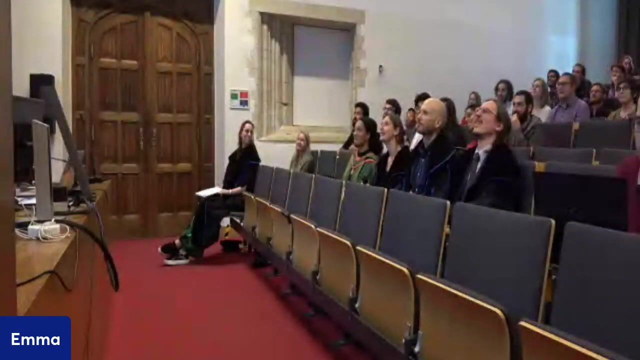 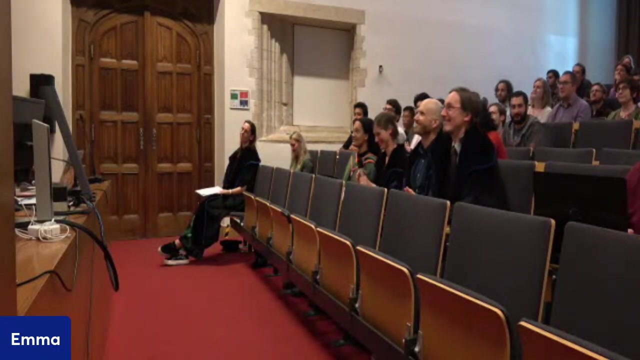 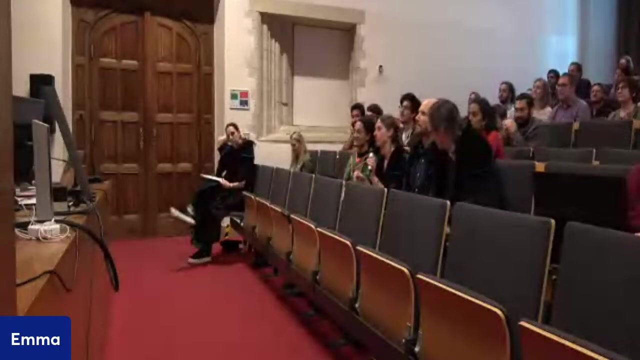 the University of London. I am going to a workshop in the University of London in London And I'm Okay. first of all, I would like to thank you for the presentation today and thank you to all the students. Also, I would like to mention that this is a really nice program: very precise, very clear. 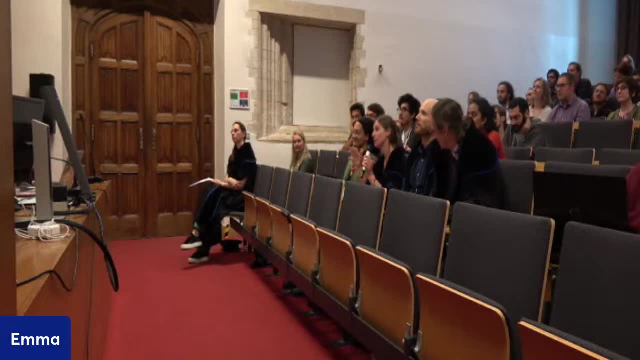 And that's a journey at different scales, with different social methods, and even trying to connect and maybe, let's say, bridge the gaps, the gaps, the gaps between services and learning, as you can imagine. And so my question may be that you have the antidote, Joan, and that you think about a lot of all the future. 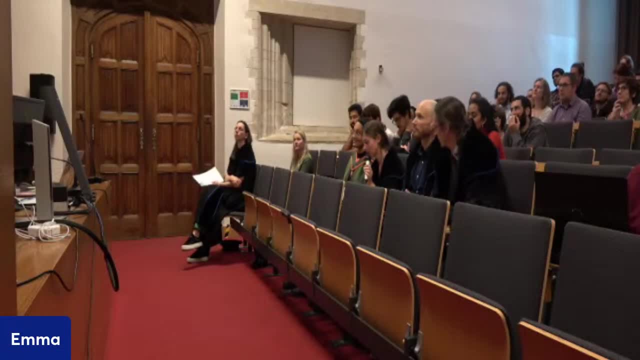 My first question would be: which observational data do you believe that the astronomers will get quite soon? that could be very useful for online activities. Very good question. Yeah, I don't know. I'm focusing myself on interferometry, but I think that this is not the easiest and the quickest. 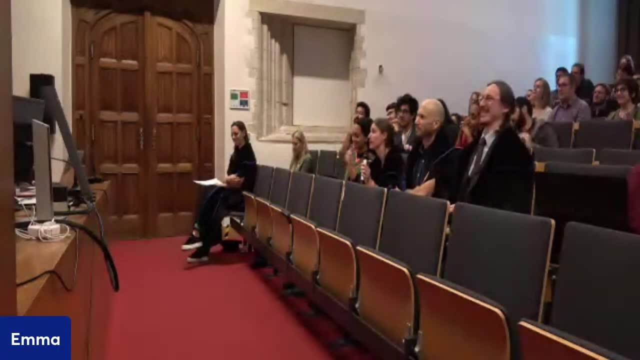 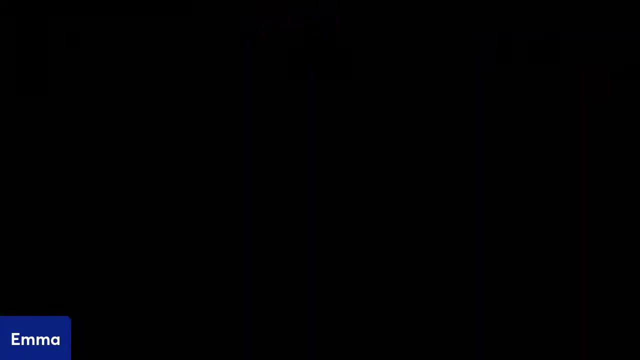 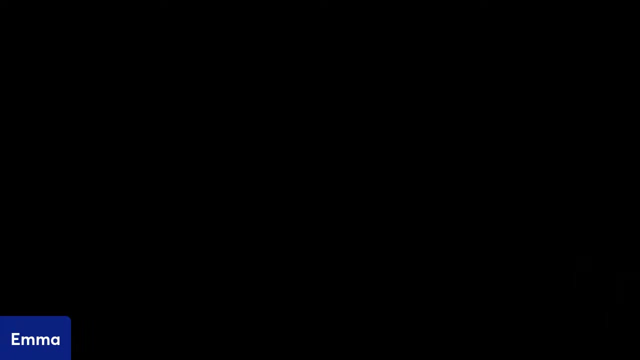 So Okay, so you talk about just triple systems, right, Okay, Yeah, Well, I think that all the work that has been doing in getting like actually observational constraints on these triple systems that were like basically taking one data point every year, 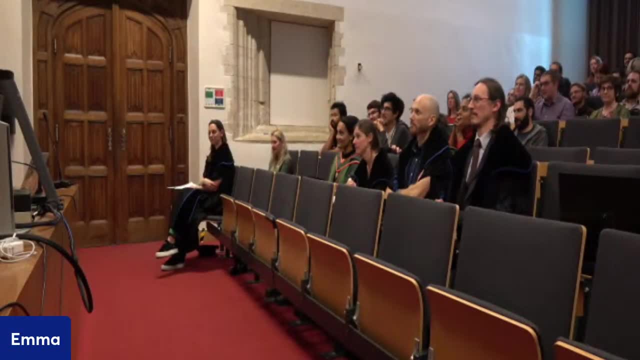 is already like a very good start to study these triple systems. The thing that I think is almost the same as I told to Lex, is also like trying to combine the different techniques So we have like a full picture of all these systems. 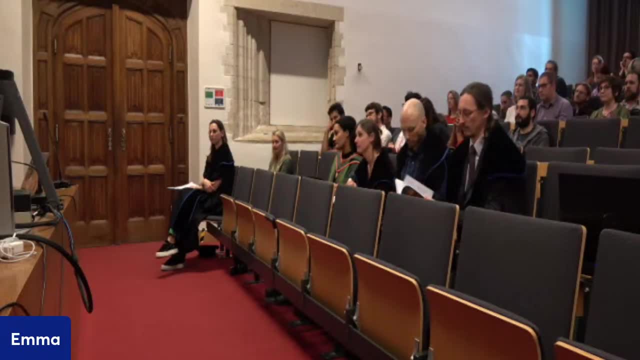 because we look at the triple system but we still don't know, like, if there are, like, maybe, other components that can be bound around. So this could be done through direct imaging, AOS-assisted imaging as well, such as Sphere maybe. 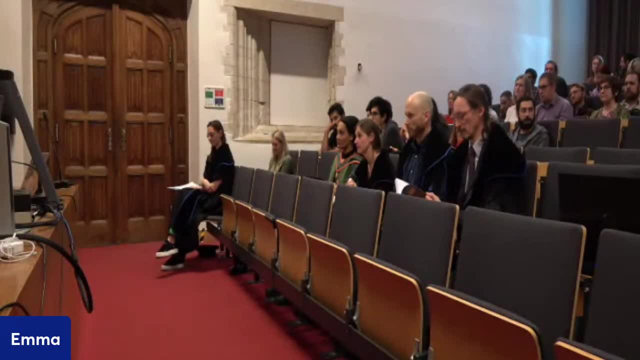 and also to look at the closest separation ranges. that has been done with spectroscopy, I think, But Yeah, we also don't have like fully solutions for all these spectroscopy binaries, and this is also something that we should do. 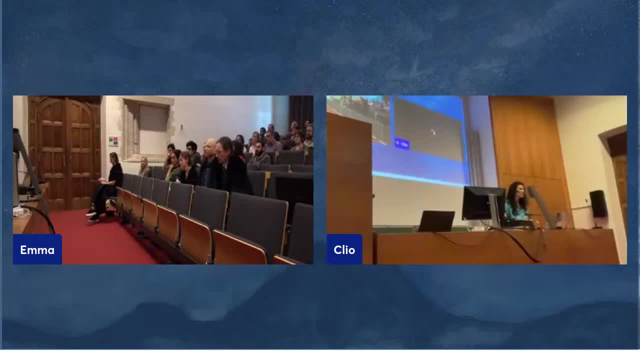 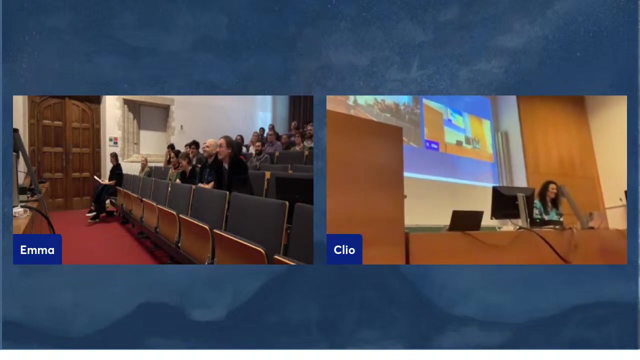 because if we want to study these triple systems in a very accurate way, we need both solutions for the outer component and the inner component, And I think that spectroscopy, in that sense and prospect, is faster to get data from than micrometry. 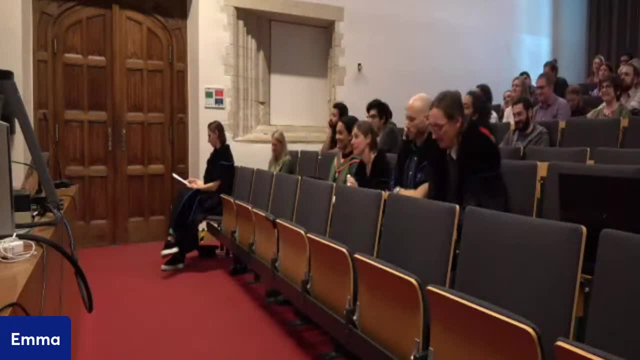 On top of my- I haven't studied like I know- there are a lot of triple systems or multiple systems that are all together in the spectroscopy sensitivities and that we can also explore them just with spectroscopy, for example. yeah, 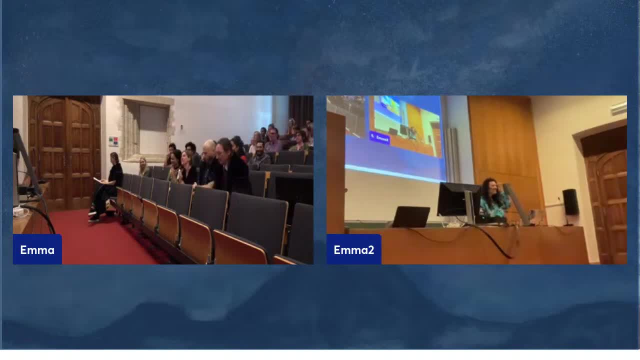 That's what I did. I can imagine, And if we take a question in the other way around, if we imagine now what could be the use of dynamic study, that could be useful for you maybe to give some precision about the different information methods. 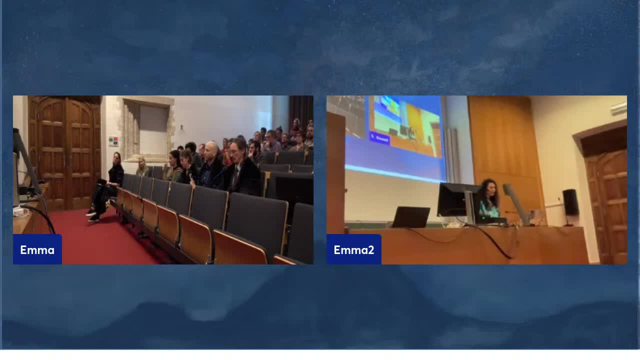 Yeah, that's a really good question. No, I haven't really estimated this. 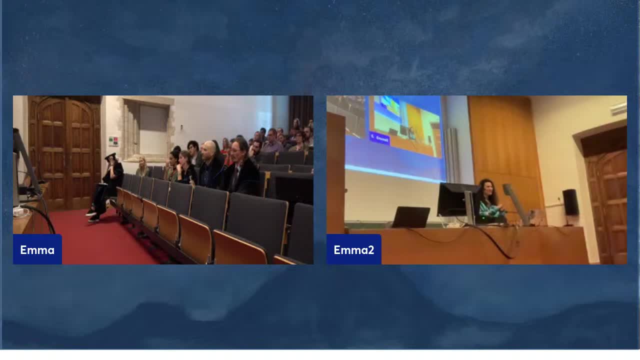 Yeah, I perfectly know what you're talking about, because we know that with NECO and the observation, for example, for planet services, people also, in which we can we collect for this really accurately, then we can spot, uh, maybe planets, um, uh, no, actually we don't. 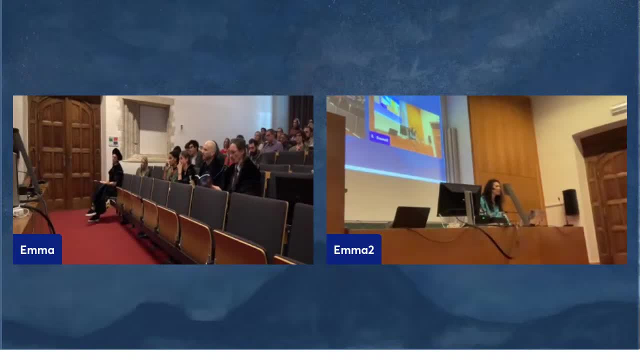 find any close by, but i also haven't fully done the correction on these people. so, yeah, i cannot answer you of this, but it's definitely something that we should look into here. thank you, thank you. uh, then i would like to ask the supervisor and co-supervisor also. 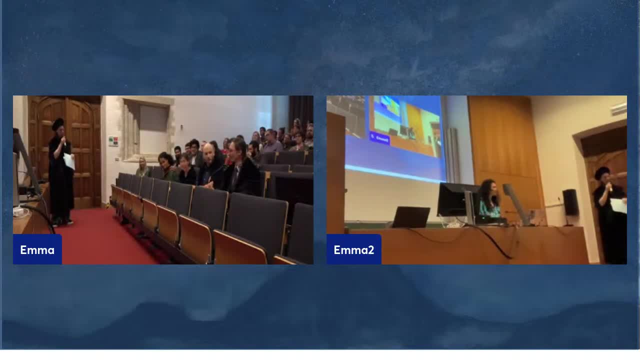 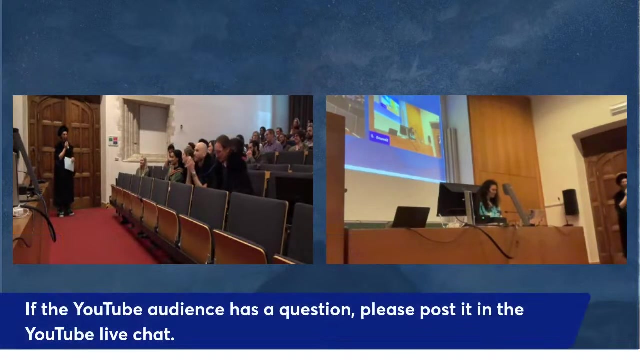 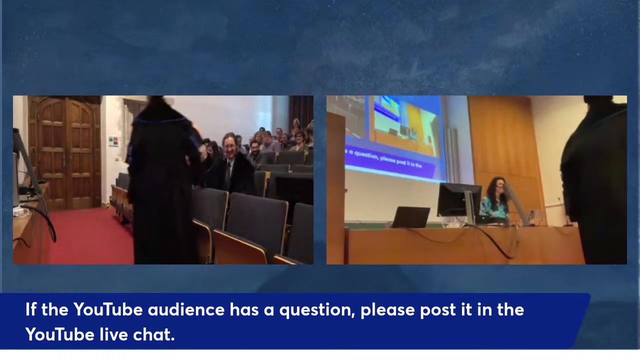 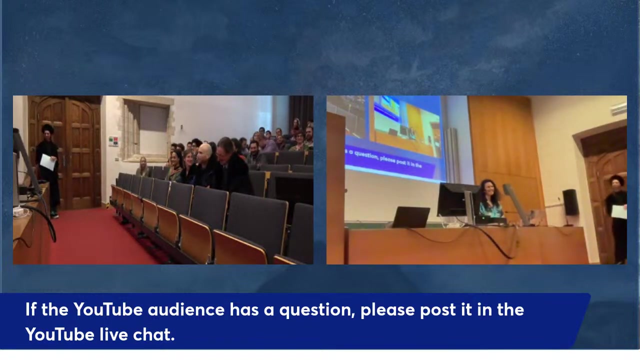 do you have any questions? yeah, so this is of course, a public fence. you are also invited any question. you should be introduced. thank you very much, emma, for this pretty awesome presentation. uh, i think you know very well. i'm really interested in your work and i'm really hope one day learn from you how to form venus stars. 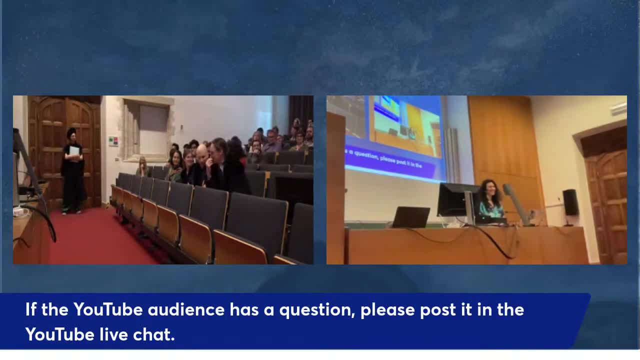 and, in that regard, um, can you speculate on whether maybe anything special needs to happen in order there's something extra needs to happen to go from one month to one day, or is it just an extreme? Well, this, I think it falls a bit more into binary evolution, which is what you do. Maybe I still think that the influence of other companions is something that can definitely help watching down to these separations. Yet, yeah, I don't think about any other specific mechanism that could help running these peanut stars. But yeah, Okay, Yeah. 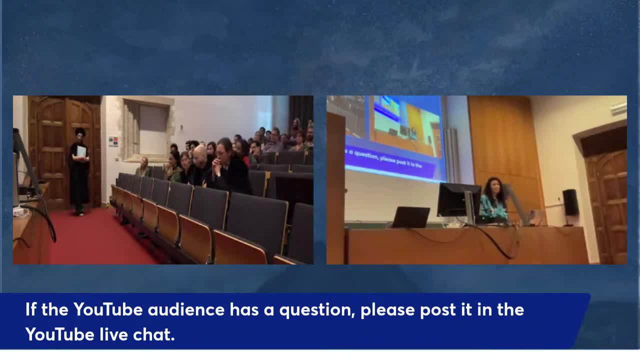 Maybe colleagues like oh yeah, but it's really hard also to tell, like, if you have a model that maybe can interact with another multiple system, and all of a sudden, like you have very Yeah. I actually don't know much more about this period of stellar collisions. I would say But On the other hand, you would say it's very hard to form a peanut star in situ without In situ. I would say yes because I don't see why they wouldn't merge instead of staying in this steady stage of keeping. 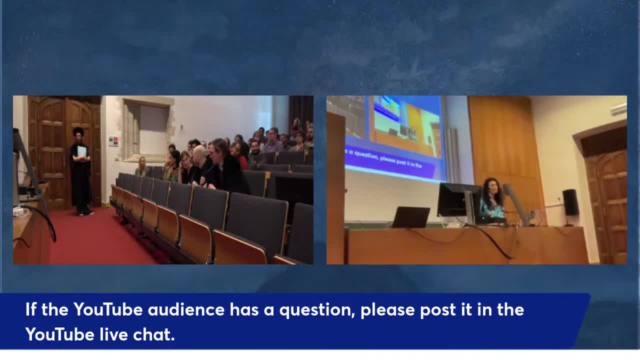 Yeah, Yeah, Such small separations- Good, Thank you. Thank you very much, And also the presentation was super nice and quite easy to understand for people who are not familiar with the topic. I have a question. You clearly showed the impact of interferon. 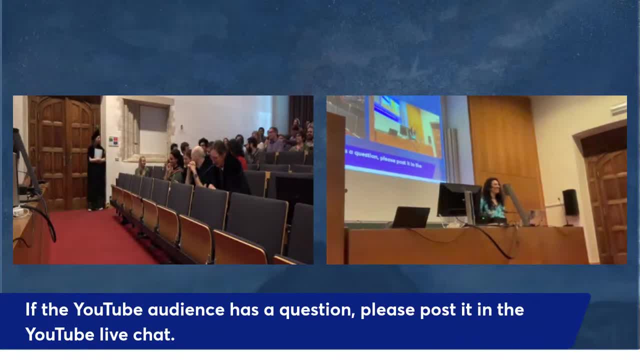 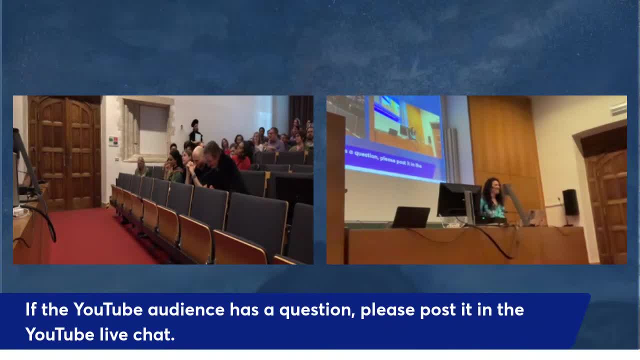 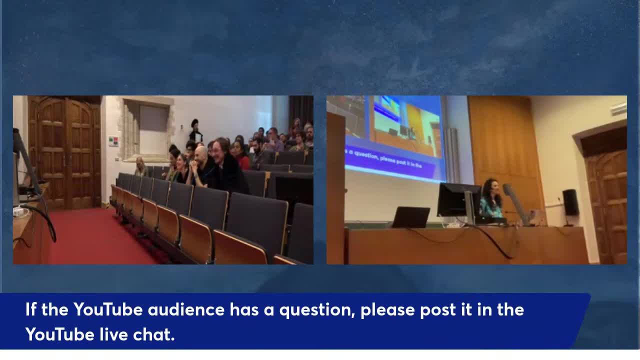 Yeah, Yeah, Yeah, Yeah. would it bring to the city in your study? Okay, yeah, of course. So we have already built a much bigger interferometer, for example for the observation of our supermassive black hole at the center of our galaxy. 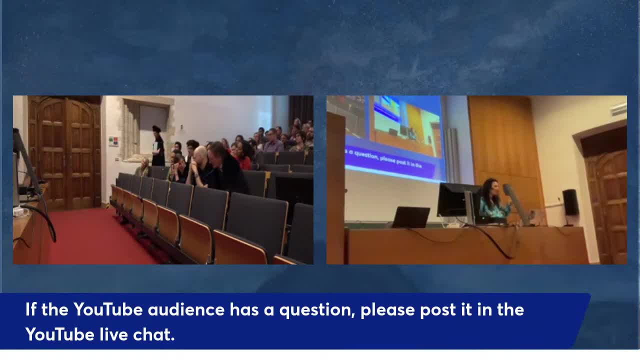 So they recreated basically a telescope of the size of Earth. Now we are really up to date with the topic because it actually was proposed by NASA, like two or three months ago, to have an interferometer on the Moon And this, I think, you get rid of all the atmospheric effects. 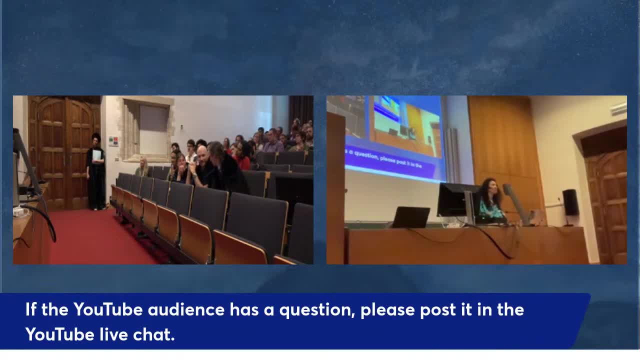 So this is like really good for images. Then you have to think about which wavelengths you're thinking of, Because, for example, for the central, the massive black hole in our galaxy- sorry, it was done like in the submillimetric. and then you lose also resolution. You build like a bigger telescope but then you increase the wavelength, so you have this kind of balance. So if you would create maybe an optical or an infrared interferometer from the Moon, then it would be very good for us actually. 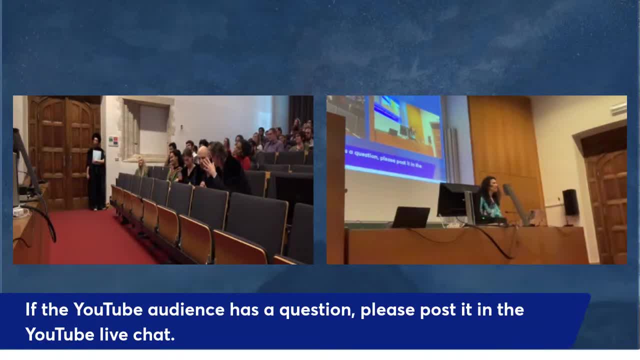 for the science we can do, because you would reach such sensitivities that would allow you to see the very close environments of the stars and maybe also reproduce images, which is something that we are working on at the moment. So we know very well. 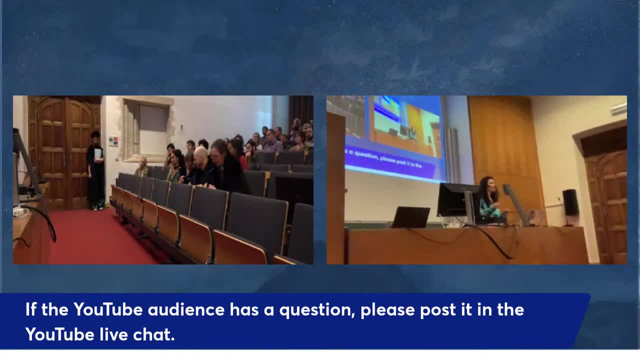 that if we are very close at the stars, we rely mainly on spectroscopy, like for simulations at least, and we don't have a great amount of images such as in the front. so that would be also very good, But still not doable. 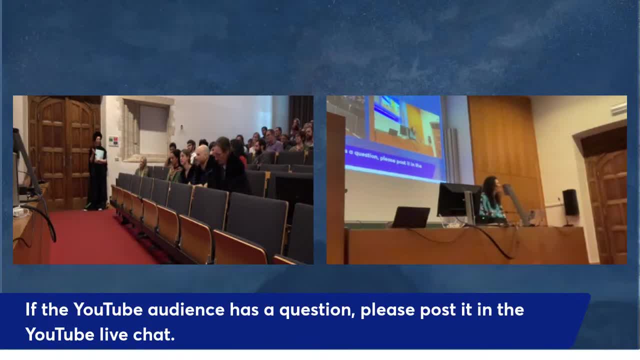 with the actual technical. Yeah, The last question. one or two turns, I guess. Are there any questions online? I don't see them. So those chances must come. Okay, And it must be going to the demonstration, Thank you. 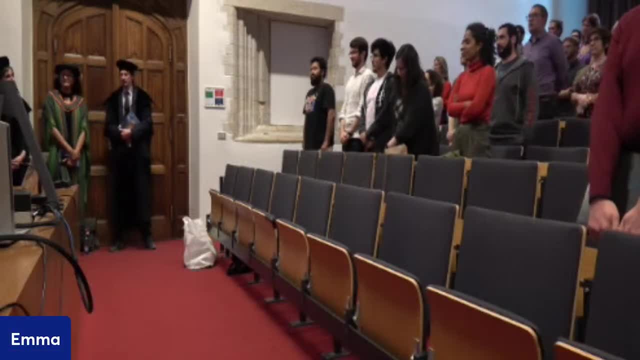 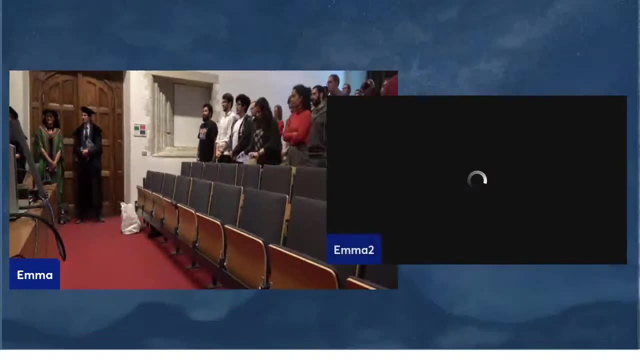 degree in science, astronomy and astrophysics. emma portier has presented to the faculty her phd thesis on the top degree in science, astronomy and astrophysics. emma portier has presented to the faculty her phd thesis on the top on the origin of lessons for spirals: impartial fulfillment of the. 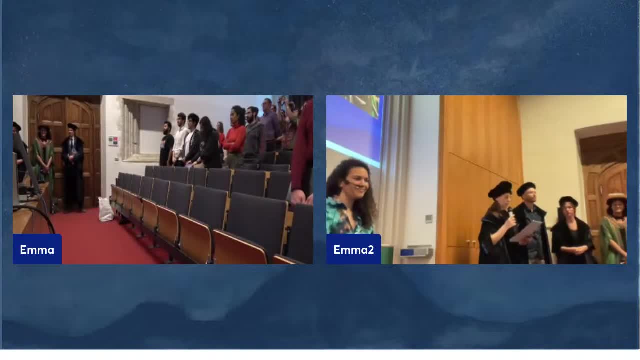 requirements for the phd in science, astronomy and astrophysics, and emma portier has defended the thesis in a public session before the examination committee. the examination committee has determined that all requirements concerning the branding of the doctoral degree that are prescribed by the law and university regulations have been met. 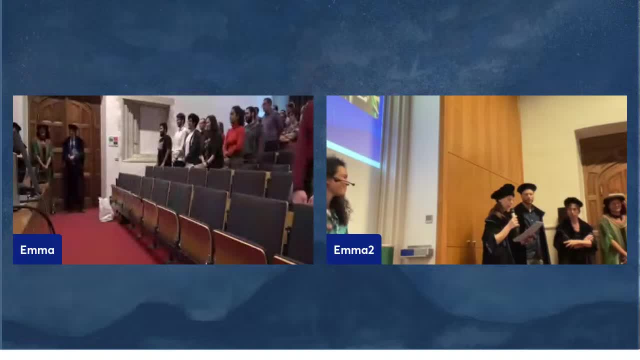 therefore, on behalf of the director of kyle levin, i am conferred upon emma portier the degree of doctor in science and story astrophysics. by obtaining a doctoral degree, you commit yourself as a doctor also in the future, in accordance with the basic principle of research and 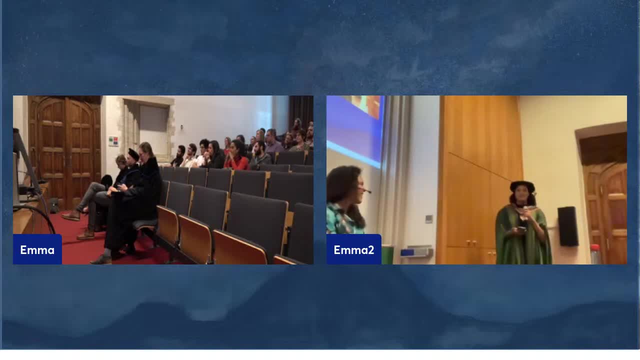 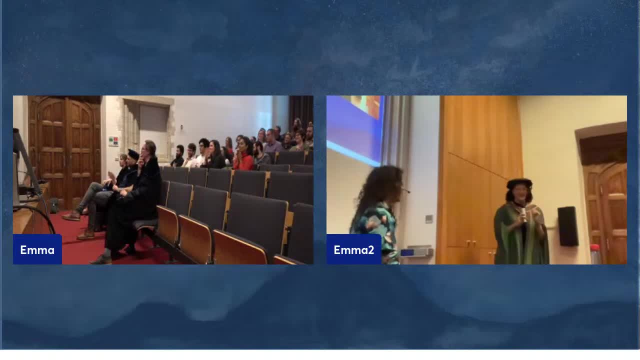 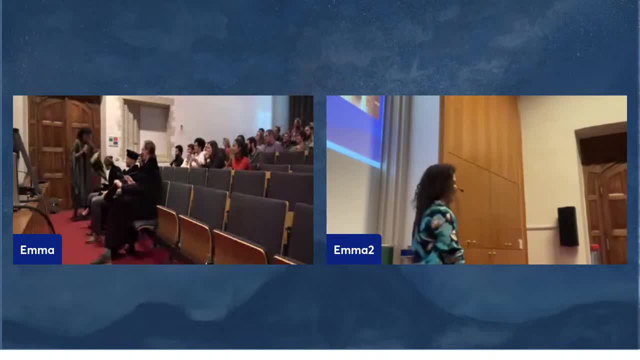 Thank you, Thanks, Thank you, Thank you. Oh, Okay, Great Thanks, Can you hear me? Yeah, Yeah, Feel better. Can you feel better Have a band coming up? Thank you, Thank you. Okay, Can you hear me? 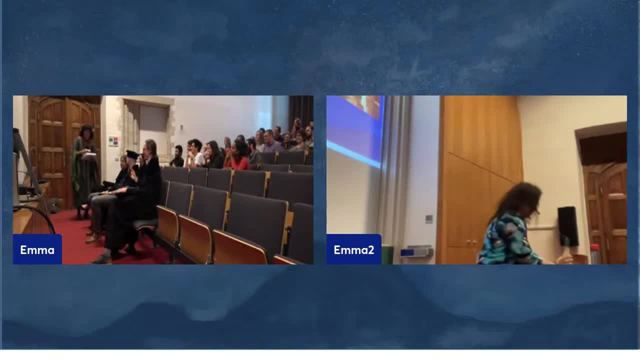 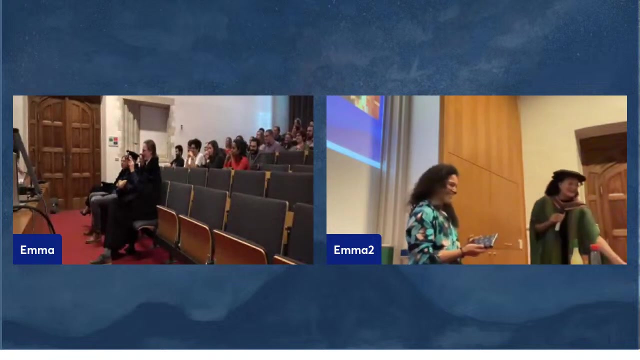 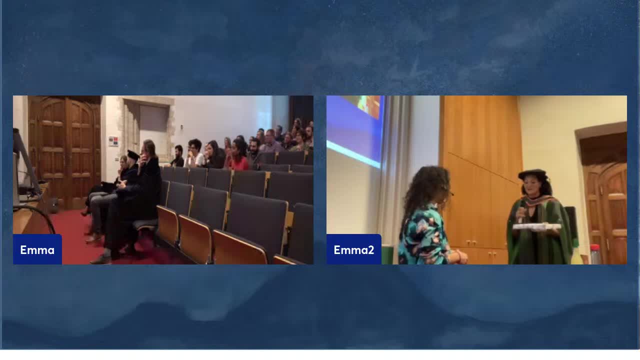 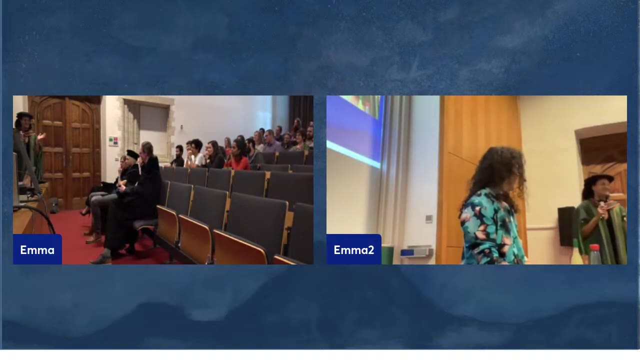 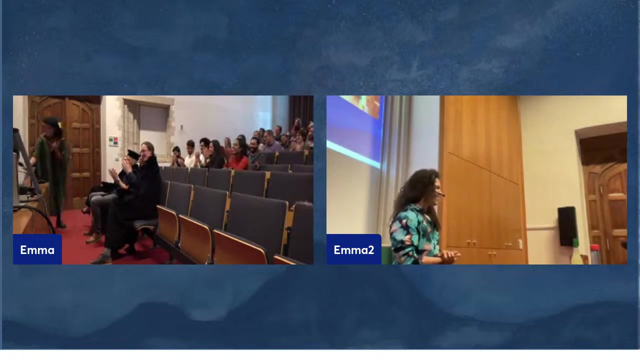 their careers at this point and I know they need our tradition to just kind of pull those good pastes into a little kind of thing. Thank you, thanks a lot. I don't know, I don't have a speech. I think that my reception is maybe easier to talk.